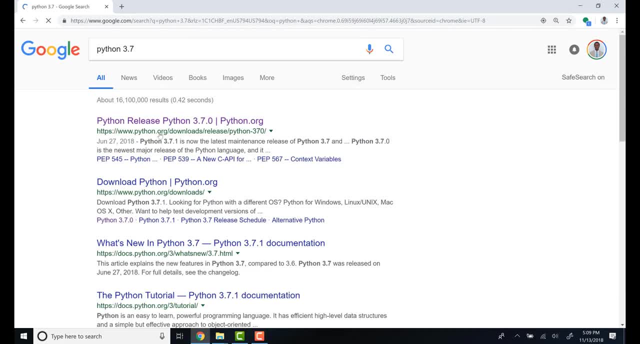 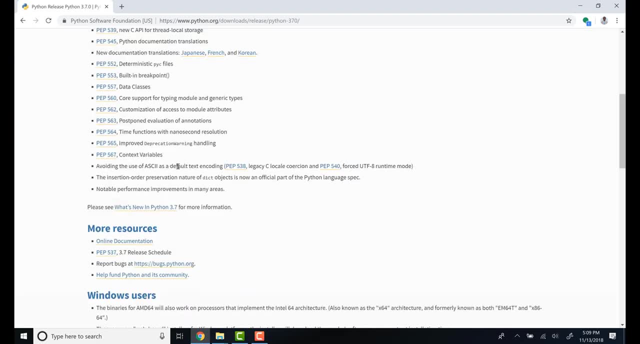 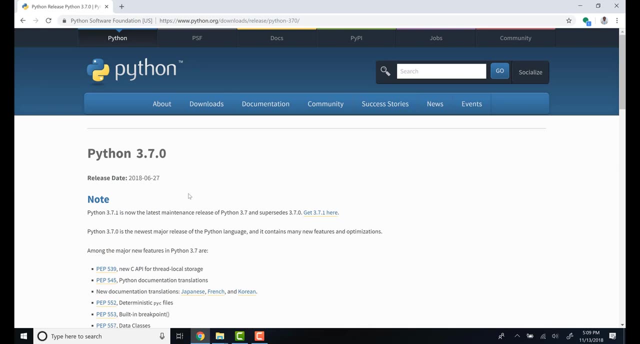 I think it's Python 3.7.. And let's go to the main Python website. Here's the main Python website. So that's the latest version, Python 3.7.. So this course will be based on, you know, Python 3,, specifically Python 3.7.. You can, you know, download the. you know the. 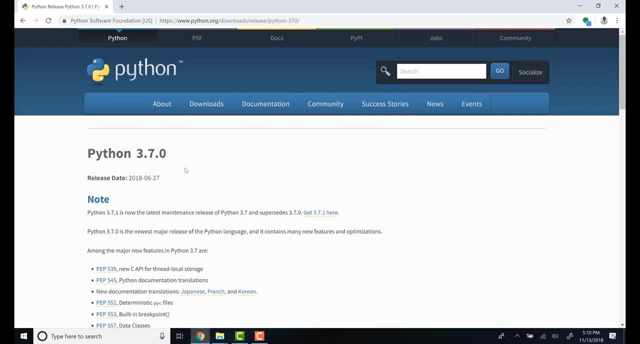 Python version and Jupyter Notebook. I think what I prefer is just to download the Anaconda, the Anaconda platform, and install it on your machine. And the beauty of you know Anaconda is it provides you, it installs automatically Python and it also provides you various, you know- data visualization. 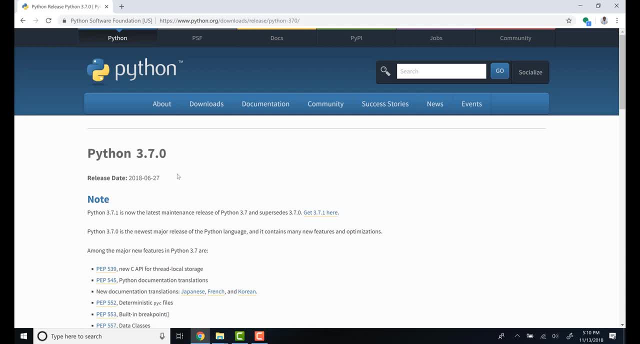 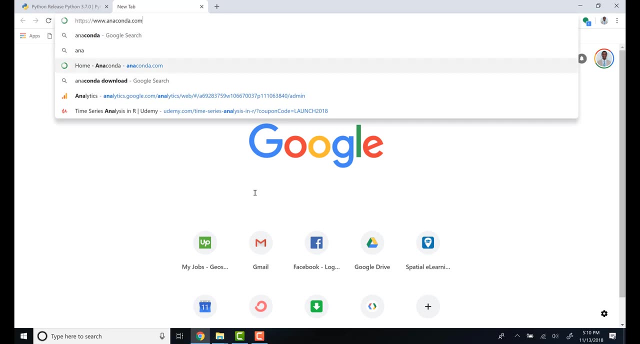 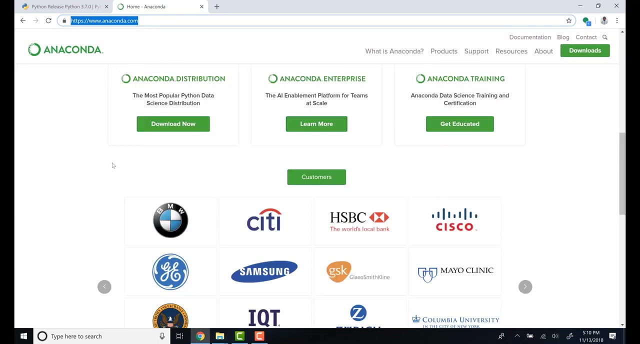 and analysis tools like the Jupyter Notebook and the Seaborn And what have you right? So let's go to the Anaconda website. Let's just add in another site, Anaconda. I think it's here Anacondacom. So here, Anacondacom, I'm in the main website. 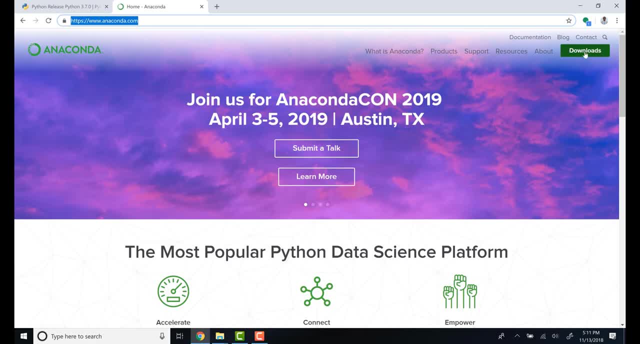 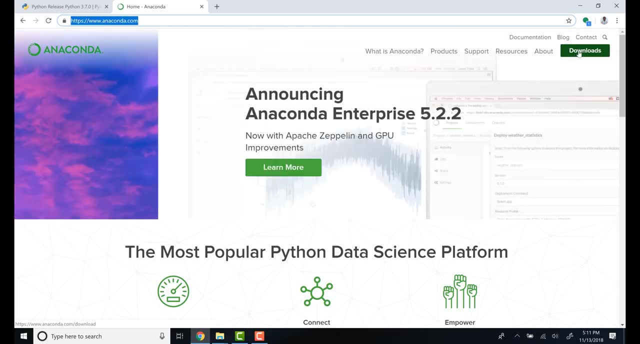 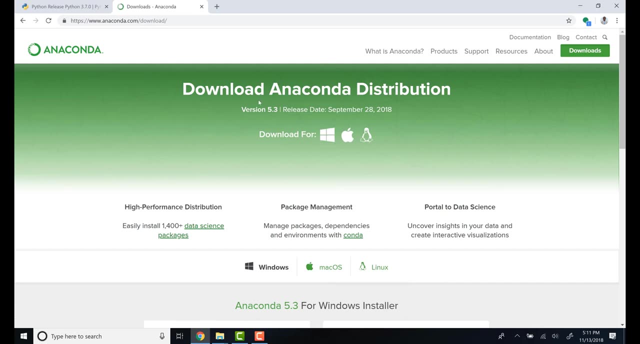 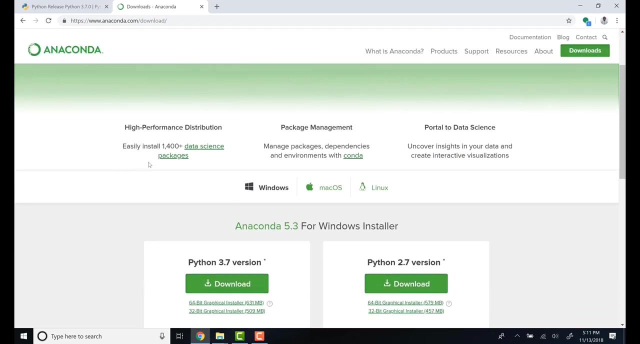 here. So what you do is just you find the downloads you know button on the top right corner here And click downloads and it will take me to the download page, So downloading the Anaconda you know package platform, rather. So what is the latest version of the Anaconda that? 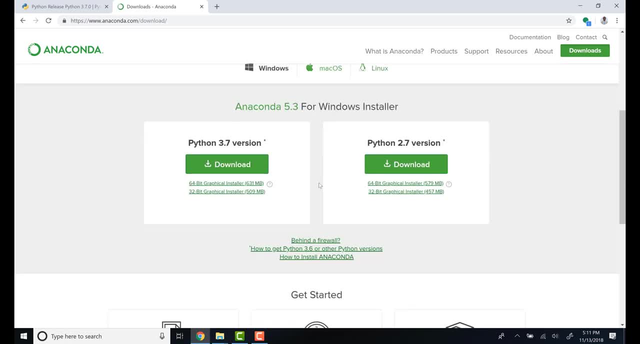 we have. So it's Anaconda 5.3,, you know, for Windows installer. So if you have a Mac, you can check this version- Anaconda 5.3 for Mac installers- And if you have a Linux installer, you will be able to see that version. But if you have, 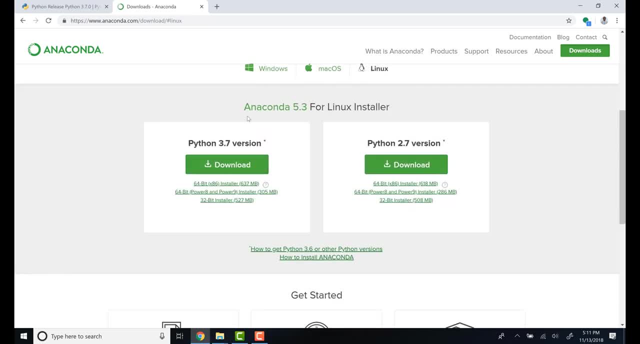 a Mac installer and you want to use an Android application, well, you know, you may go ahead and click download and it will take you to the download page. So at downloading the Anaconda machine, you can, um, you know, check this anaconda 5.3 for linux. so, um, so anaconda comes, you know. 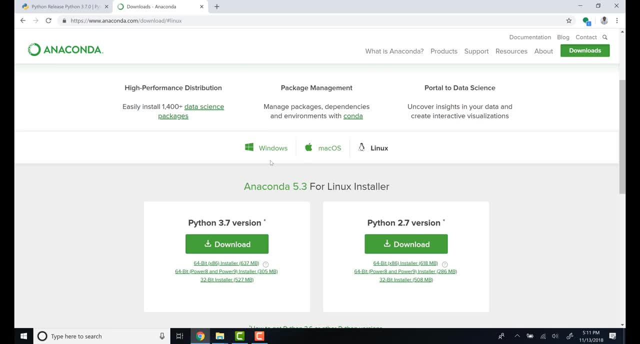 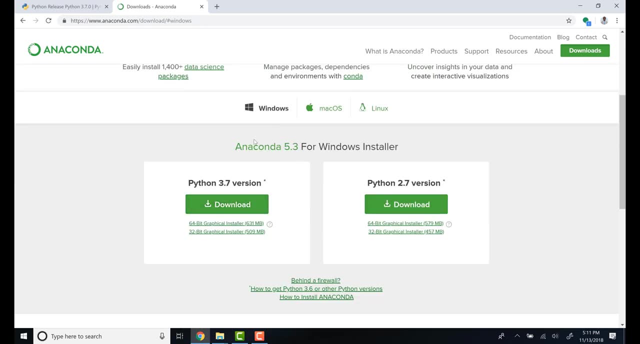 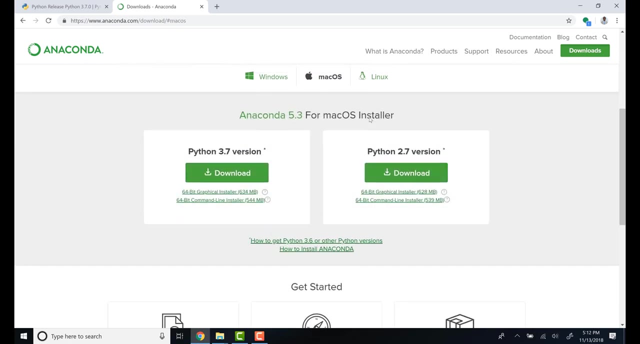 for all of this. you know the three um operating systems for windows, mac and linux. um, you know, in my case i have a windows machine, so i'll just go ahead and download the windows version. but if you have like, if you're working on a mac operating system or linux, you can. um, you know. 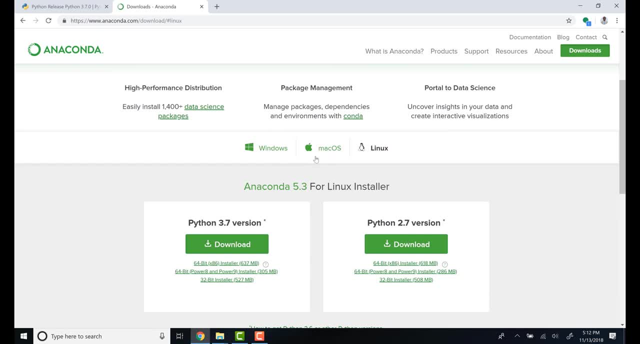 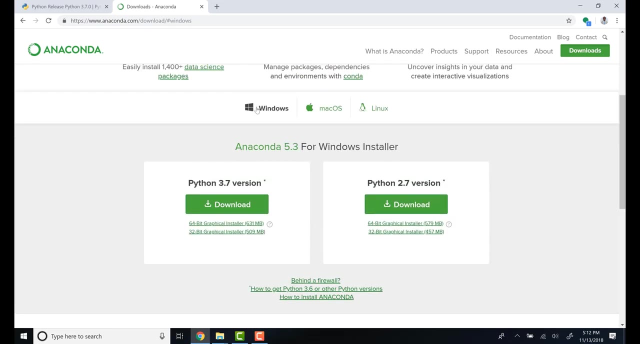 do so. right, just choose the you know your own um version, if it's windows, mac or linux. okay, so for now, uh, since i have windows um operating system, i'll just click the windows version um. it's, um, you know, dark black. that's what i selected, and also it shows you here. uh, you know, for windows, 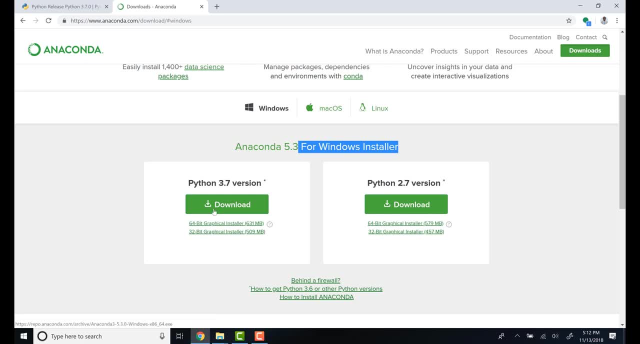 version. so this is the latest anaconda, and the other uh thing that you have to know is you. it will provide you two options of python uh: python 2.7 version and python 3.7. so this course is based on the latest python um, python 3, specifically python 3.7. so i'll just go ahead and download this latest version of python. 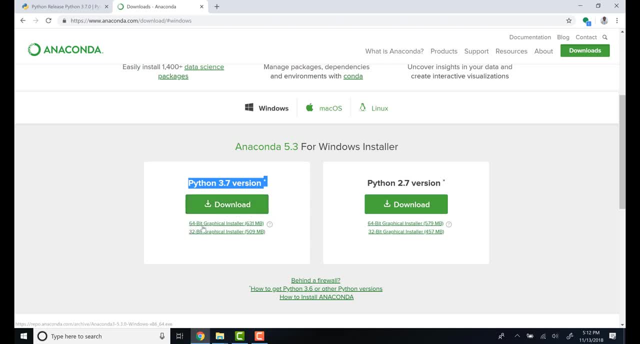 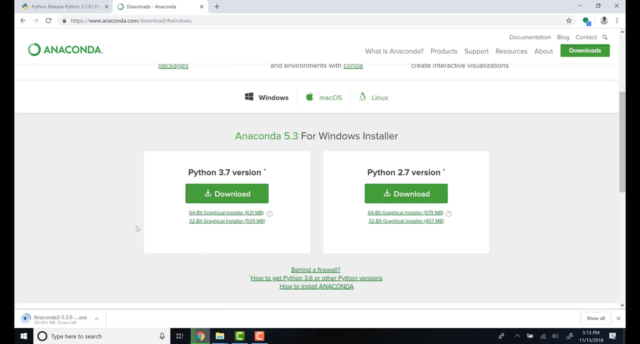 and you can also choose here if your operating system has a 64-bit or 34-bit. you can, you know, choose so. so in my case i have a 64-bit operating system, so i'll just click and download the 64-bit. you know python and um, the anaconda. uh, was the python 3.7 version. all right? 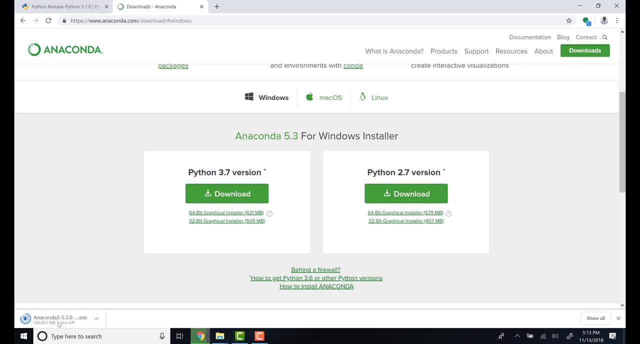 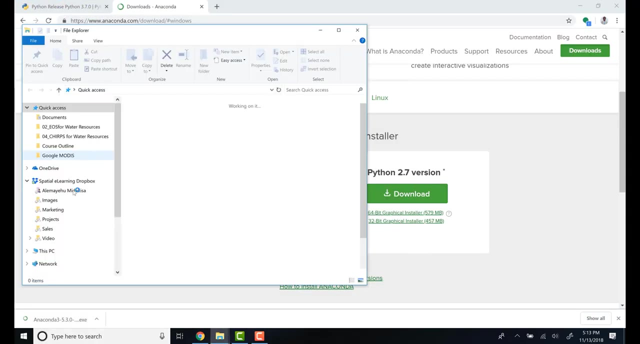 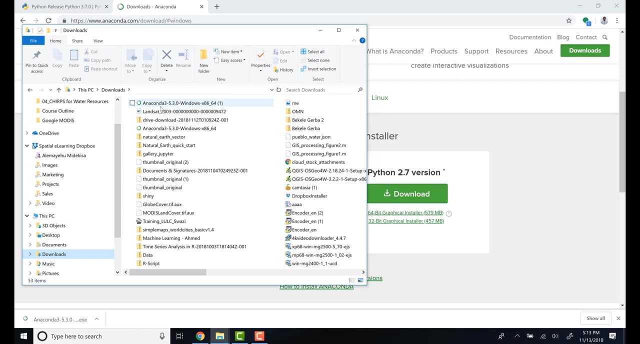 and, as you can see here, anaconda is downloading. once this blue circle is complete, my download is done. then i can go ahead and look at that in the uh download, the download option. let me go download lot, okay, here. so anaconda here is just, you know, downloaded here 64-bit 3.5. 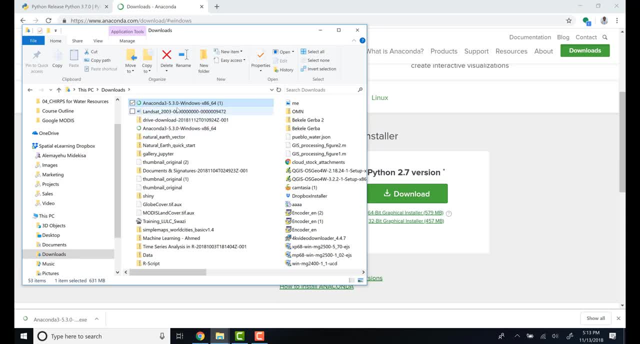 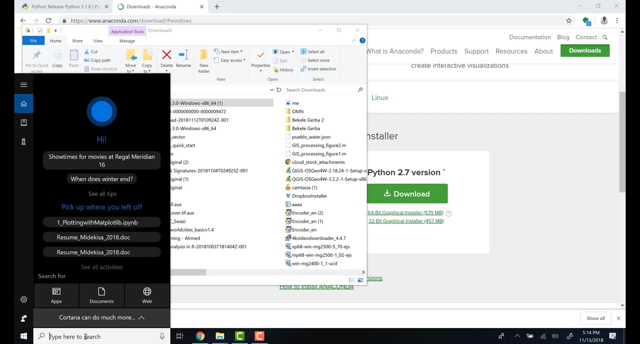 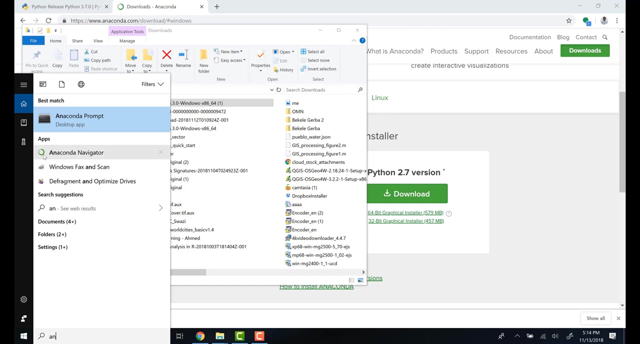 sorry, 5.3 version. so for you, you know, go ahead and double click this and it will automatically start installing anaconda in your machine, right? but because I already have installed anaconda, let's just go ahead and then start opening the anaconda navigator, right? so here's just a green, you know logo, or I can hear so. 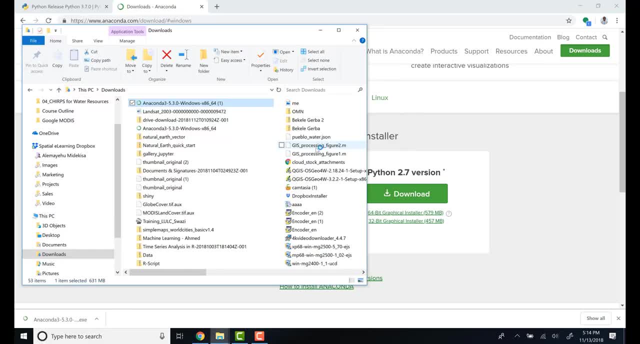 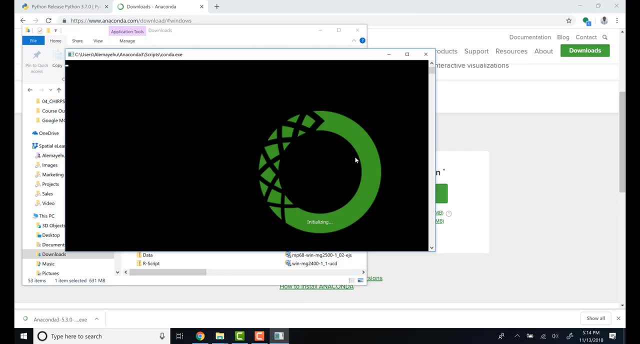 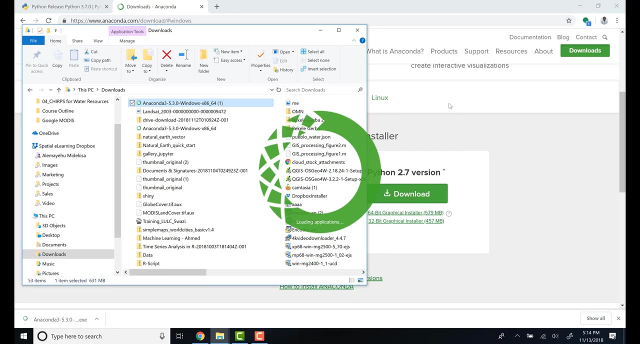 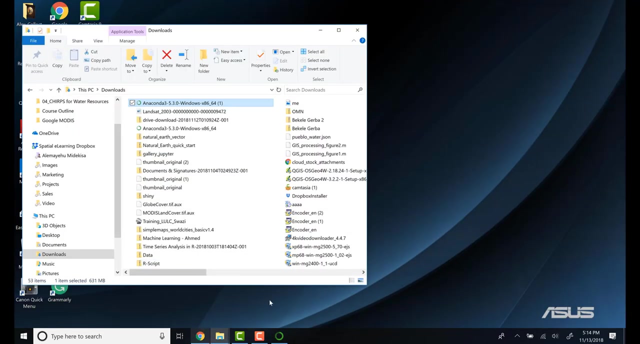 anaconda navigator. if I click that, the anaconda window, you know, pops up, right, it's just you have to wait a little bit. it takes time to configure and just load, okay, so so my anaconda, let me just minimize it this, okay. so this is the my anaconda, you know navigator, right? so, as you can see, 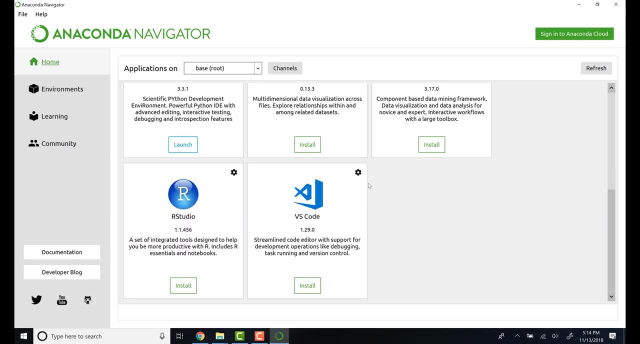 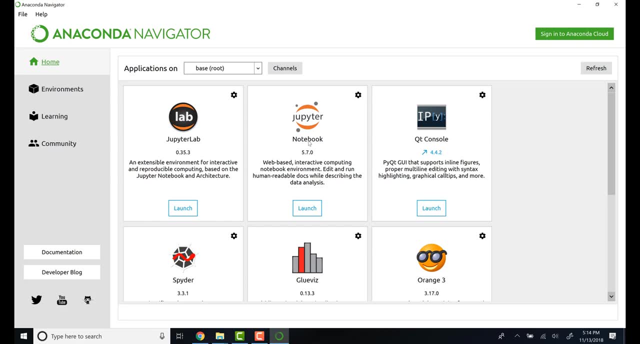 here, you know, the anaconda navigator has, you know, various tools, including, you know, the Jupyter lab and in Jupyter notebooks, this is the main platform where we will take, you know, this course. this is a Jupyter notebook where we'll do you know, Python coding interactively. 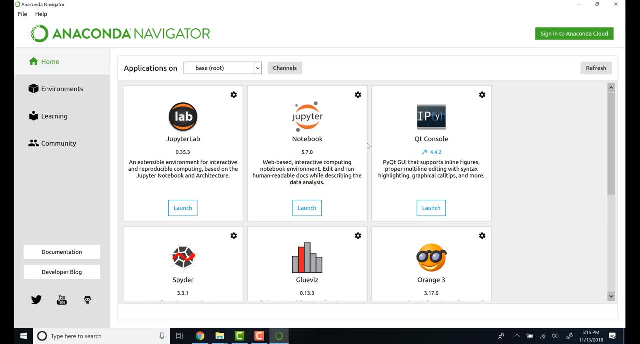 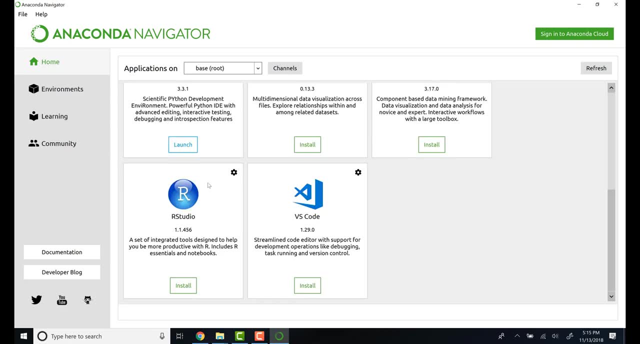 right, you know. so we'll use this one, but for now let's just go ahead and check the other. so the, you know, the I pi, and then the spider and gluvi's, or range three, and then our studio, which is a popular data science, you know, open source. 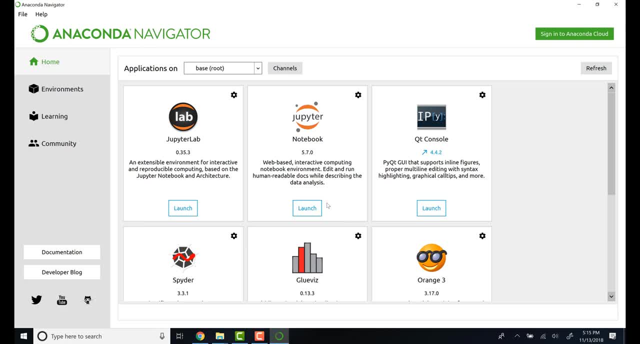 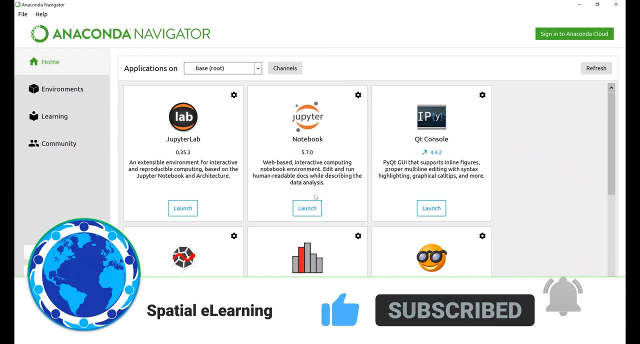 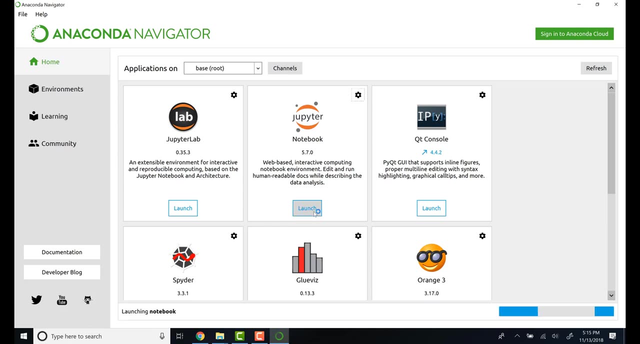 tool, VS code. so you have anaconda comes with. you know various applications, so in our case we're going to use vstio, use the Jupyter Notebook. So let's initiate a Jupyter Notebook like launch a Jupyter Notebook. This is one approach, how you can open a Jupyter Notebook right, And then I'll. 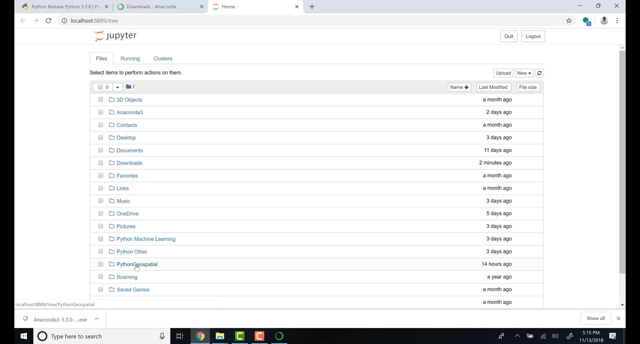 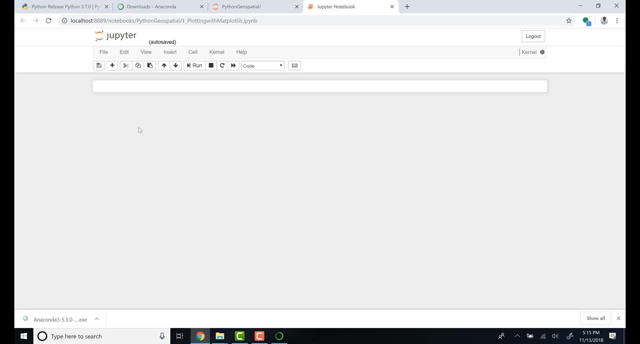 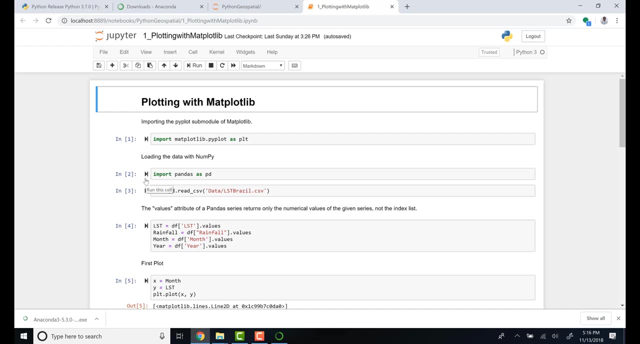 show you another way of initiating a Jupyter Notebook. So Python geospatial. this is my course directory and it will just take me directly to the code, right? So this is technically an interactive way of writing a Python script and just looking at your results and looking. 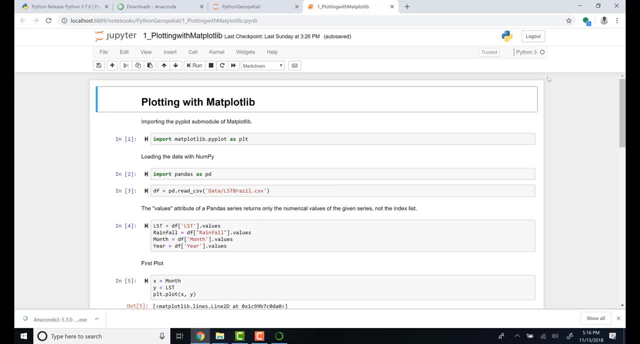 at your maps and plots, which is pretty cool, And then you can also see that this is a Python version here. As you can see, it's Python 3,, right? And then you can save your file. So this is just the code, like a Python Notebook, And 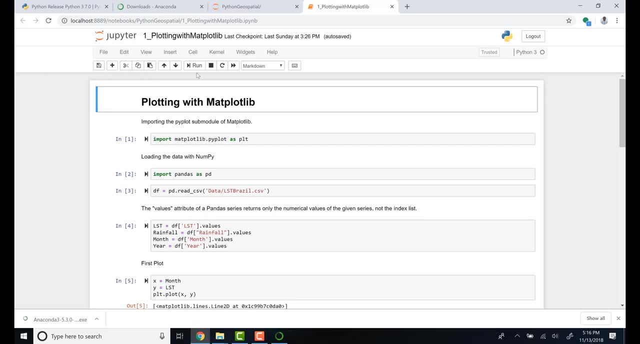 then you can add cells, here You can cut, here You can run. So it's pretty handy. And so let's just look at another way of installing a Jupyter Notebook like this same thing. right, Let me close this, Okay. 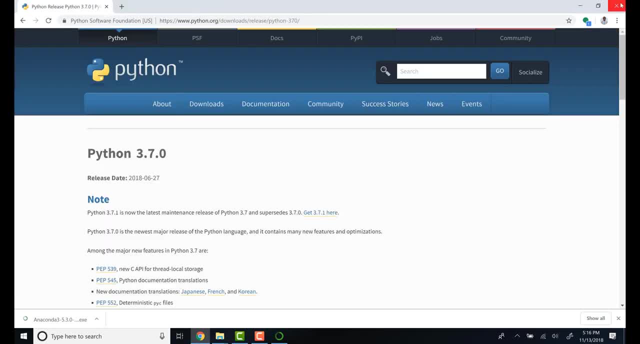 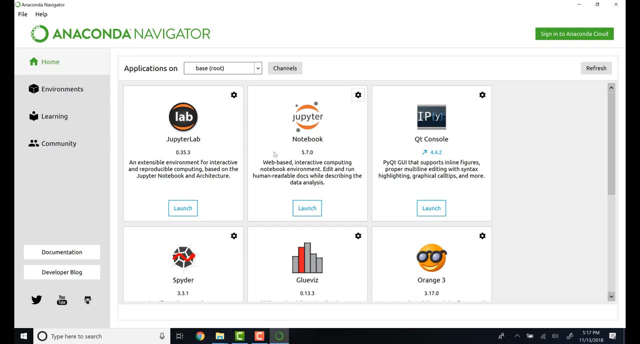 Okay, Okay, Let me close the Anaconda window, the Python window, And then let me close the Anaconda Navigator. So, without going manually to the Anaconda Navigator, you can open the Jupyter Notebook just programmatically by using a console. Yes, All right, So because I already 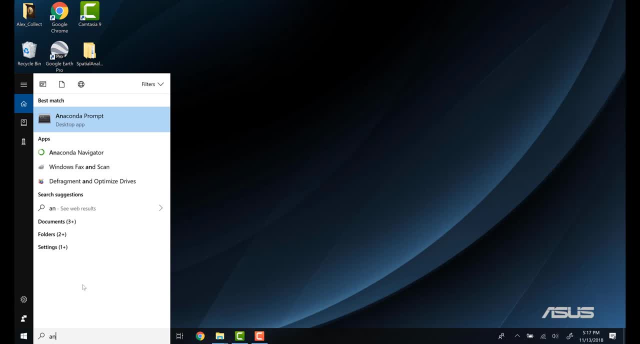 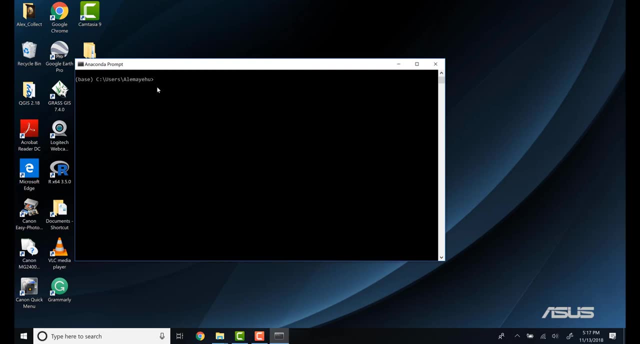 have Anaconda installed, then I can open the Anaconda prompt here You can see, here it's black. So just if I click that and this is an Anaconda prompt. So anytime you want, you know to write, install Anaconda, like package, like you know, NumPy or Pandas and what have you. 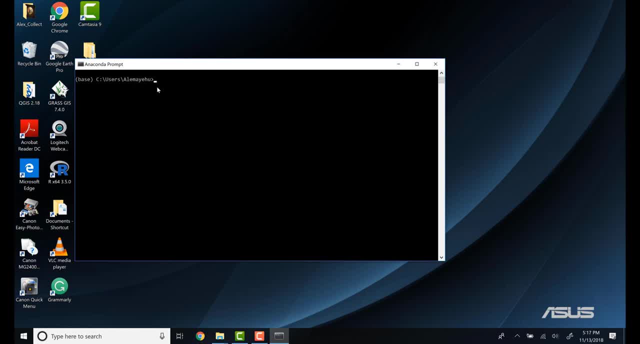 this is like how you can write you know a code, installation code, and just run it And then it will download. But even to open a Jupyter Notebook, I can do that here. So what I'll do is just write. 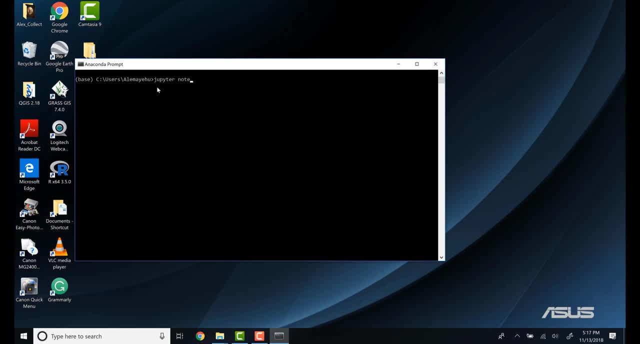 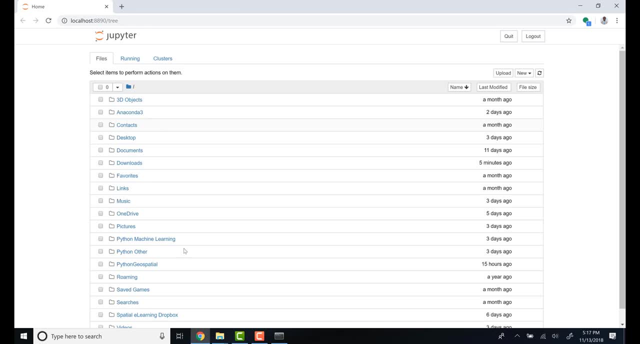 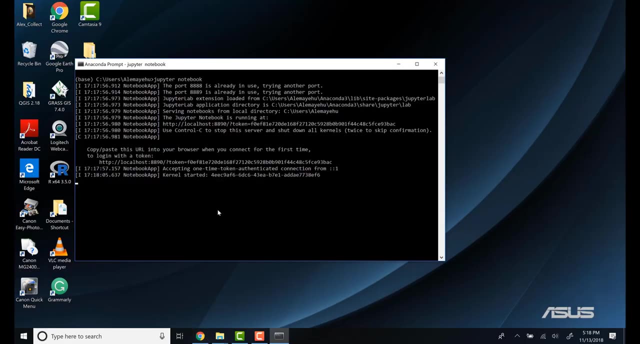 I'll write Jupyter Notebook And then, if I hit, it will automatically open a Jupyter Notebook, The same thing that I have done manually. right, So it's pretty cool. So every time you want to open, you know, a Jupyter Notebook, you can just you know. 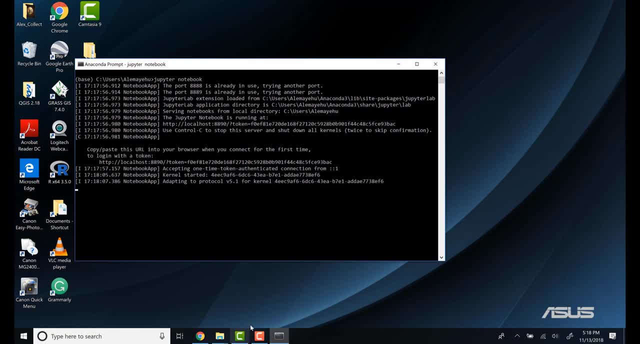 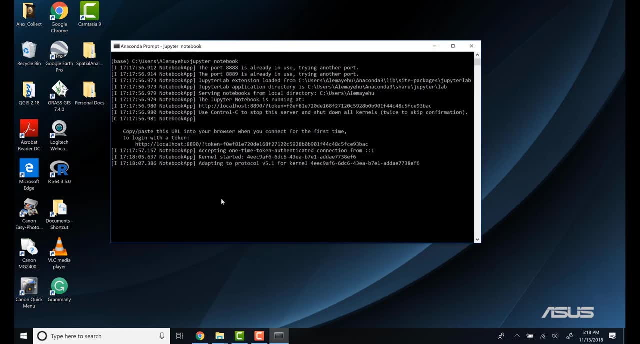 write it here programmatically. So that's all to what I have to. you know, show you how you can do. You can download Python with the Anaconda, you know navigator And then, once you have Anaconda navigator, you can initiate a Jupyter Notebook to start, you know, your coding exercise. 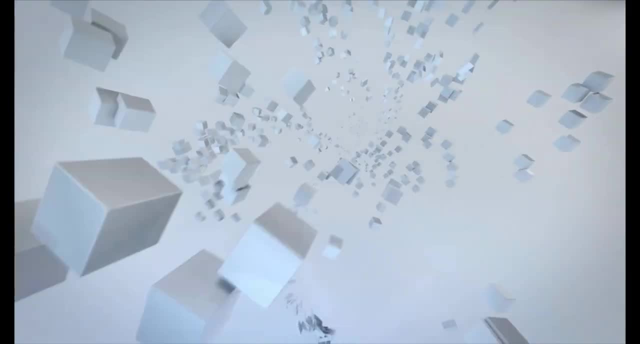 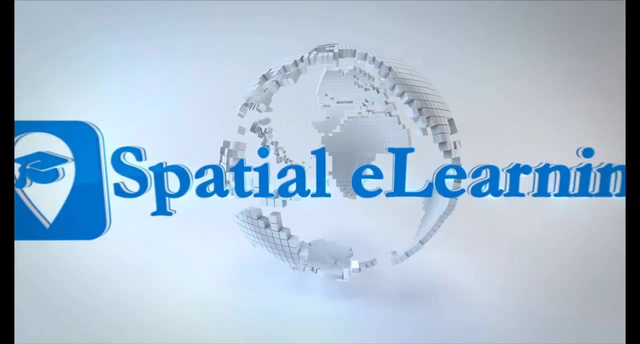 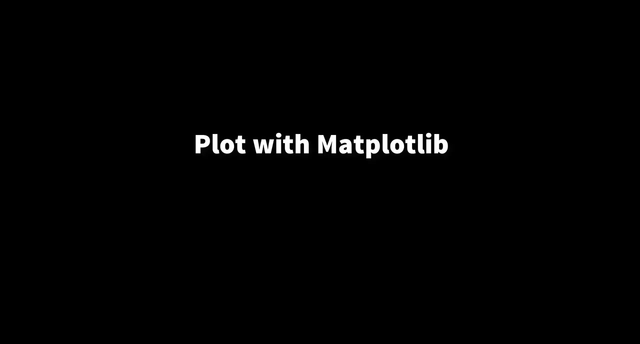 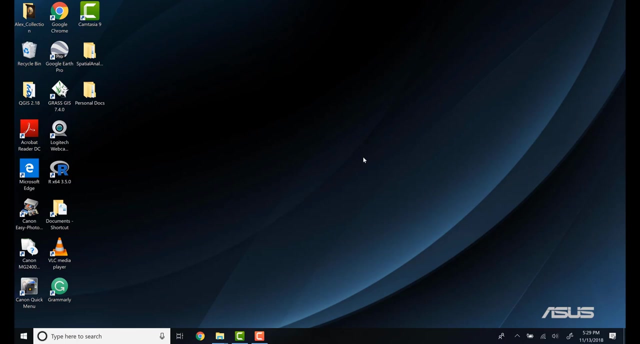 All right, And this lecture we'll be installing the Jupyter Notebook, initiating a Jupyter Notebook using a code prompter, And we will do some exercise on matplotlib to do you know basic graph. And let's first start. So the first thing you do to start a notebook is just you can. 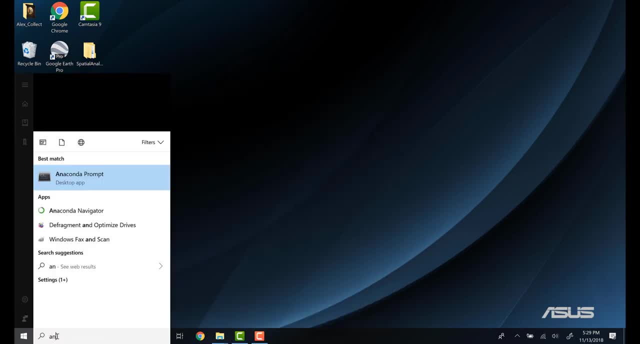 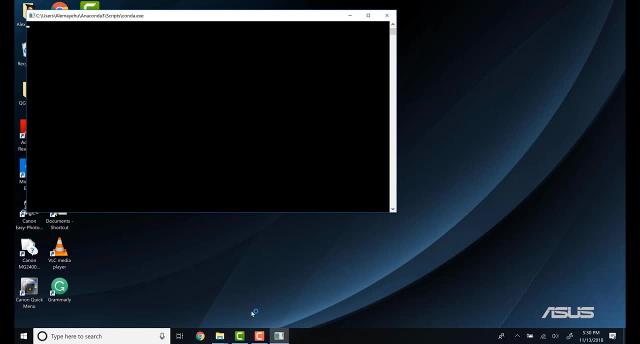 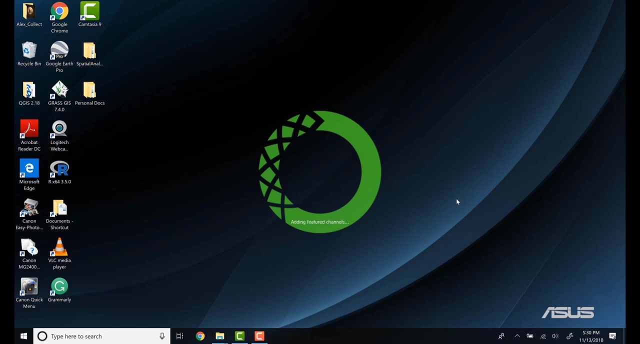 definitely use the Anaconda. Okay, So you can use the Anaconda you know navigator, just if you want to do it manually, And once the Anaconda navigator initiates you can launch a Jupyter Notebook, okay, So that's kind of a manual way of doing that. 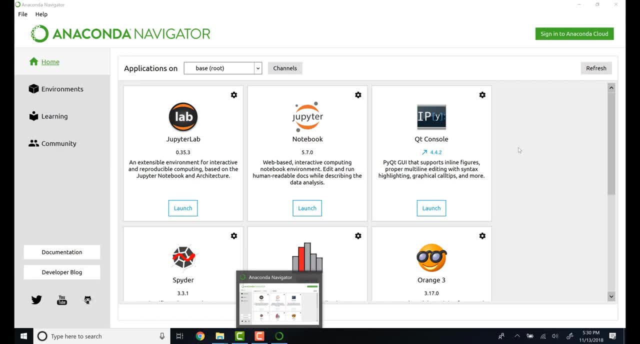 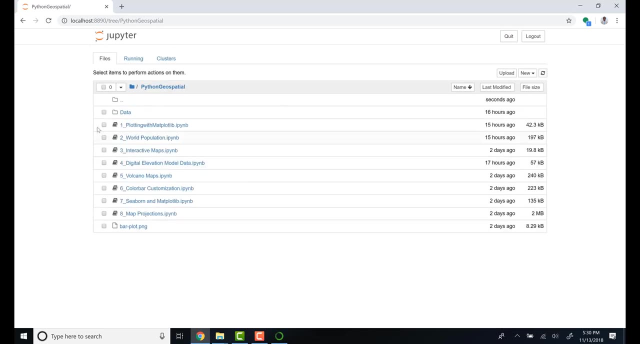 And so Anaconda is just configuring and initiating. So once you have the Anaconda navigator you just launch Jupyter Notebook, all right, And then you just go to the folder that you have your all you know scripts. I mean you can, you know, save it in a different location if you want to? 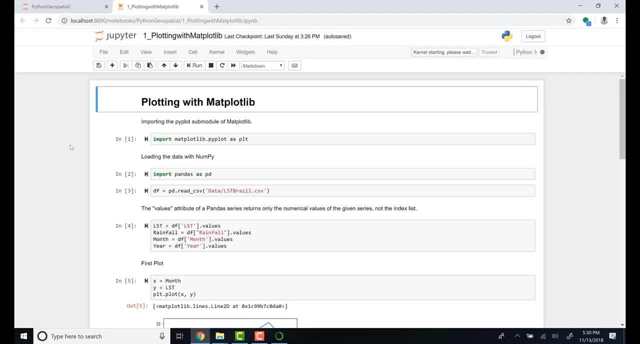 So let's get started with the first you know code, Python code that we have. So the first thing is: this is just you know, an exercise where we will do some demonstration on Jupyter, Okay, Okay. So the first thing is: this is just, you know, a demonstration on how to plot is in matplotlib. 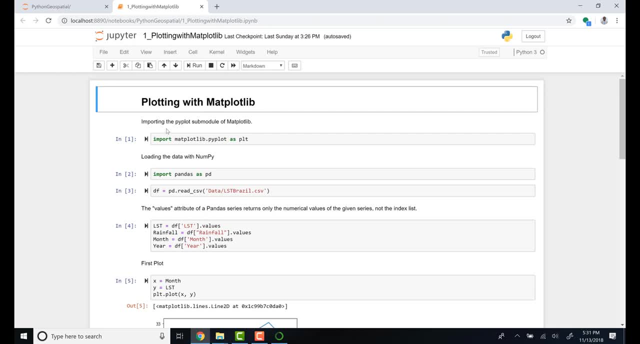 right, And so this is kind of an interactive you know platform to code, you know Python, You can, you know, create new cells, For example here: if I just create a new cell here, it will open. 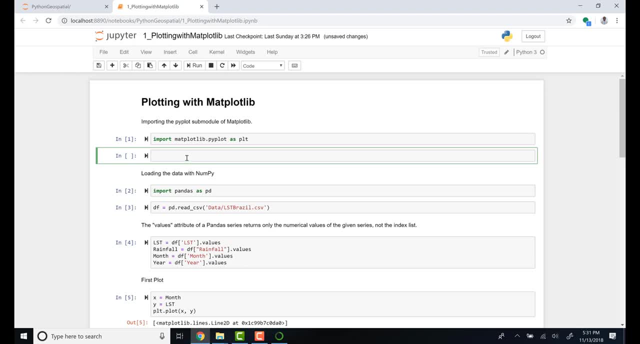 And also, you know, if you want to write a code, like for example, import pandas, so this is just a code, right. And if you want to like write a node, you can change here, like from a code to a markdown. 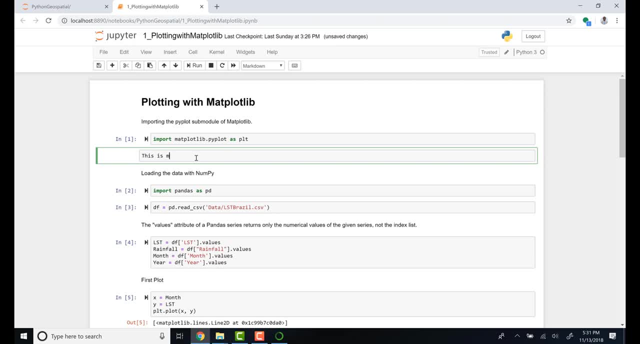 And you can say like this is my code right. And then if you click it's not running, so it's just a text file. So you can change that here. And then, if you want to like move this cell, you can just move it up and down. 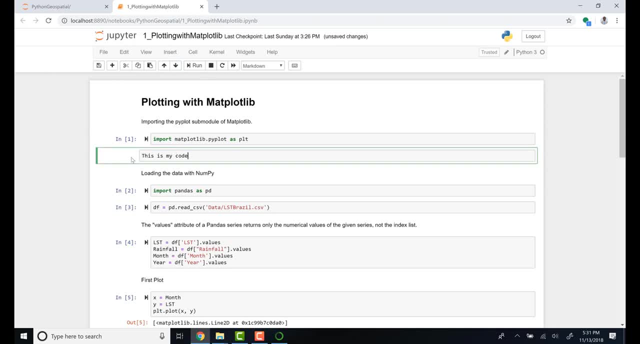 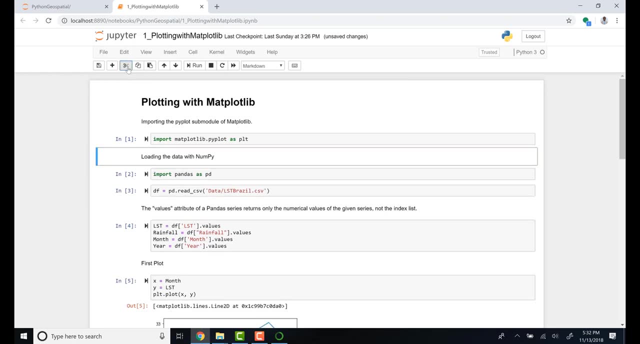 If I want to move it down, I can do that, I can do that and I can, you know, edit that, just delete that. Even I can delete the entire cell, like I can cut that and just delete it. So it's a pretty cool interactive platform for coding. 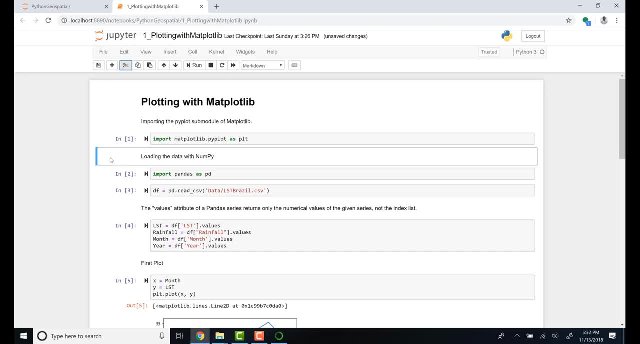 So it's a code editor, but it's interactive. You can, you know, add code. you can import data. you can you know print. you know your intermediate results. You can also plot. you know time series. you can plot maps for geospatial data. 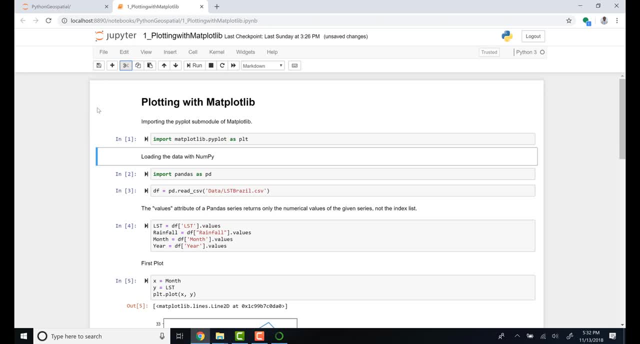 So that's kind of an overview of you know Jupyter Notebook. So let's get started with our you know plotting. So the first thing I'll do is just import matplotlib package and pyplot as plot. So if I, so, if you want to run a script, so this is our first line, you just go ahead. 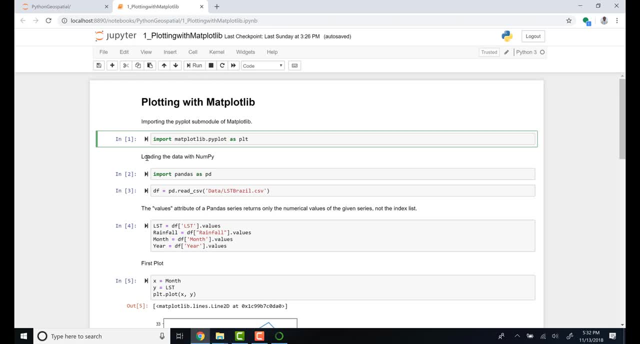 and then do that. If you want to run it, you know line by line. So this is the first line of code And then, if I run that, it's so loading. the data was an mpy and I think let me just remove. 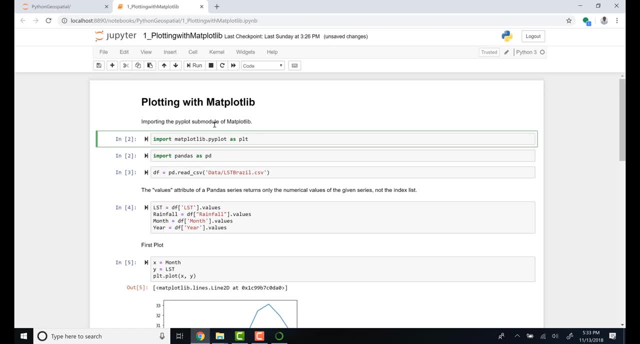 this line, okay, So if there's no issue, it would just, you know, keep on running the next one, So just, and then let's also import, you know, pandas as pd? Okay, All right, But mind you like before we import the data, if, in your case, you might have problem with. 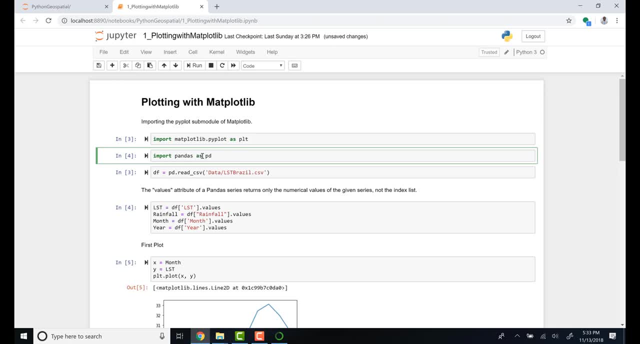 when you import the matplotlib and then the pandas, you have to first install this package right, And once you install it, you can- you can, you know- import it. So let me show you how you can. you can install a package for the Jupyter Notebook. 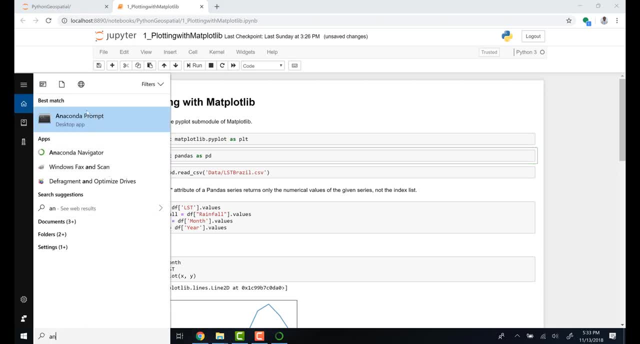 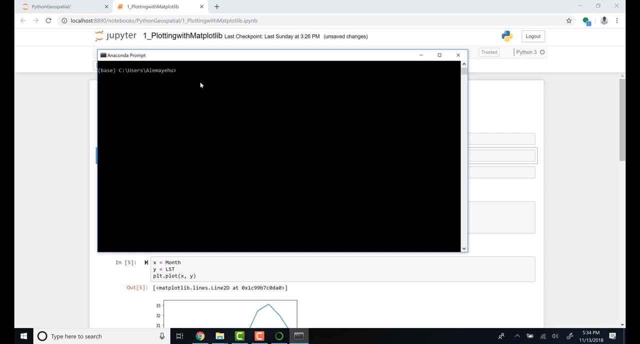 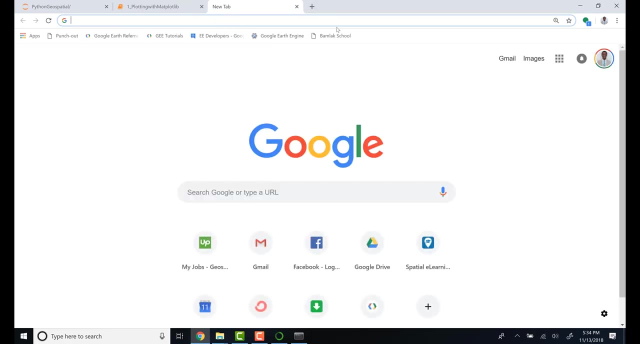 So let's go to the Anaconda prompt. right So that's how you install packets, For example the pandas. right So to install any Jupyter, any python package. let me show you like. let's Google it like. 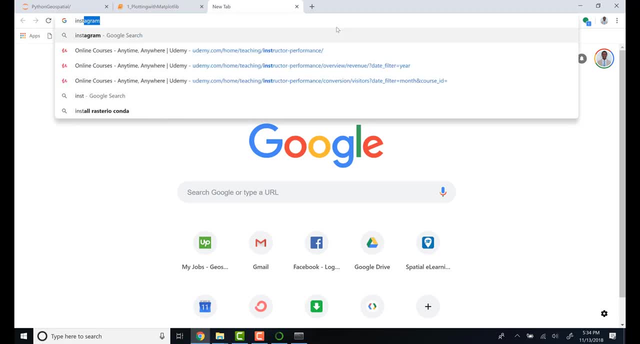 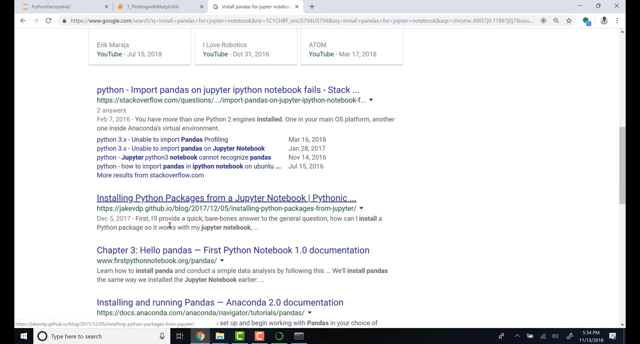 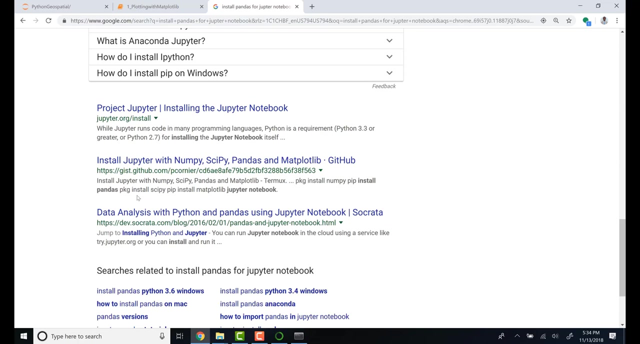 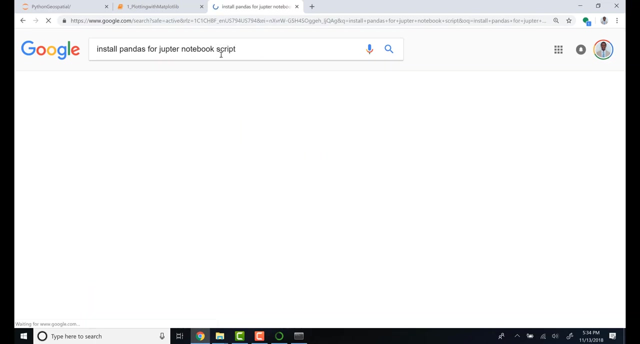 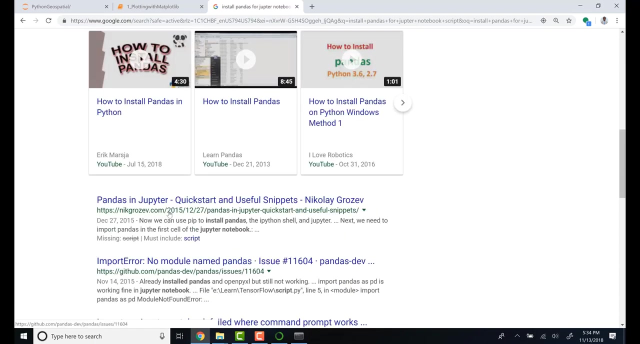 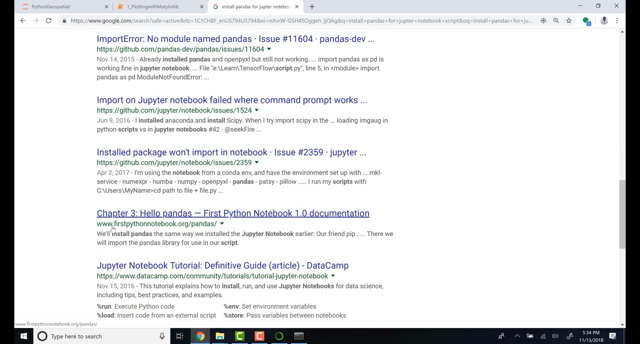 install. install pandas Jupyter Notebook. right, so if you, if you, just you know, click here, you, I'm just looking for, you know, sample script like script, just want to show you how you can get like some codes or how you can. all right, there's not a lot much, okay, so let's just go back and 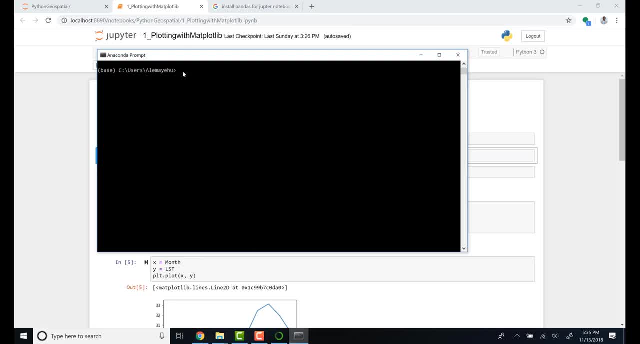 let's go to the you know anaconda prompt and let's do install the pandas package. right, but I have, I have already installed it, just, but for you, that's how you install it literally. you so conda, right, conda, install pandas. that's the package that you want, if it's. 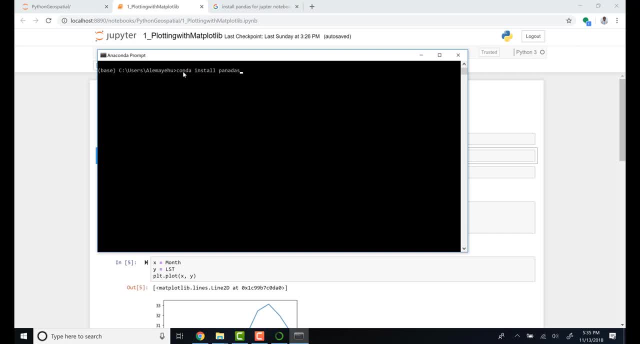 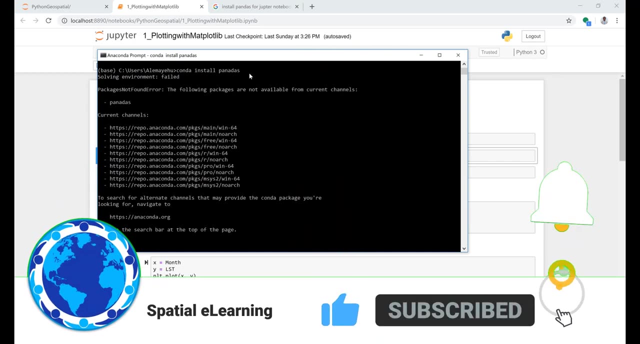 a different package. you write so conda install. you know the name of the package and just you. you hit enter. now it's just active. is he solving? environment says it's. it's attempting to install that. so it's just responding. so this is a line of code that you need to know whenever you have you have to install some package. 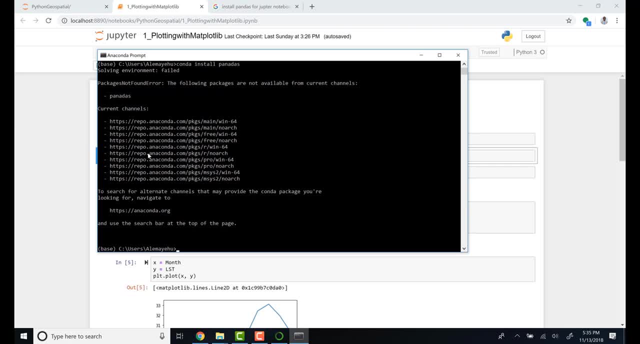 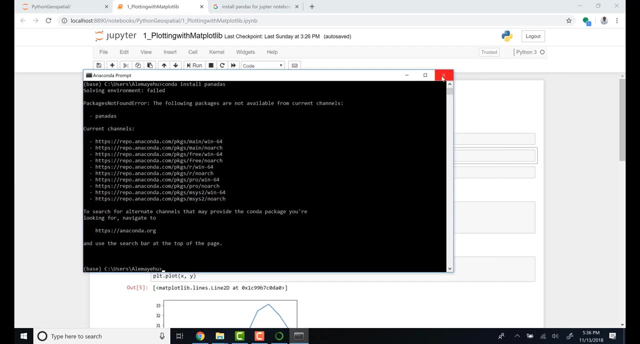 in this weird package. this is how you install it all right on our Anaconda prompt. okay, so it says that you know the following package are not available from the current child, but it's already, you know, installed. I think that's the rate, the reason that it's not you know, letting me do that, okay, and if your package is, 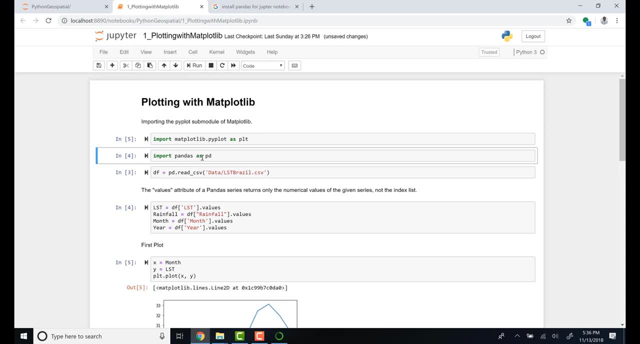 not installed. if you run here, you'll just- you know- see an error message. if it's not showing you here, then it means that your package is already installed. because if you have got the different packages or these accounts, is happening back on yourious one of your accounts. you do not always want to show up on the. 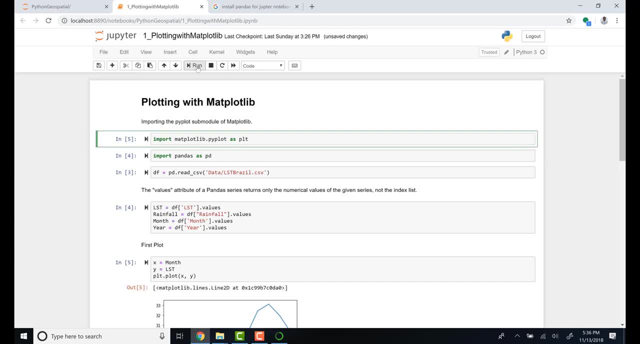 account here. it would cause that problem like locked, you have to go global. we'll have to manually log out of your account just to make sure of all of this stuff here. if this是, and then it's, it's importing it, so no issue, right? okay, this is the first. 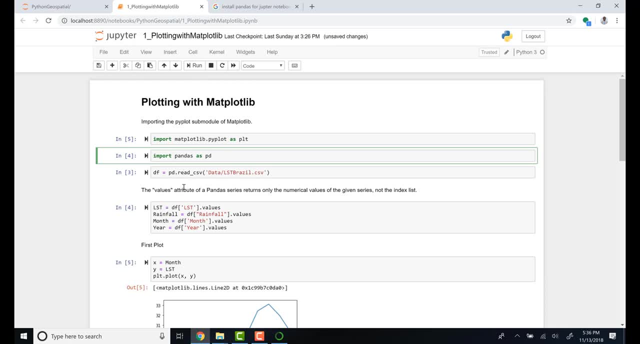 housekeeping that you need to know before you. you just go in some tips, right, okay, so run the import, the my plot and the pandas, and then this is where my- you know- data is saved. so so I'll define a DF PD as a pandas and really says: if 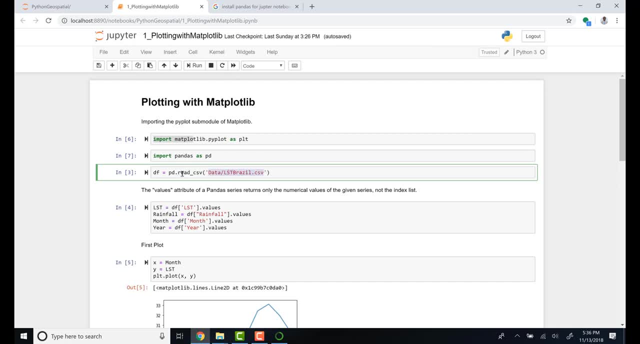 you, so technically, I'm writing the name of the fight. another thing that I'd like to show you is just, you might be interested, where is where? should I put my data in it on all my scripts? so where is that? you know? let's just add another. 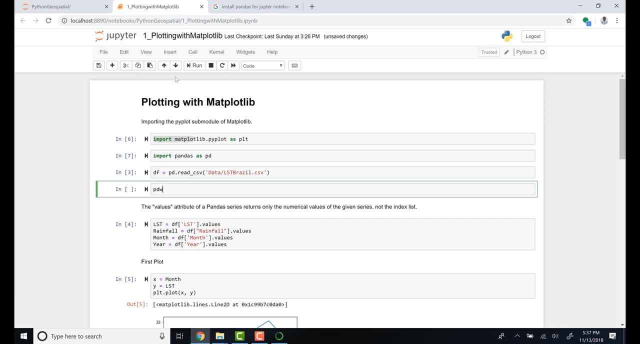 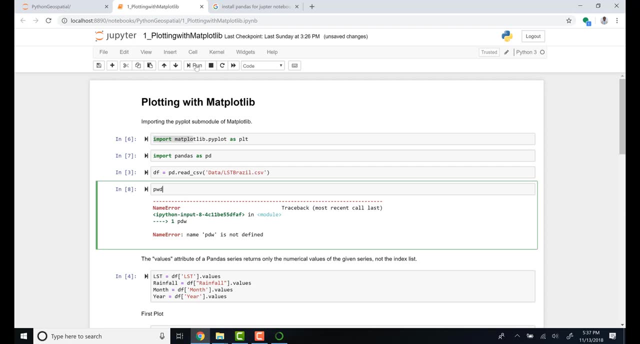 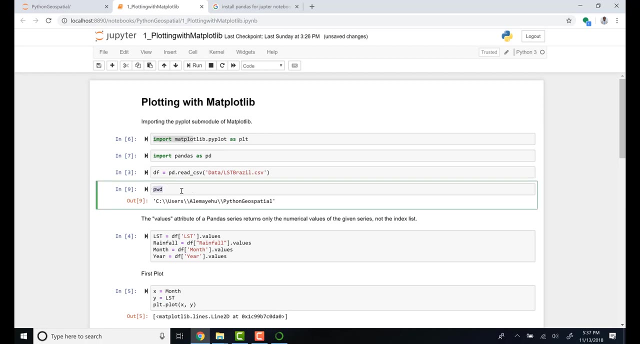 line here. I think it's PW. let's just try that. okay, PW deep. okay, all right, perfect. so PWD is just you're working on. if you're running something on it, you have to run it on your found, you know, directory for for this Jupiter notebook. it will, if you write PWD it. 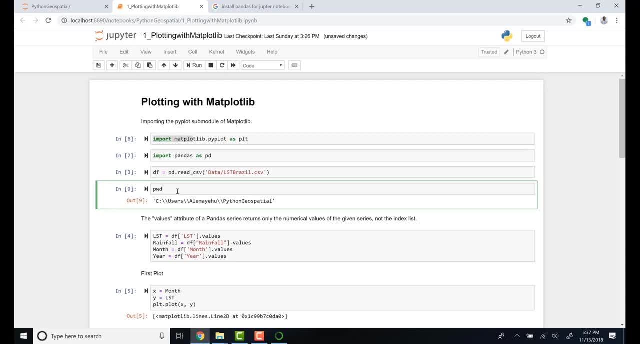 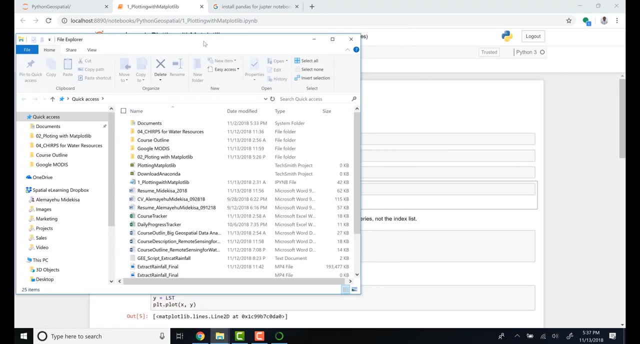 will tell you where you're. just technically you're working directory, right? see, if I go here, see users, you know, if I go to this file I'll get my all my- you know- anaconda codes and all the input data. that's just my working directory. so let me go to C and users and then 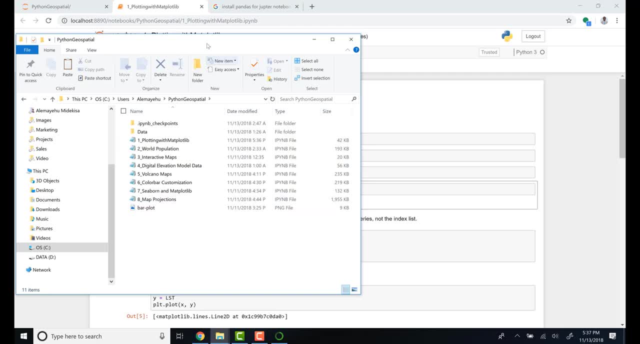 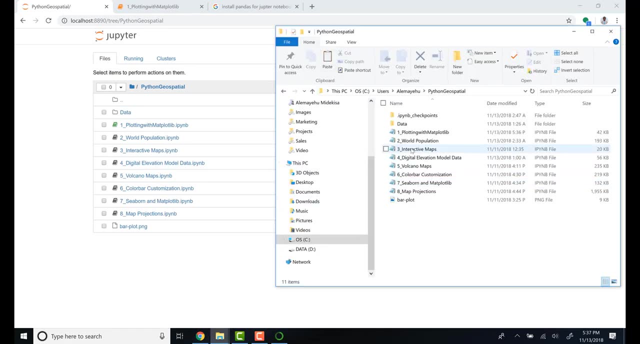 Python geospatial- that's where it is. okay, so you can see all this. you know all these. let's go to the main page. okay, so you can see all this codes right here. right, you can see all of my. you know Python and you know chords with IP Y and B. you know. 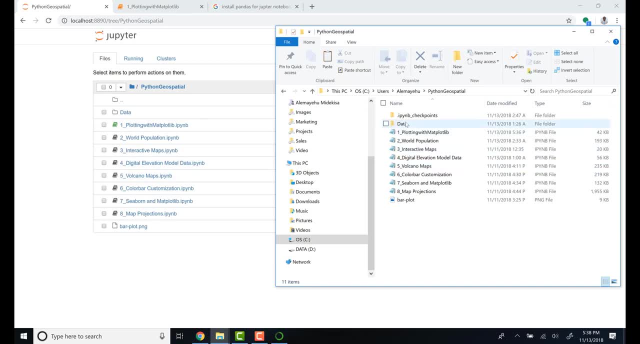 suffix. so you can see all of this course, right, and then my data is here. you go see all these codes. you know suffice. you can see all of these codes mine cities and donde la ciudad. you can see all these codes and you know all i步 am iąbeä walk around. you know my city, so then my data is here. 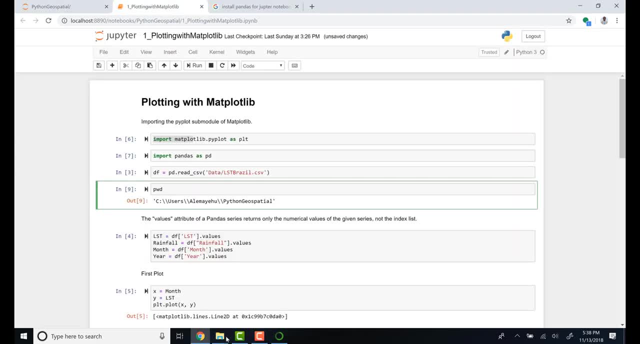 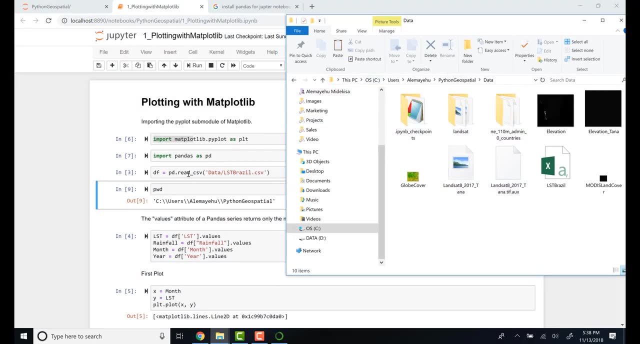 here. So that's that's how you. so that's how you write, like your data. So this is your working directory. So when you write the file name, you just simply, because this is our working directory, you know we're writing here: data LST Brazil. So data LST Brazil. 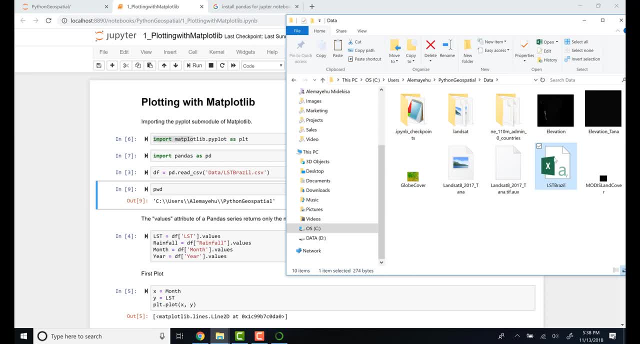 LST Brazil. here's the CSV file. So that's, we're just technically calling this file. So for, in your case, the first thing you need to know is just to locate your working directory right By writing PWD. Once you know your working directory, create a data. 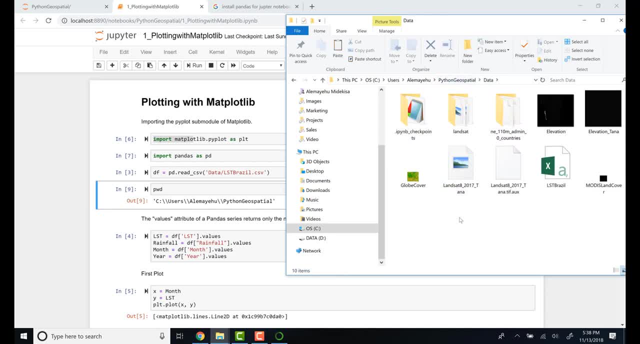 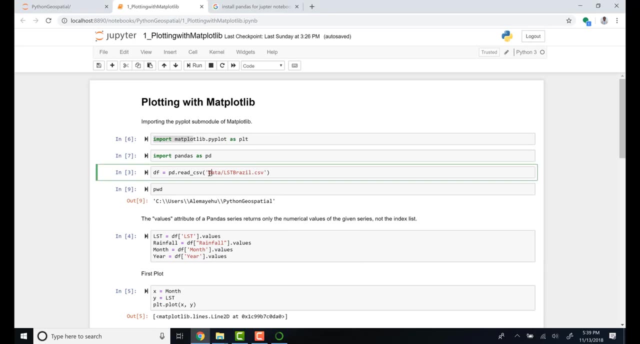 folder and a data folder and try to add, you know, the data, the data files LST Brazil and put it there and that's it, And just write this. you know, write the script and just run. it should run smoothly, Right, That's the first thing. 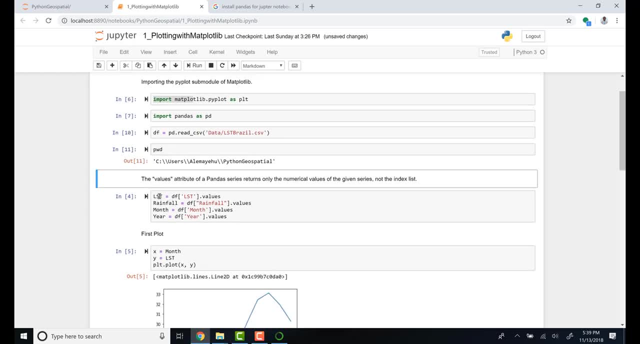 you need to know. And then, once we imported the data, let's just call. so our data is just DF now. So let's select some variables, right. And the other thing is we might be interested to do like DF head. 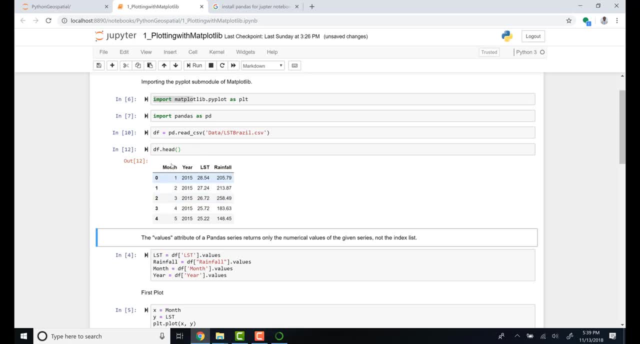 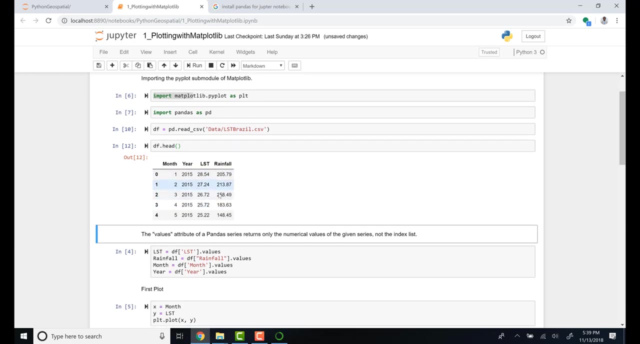 So if you write DF head, then you know what the different columns in this database are, right? So I have a month's parameter, a year parameter and LST and land surface temperature and rainfall. This is for Brazil, right? And I would like to map, you know, LST, you know. 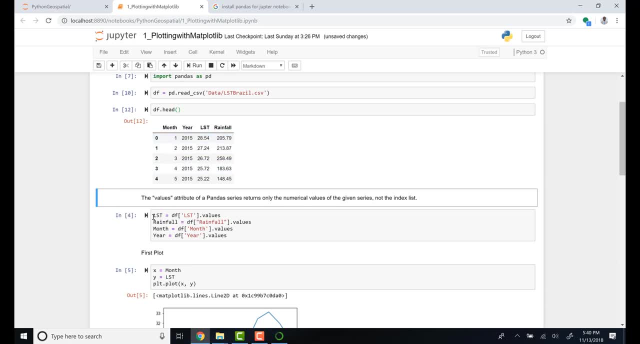 so I want to select. you know the different parameters here. So what I'm doing here is just: LST is equal to DF, So I'm going to go to the file and just write the name of the column here- LST, then value. 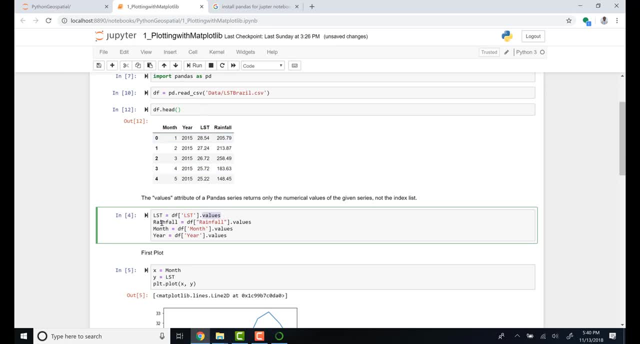 So it's just selecting that specific column, And then the same thing for rainfall here, And then the same thing for the months and the year. Okay, So now it's easy for me to plot. each of you know these parameters, right. 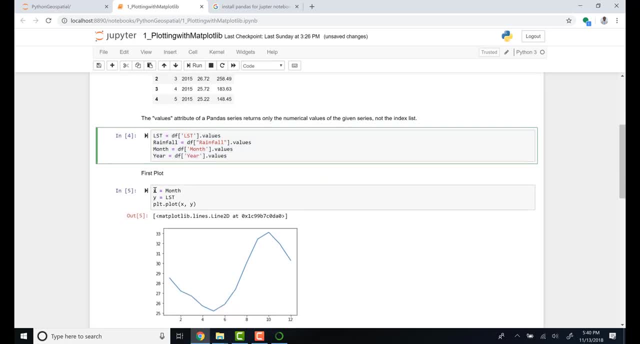 And the next thing is I define my X and Y parameters, because I'm doing, you know, line plot here. So So I'm telling like: so I want my X axis to be months, Here's months. We define that. And then the Y axis is just LST. So you know, the Y axis is LST, right, And then plot dot. 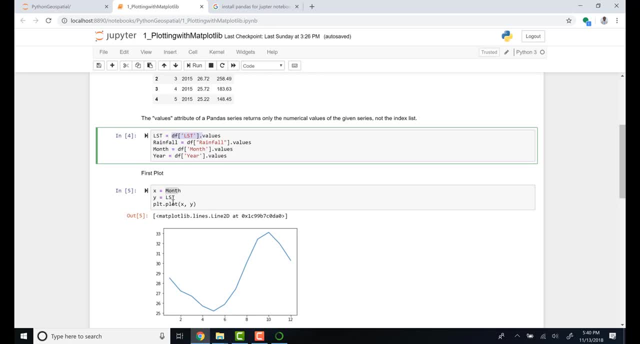 plot XY. I'm just plotting, you know, LST by month, right? And then you just run that. I'll have to just run this first. that's why, Okay Perfect, Because I have to run this. you know this pattern. Okay Perfect, Okay, Okay. testimony for doing this is this: you. can do this. This is the like. if you want to do like Nu possible, so, many, many of these. this is just like you can actually do this. Right, This should be fine. Okay, So this is what looks. let's do it. just do that. So use. this is what I'm doing here, here, So I'm working with the function you. 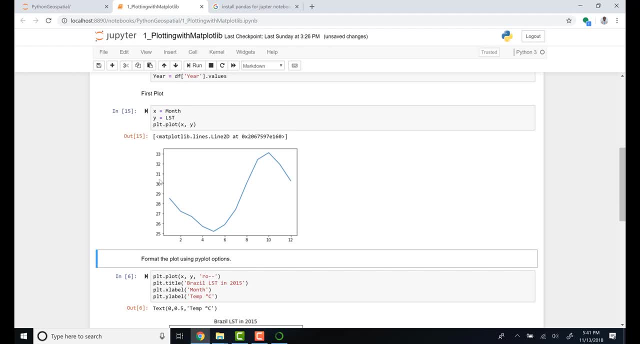 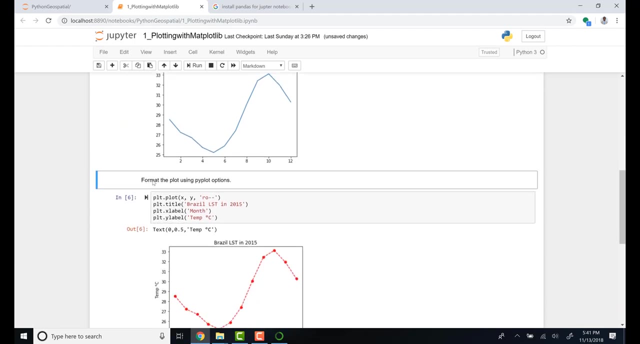 batch of scripts. So now we have made our first you know time series plot. So this is you know months of the year And this is land surface temperature values, you know for Brazil. And this is just you know basic, you know plot. So let's do some a little bit of you know. 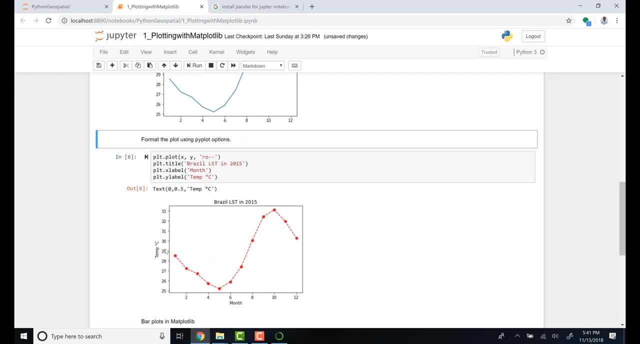 you know changing the color and then title, and you know the x and y axis, right, Let's add some. you know parameters, plot dot, plot x, y, and then add plot title. So we're going to write a. 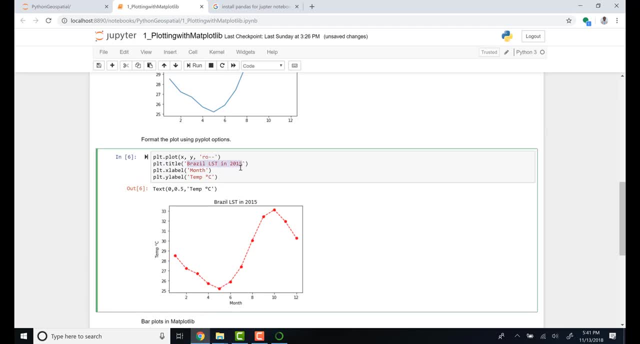 title here: Brazilian LST. Here is just my title. If I want to change it, it can change. And you know, plot x label, So this is our x label, and then plot y label, So this is our y axis. I can. 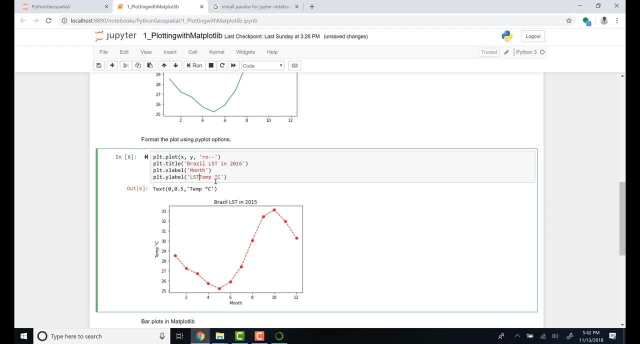 change. actually LST, right, Our land surface temperature in degree Celsius, right. So let's just run this. It should change right. We have temp here And you know months here. So when I run the script, it should. 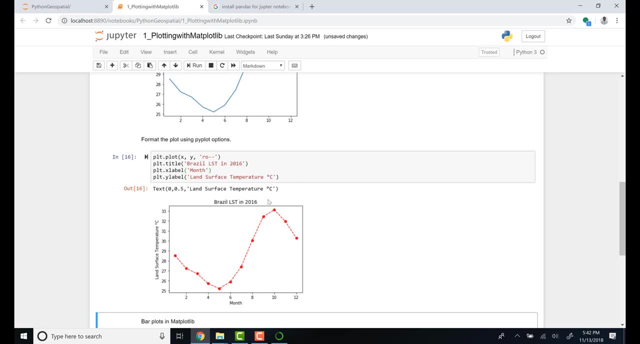 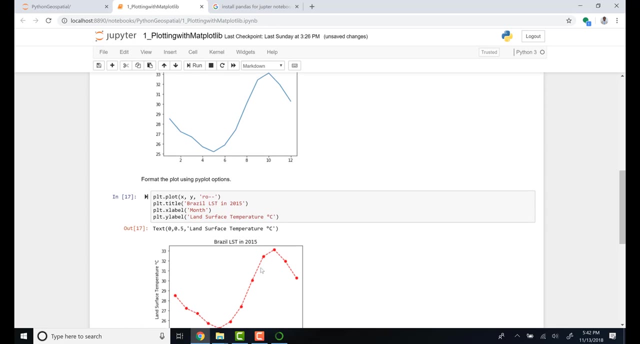 change, right, So land surface temperature is changing automatically. And then here was 2015 and 2016.. Actually, this changed that back to 2015.. Okay, perfect. So now we have also, you know, changed, you know, the color and the type of 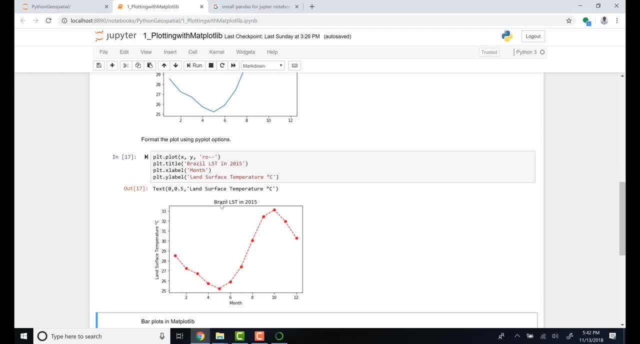 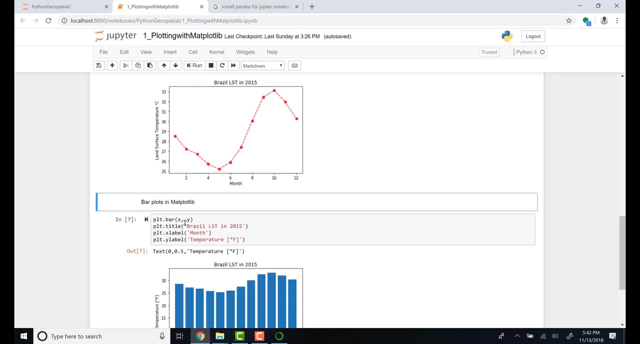 you know line And we have added a title, We have added, you know, x and y axis. That's pretty cool And let's do this is a line graph And then let's do a bar plot, So to do a. 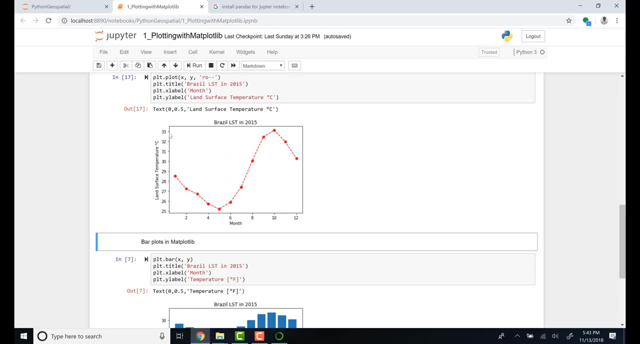 bar plot. instead of you know PLT plot, we do PLT bar right, And then let's do a line graph And then xy. So and then we also just, you know title, you know x and y label. So if you run, 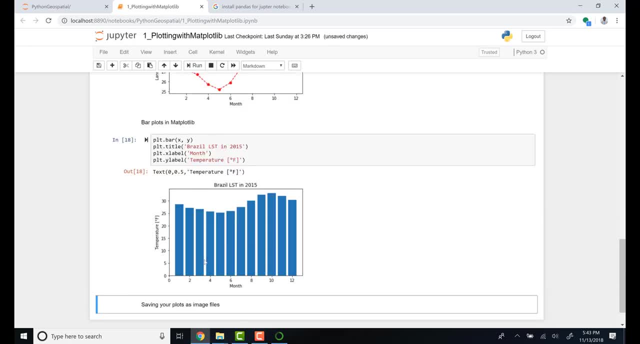 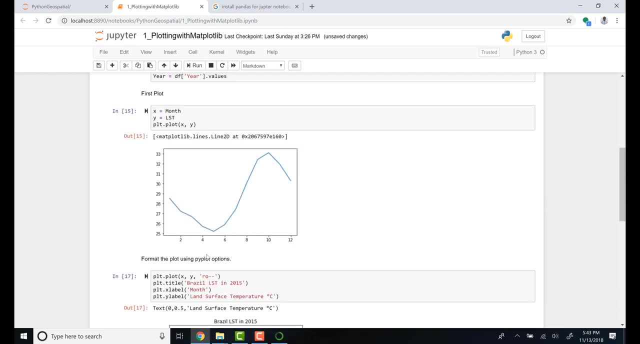 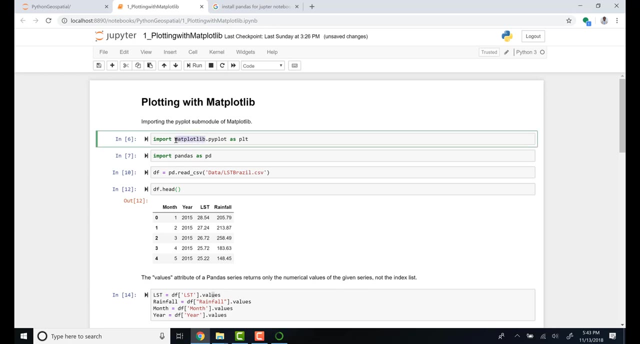 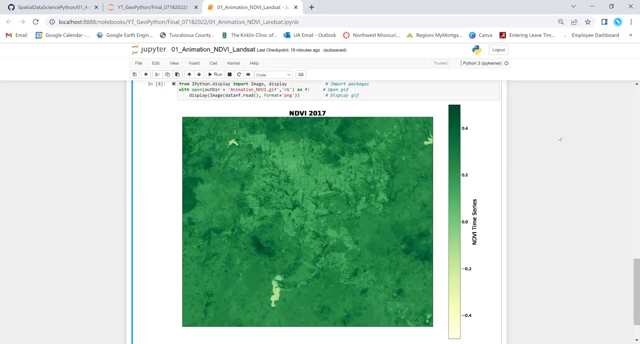 this script. it will just give us pretty nice looking. you know, bar plot instead of a line. So that's how we can do some plotting using the matplotlib package in Python- a Jupyter notebook, right. So in this lecture we'll be looking at how you can generate a time series animation using Python. 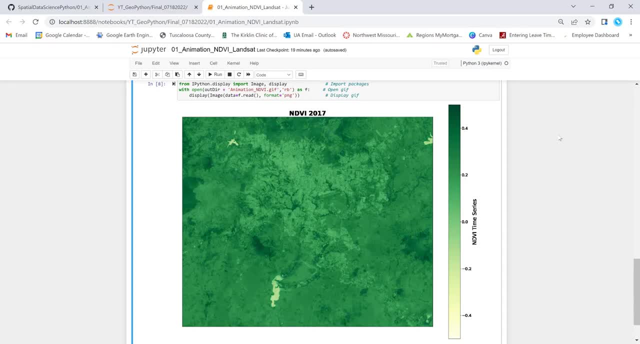 how can we automate the process using open source Python tool? if you have, you know multi, multi date, you know imagery or satellite imagery, in this case an NDVI, And we'll get. we'll get that done here. 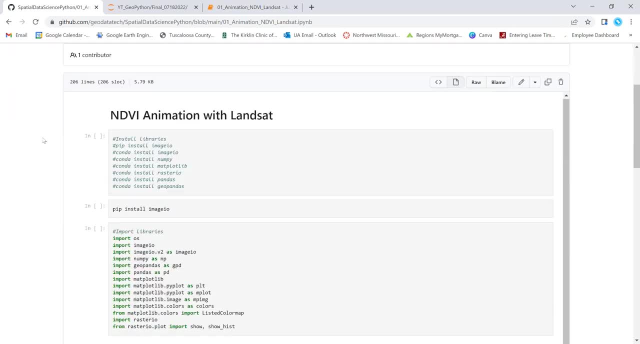 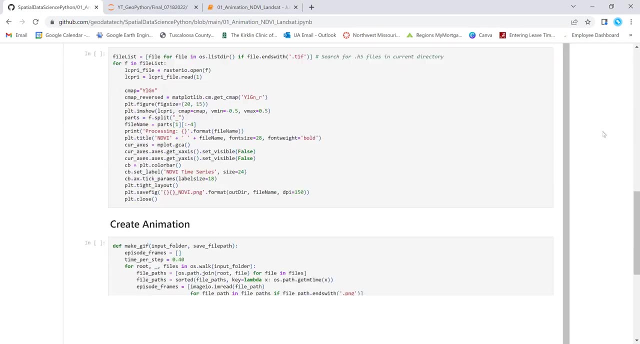 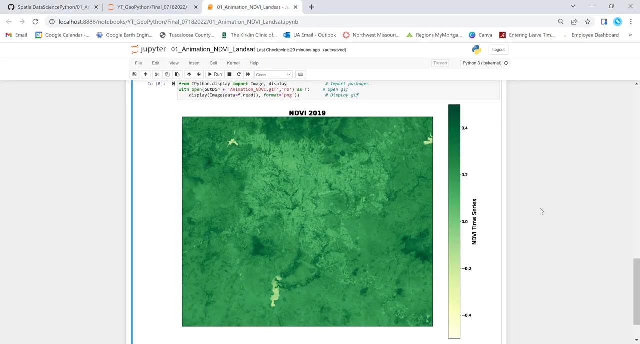 So I'll be using this bit of code. it's available on GitHub, I'll put the link below And this is the script that would achieve that. So in this example, I'll use NDVI, normalized difference vegetation index derived from Landsat image, and I have multiple years of data And I'll be able to use this. 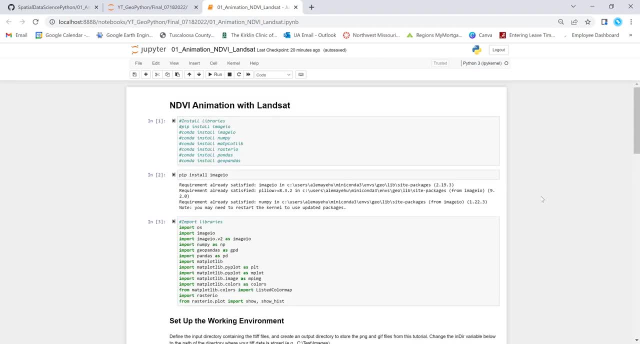 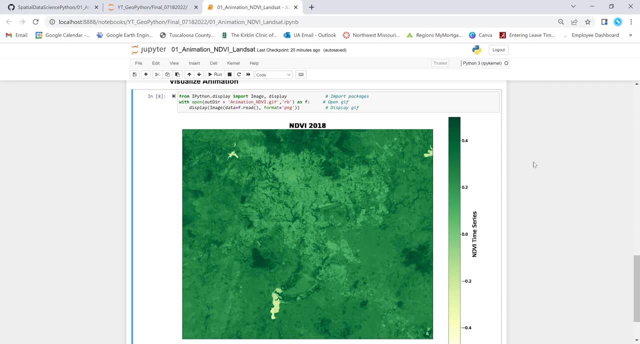 code to generate the time series and pretty much you know well, you know well documented in terms of you know color bar and title and things like that, And also the different years here to show that kind of animation, year to year variation or you know various temporal stamp. if it's a different data set, Okay so. 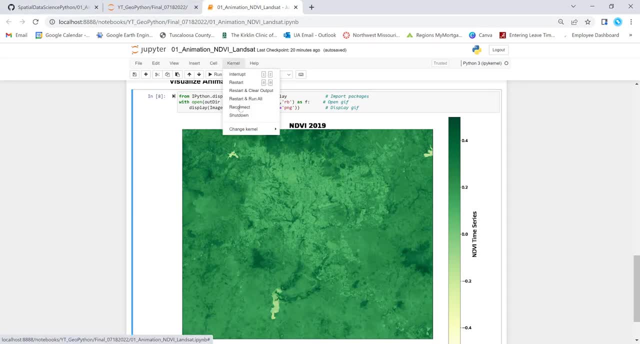 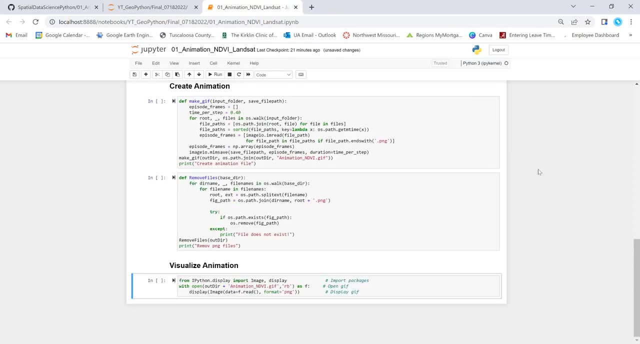 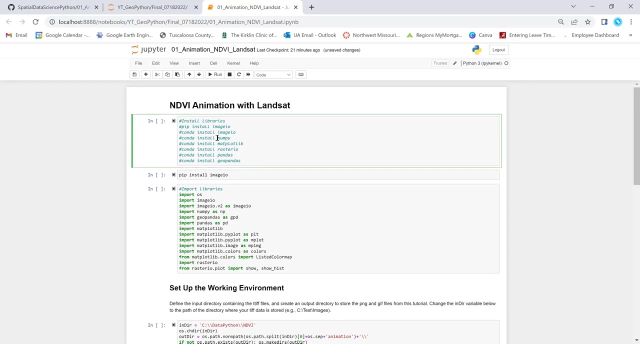 let's get started. And before I start I'll just clean up everything here so that we can run from scratch And that's clean. So the first thing is. so this is, as I mentioned earlier. let me just zoom in a little bit so that you can see the the code here. So this is NDVI. 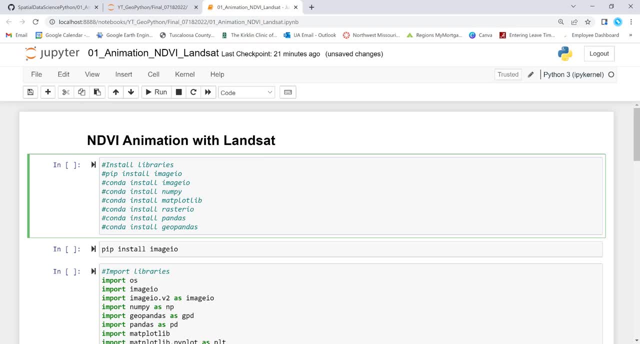 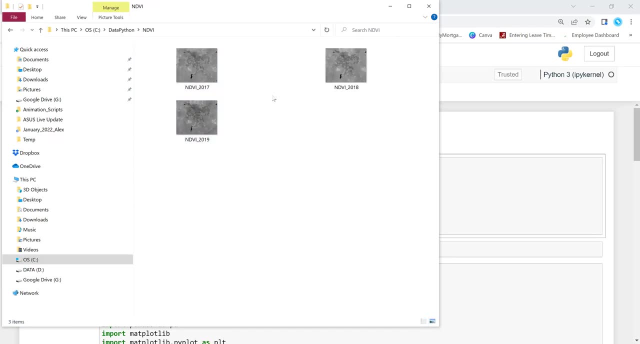 animation with Landsat data. So before we start, actually, let me show you the data set here, And so this is the data set that I'll plan to generate animation. I have multiple years, in this case three years. First is NDVI 2017.. And the other one is: 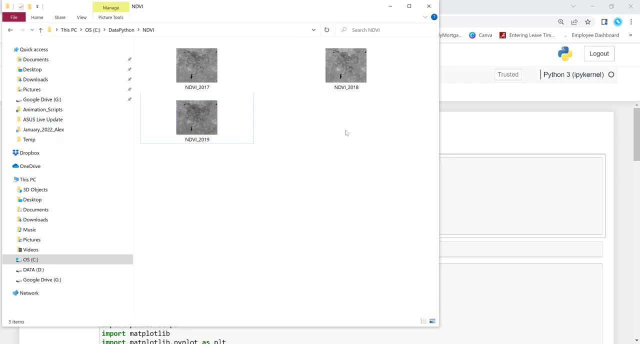 NDVI 2018 and 2019.. So I want to show a time series data And, using GIF animation, which is pretty cool and powerful, to show some temporal variation in your data. right, So this is derived from Landsat satellite, So I'll pull this data. 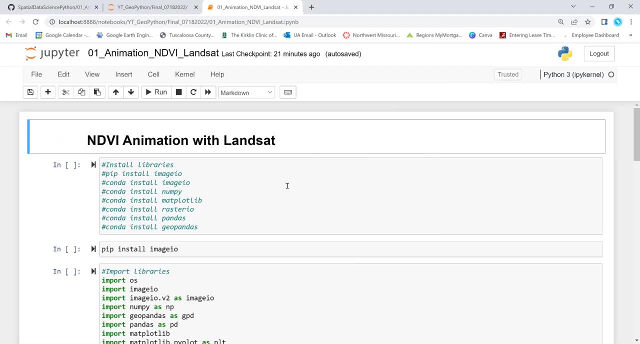 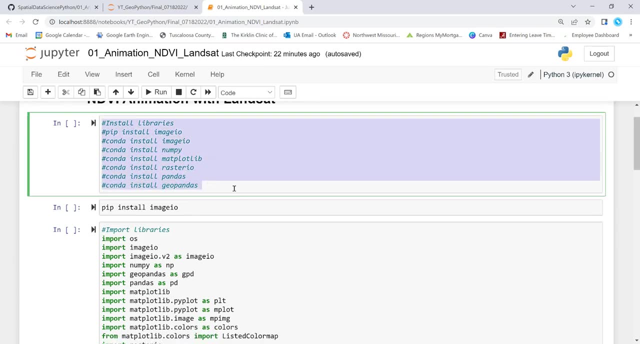 and just using this, this code, and we'll generate a GIF animation. okay, So these are the different, you know, libraries that you need to install. Most of these you can install them using Conda And all of this. you know Conda install Imagio and then PyMap. 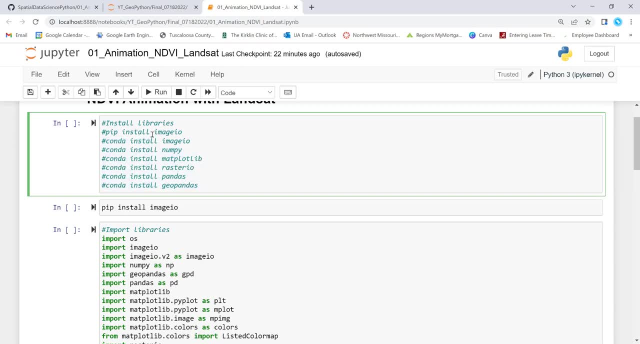 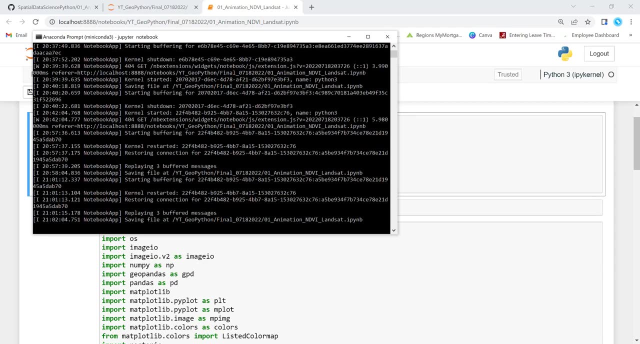 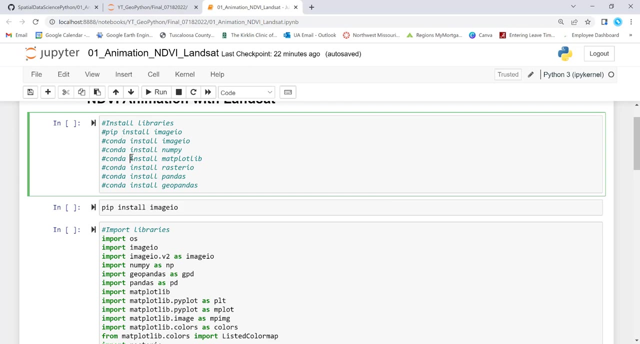 Plotlib, Rasterio, Pandas and GeoPandas, And then Imagio. I'll install it using a pip install here in the Jupyter notebook. okay, And I've already created. you know my Conda environment. you need to create one if you haven't done so, So you have to install all of this package in a. 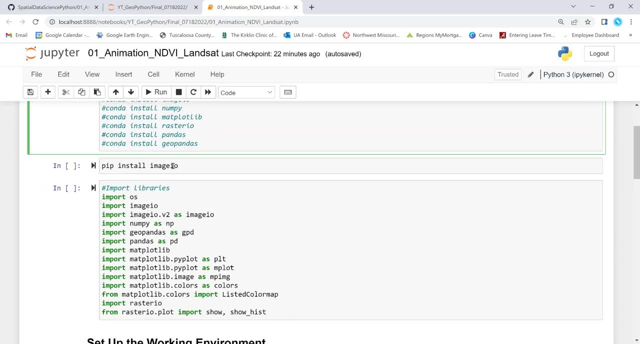 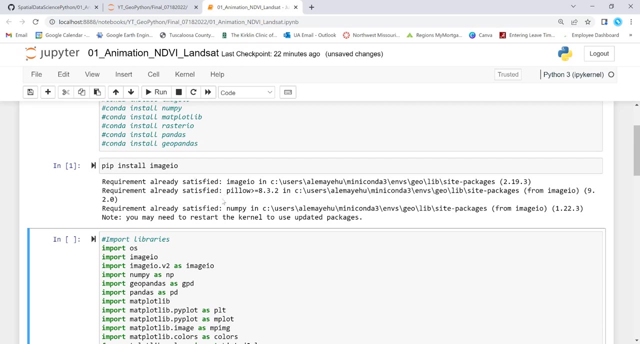 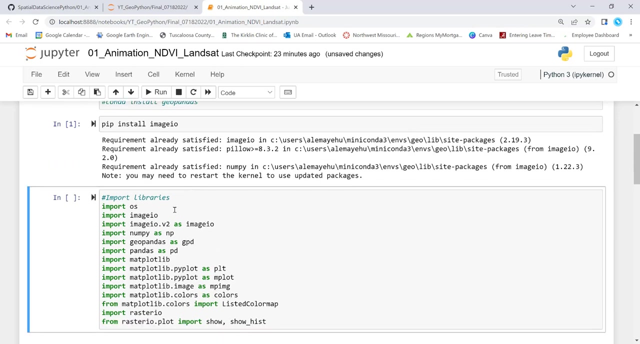 Conda environment, And if you have done so, then let's just get started. So go ahead and then execute this pip, install Imagio. it will import, actually install the, the library Imagio, which is powerful to generate, you know, GIF or animation, right, and here I have a bunch. 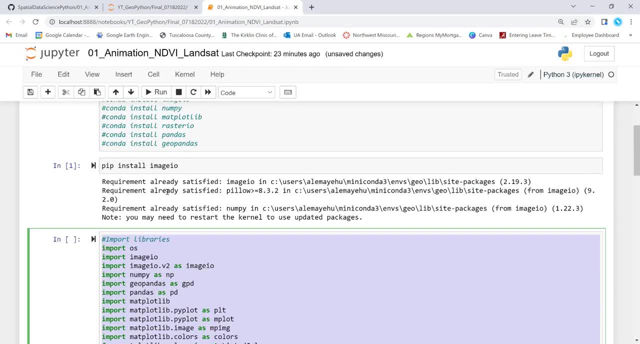 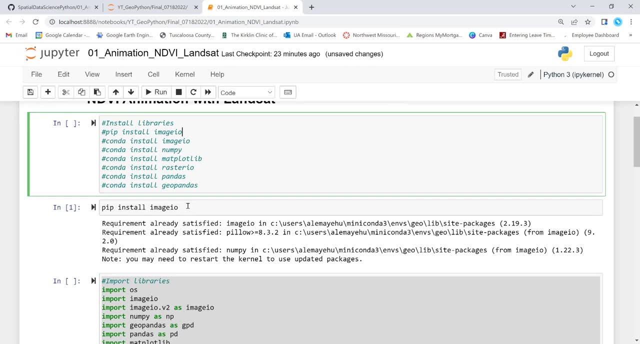 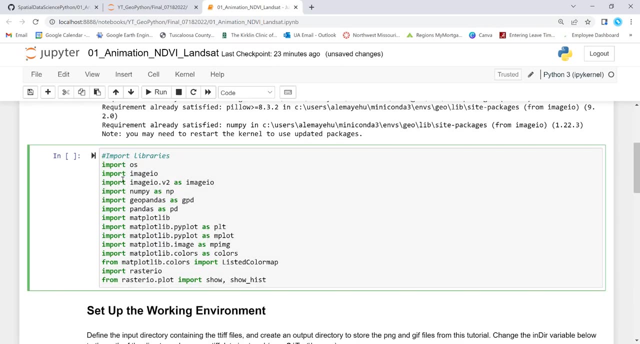 of you know libraries that I import. I've already installed all of this. you know libraries, you know using a conda environment here, so I just need to import them. if you have not done so, just go ahead and install all of this in a conda environment, and I have. I'll execute all of this to import all of the. 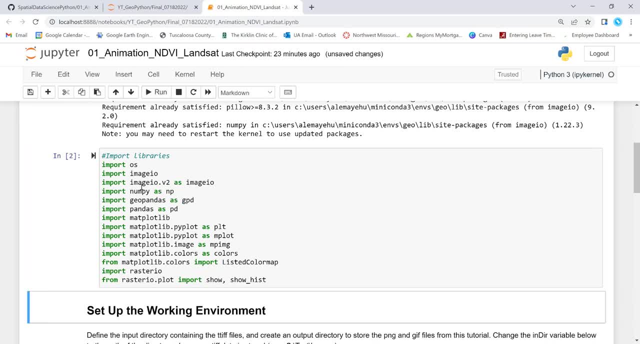 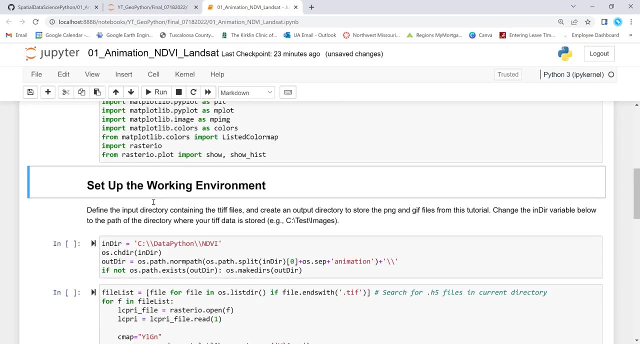 dependencies or just the necessary libraries to execute this animation, a script, and so it has imported all of them. so I don't see any error. and the other thing is I'll set up an environment where I can access my image here. I've shown you already here. 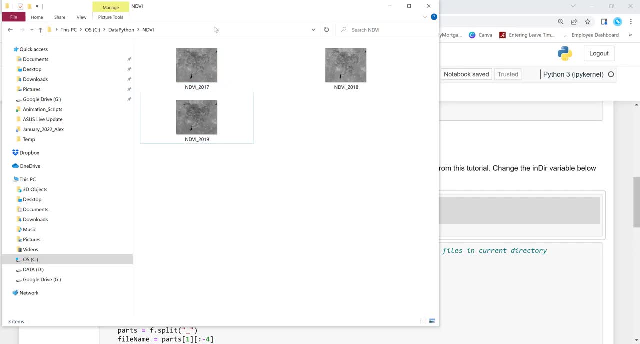 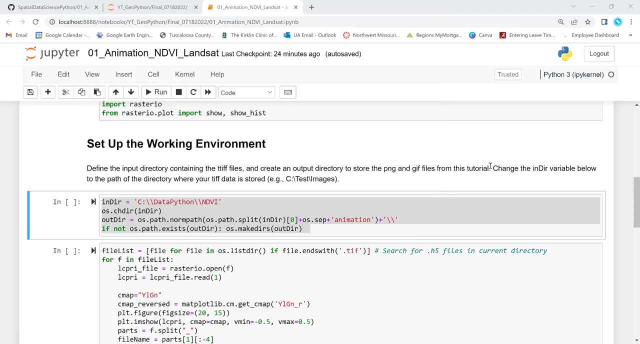 right. so I need to copy paste- you know- the directory for this so that I can access this raw imagery to generate a time series animation. so I just copy pasted that. you can change this into wherever you put that you know raster image and the other thing is this will generate an automa like a new folder. 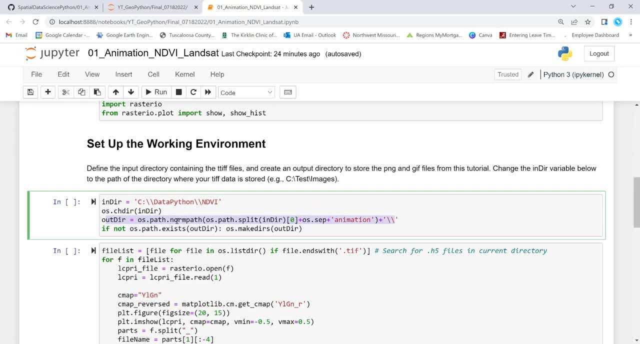 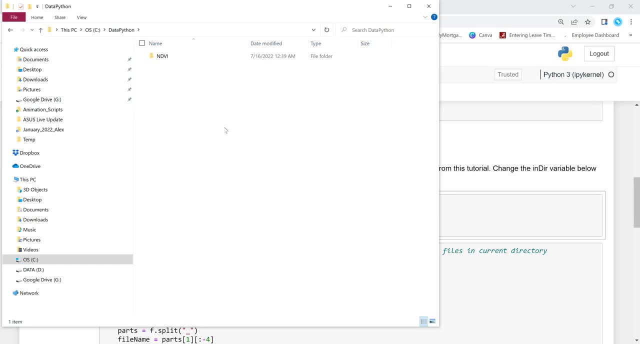 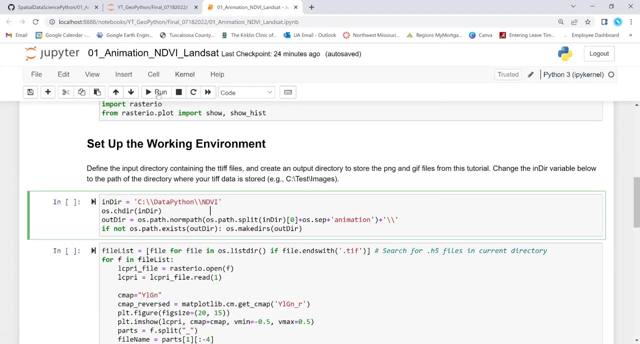 called animation so that you can store all the animation files. so when, when I execute this- as you can see here, this is my main directory- and when I execute this, you will create a an animation for empty animation folder. let's just check that once we execute this code, it will- it should- create animation. here you go. 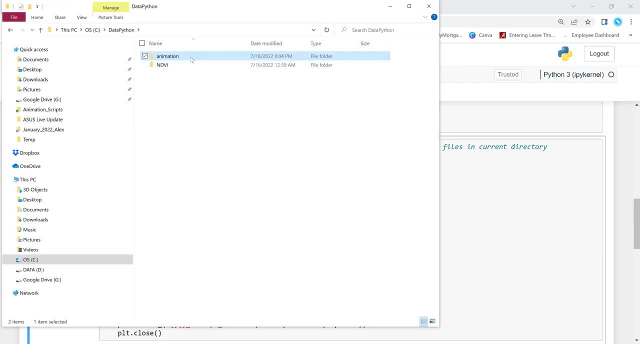 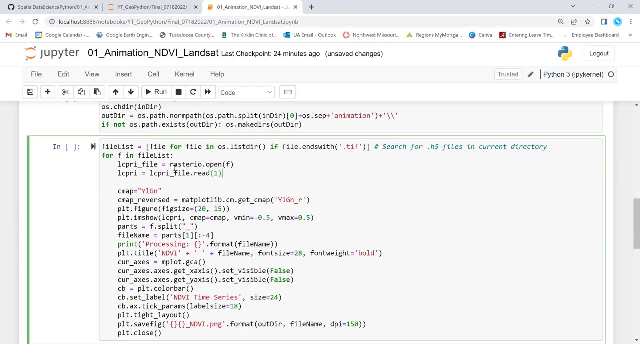 so we have created that animation folder, so it's empty, as you can see, we don't have any, any G file. so the next step is actually to you know, access all of our images. you know the file file list, you know you can, you can write this bit of: 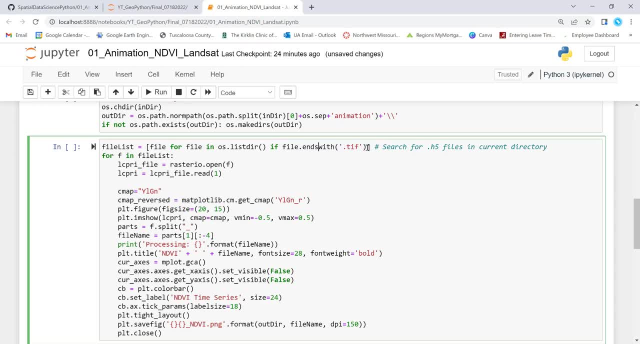 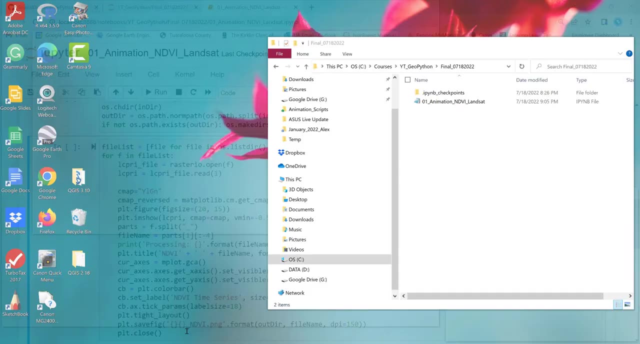 code and the file name here is T file, that in Swiss teeth. I can just edit this and save that. so the first thing, what it does, is just list the the teeth imagery. sorry that let's just go here, so it will just list. we'll go to this. 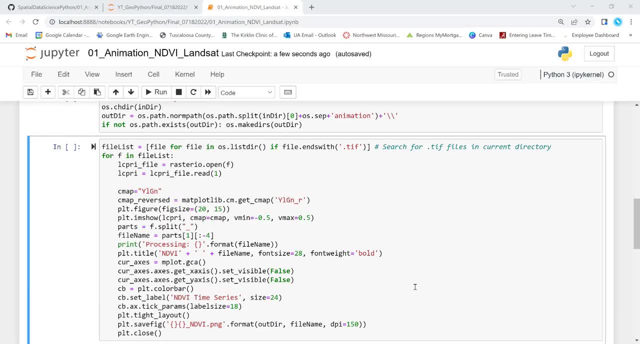 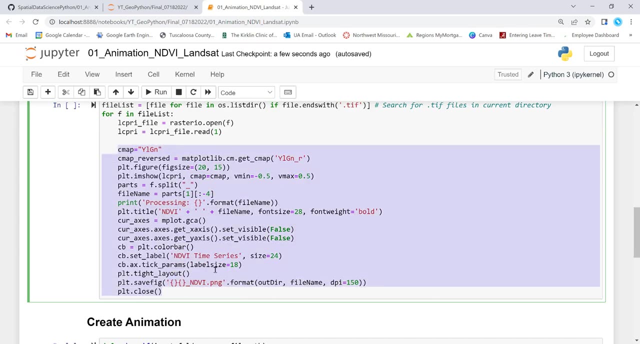 folder and list all of the imagery, okay. and then for each image it will, it will actually read that, using the raster, your package, okay. and once it reads that, it will generate a plot, okay, all of this bit of code will help us to generate, you know, the, the code, sorry, the the map, and actually we can, we can. 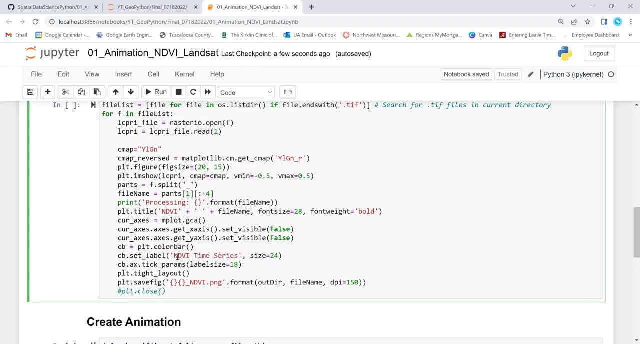 plot that if you just comment this, it will generate that, that time series. so let me just give you a little bit of description what what this guy's do. so CMAP is a color- yellow, green color. you can change this if you want to, and if you want to reverse the order, you can change. you can apply this or 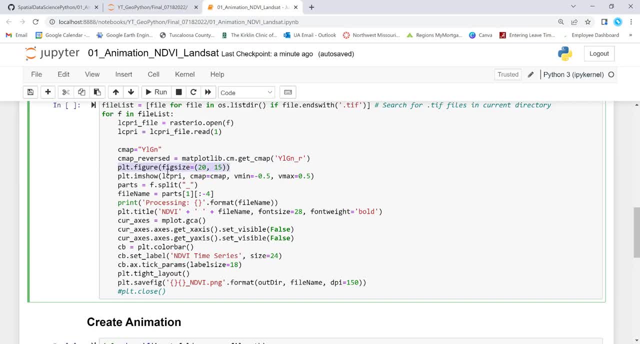 sometimes you can comment that, and this is the dimension of that, they eat the. you know the, the layout of the, you know the plot, the graph, 20 by 15 and finally, this will achieve or execute the plotting. so just you're technically using plot image show, I am show. LCPRI is the, the data, the. 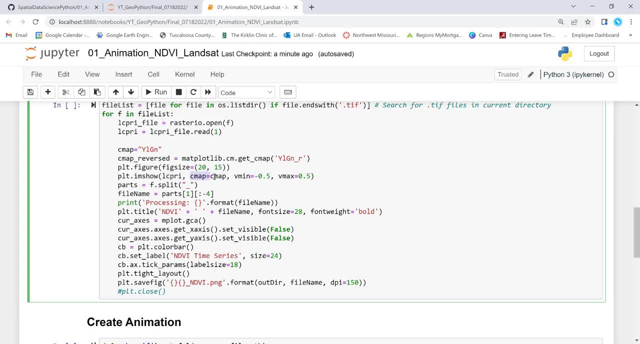 roster. you have already already using the raster you and then see map, is your color right? and so I mean you can. you can pull this to a river, you know, into a river reverse. or you can apply this CMAP reverse if you want to invert, you know. 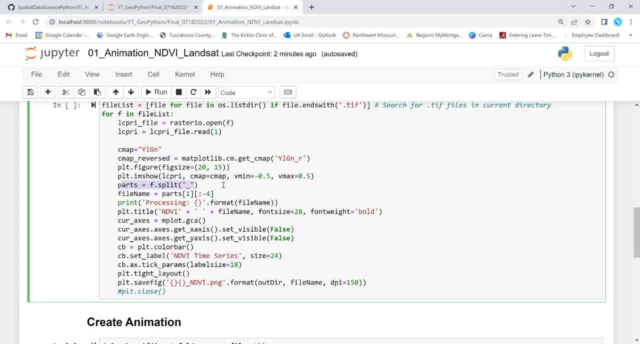 the legend and now just list the data and you know, generate some sort of title. here you can generate a title to the time, to the, the plot, and some you know axis, and also some you know title for the color, the color bar, and actually save the file using. you know the year, in this case you know 2017, 2018. 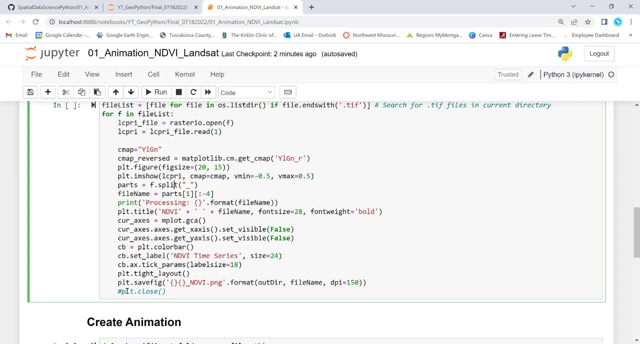 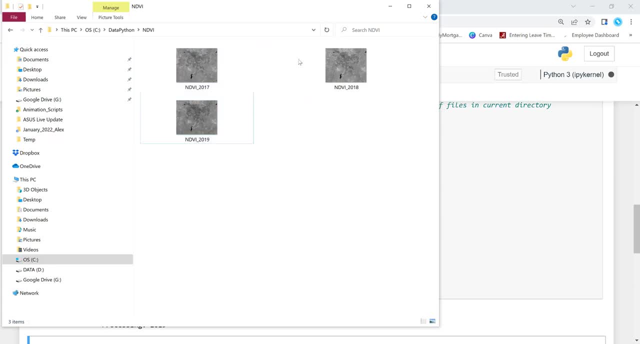 and 2019 and the NDVI. so let's just first execute- you know this, so that we can see some. you know some map here. as you can see here, this is just a great you know gray color NDVI image. all right, so this is what we have before we. 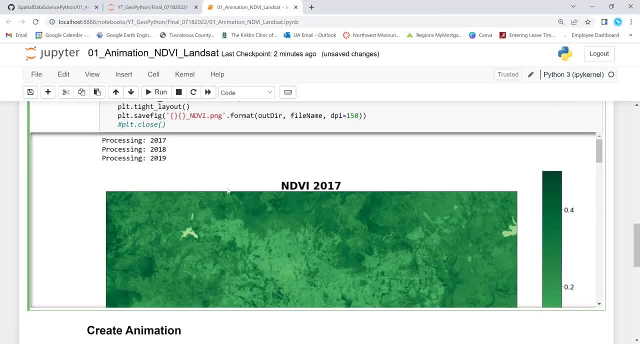 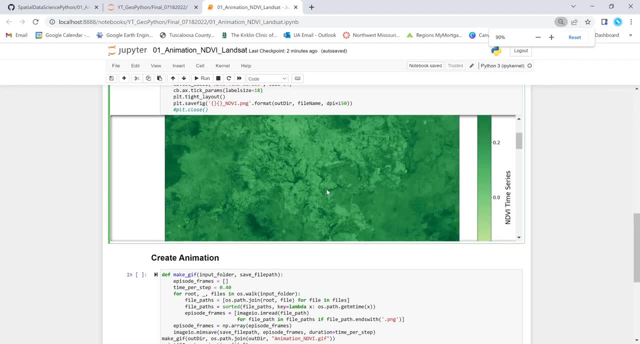 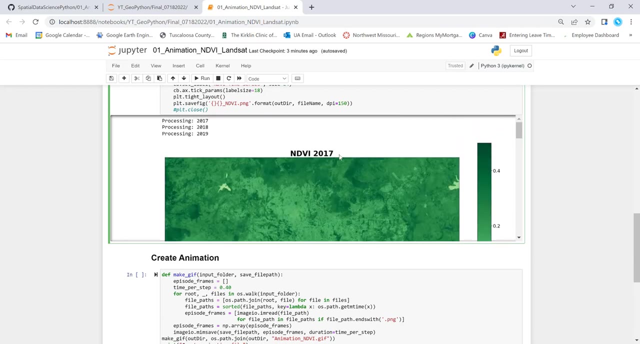 execute that code. now we are able to generate the. you know that times here is. if I zoom out a little bit here we can see: you know this is you know the time series and the plot. we have a title here, automatically generated in the color bar. here you can see the color bar and. 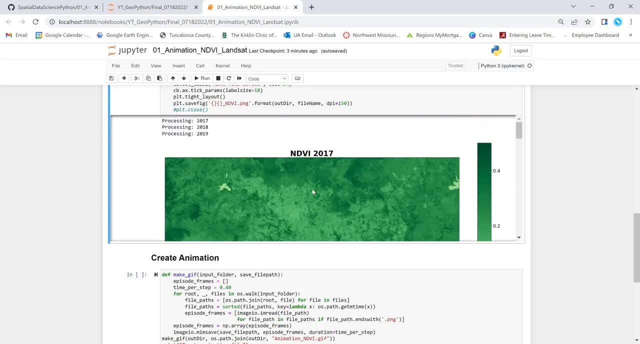 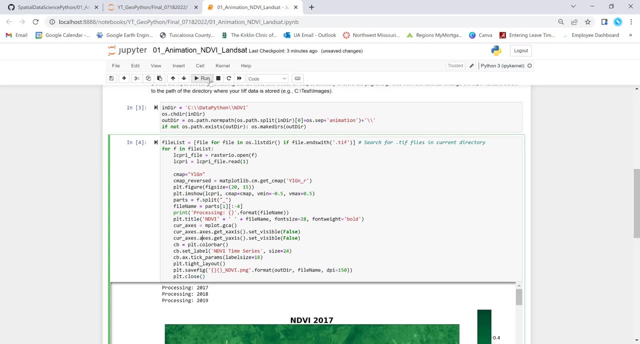 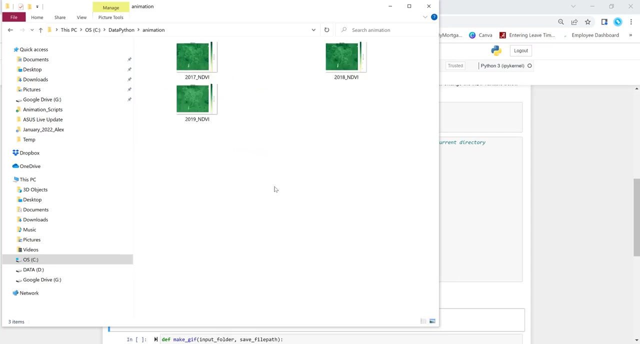 for all the years, right? so that's the first step, and so we haven't yet implemented. actually, let me close this so that we, our space is a little cleaner. So, as it generates all of the plots, it will automatically generate some sort of monitoring of the output, And if you go to the animation folder, you can see some of this image, right, Let me just make it a little larger. 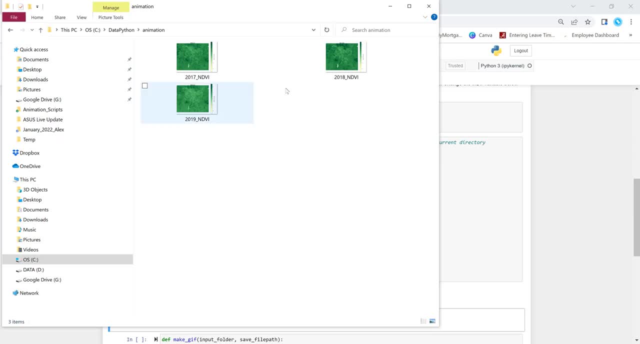 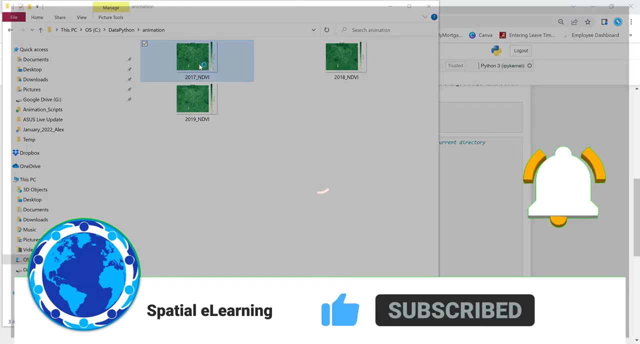 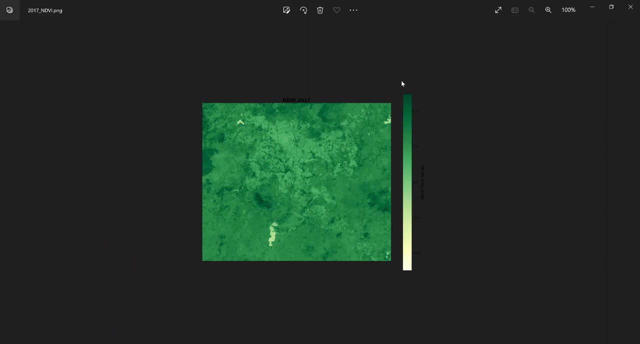 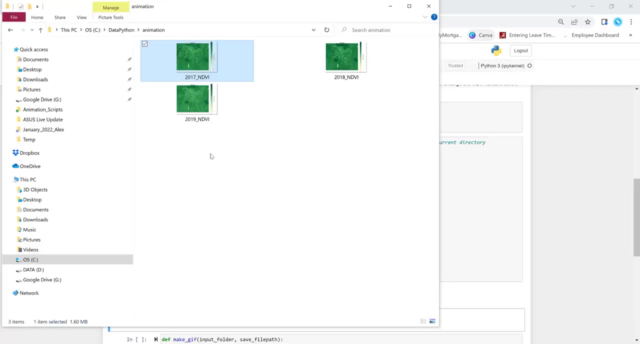 So you can see we have already created this. you know static map layout. If you click here you can see the. you know the image we have created. you know higher NDVI value, lower NDVI value. Of course it's not visible here, just the background. We'll do that on the dashboard, on the Jupyter notebook dashboard. 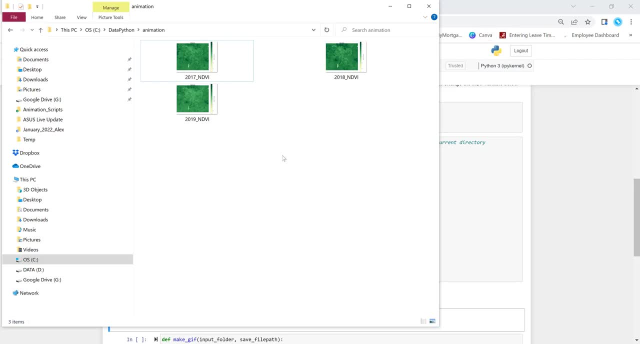 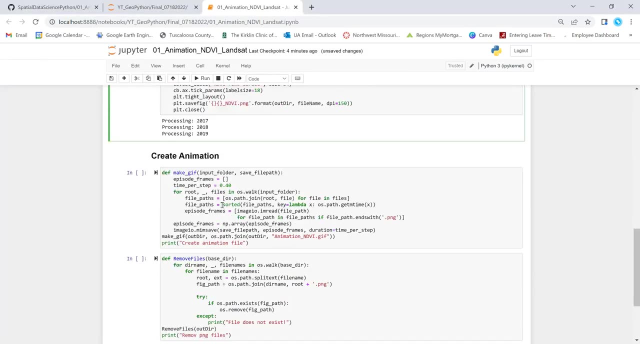 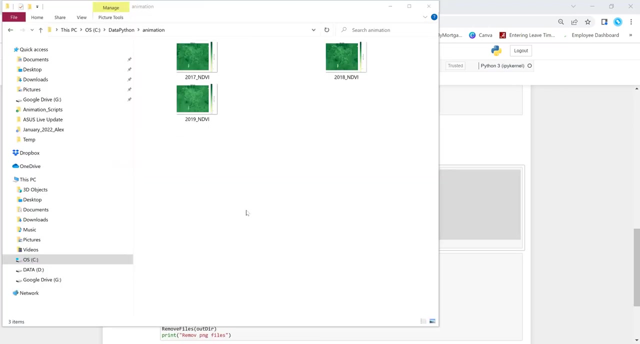 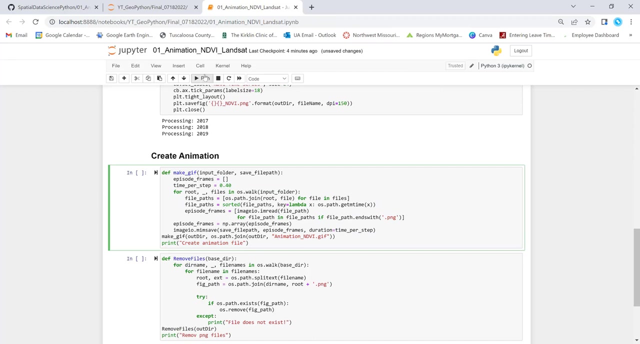 So now what the next step is. the next bit of code pulls all of these static- you know- maps and then just generates a GIF. okay, This is where we generate the GIF. So what this function does is that it will pull all of this you know static image here and sorts them in order and generates a GIF file. okay, So I'll execute that. Once I do that, we'll have a GIF image here. 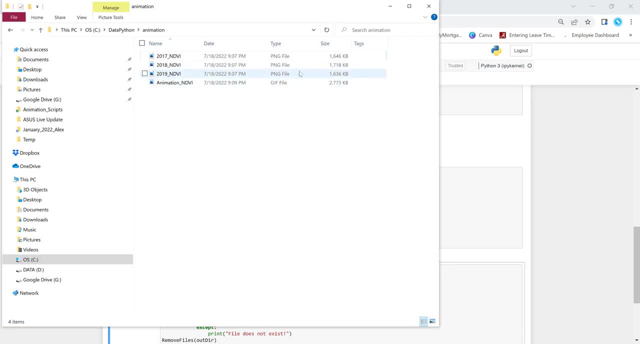 Let me actually list by detail. You can see all of the static maps, are? you know, PNG? Once I execute that code, we have this animation NDVI, right? So let's just click that. You see. you can see. we have already created animation, right? So you have. you know the different years: 2017, eight and 19.. So you know some special variation You can monitor here. I deliberately did like only 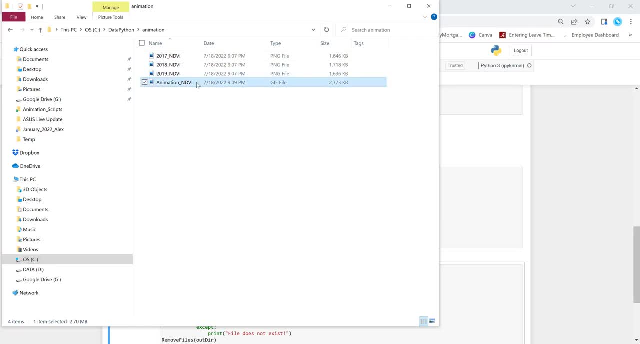 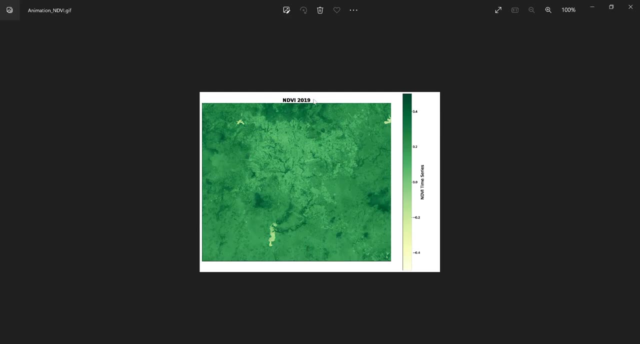 If you can monitor here I deliberately did like only you know few years, but if t easy, p will d your order. so p If you have the data set, you can do it like for 10 years or 15 years of temporal variation over space, right. 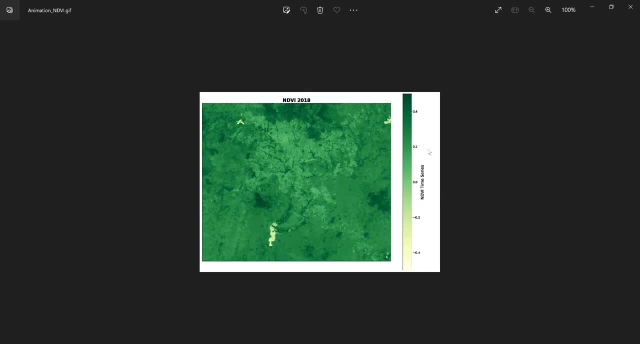 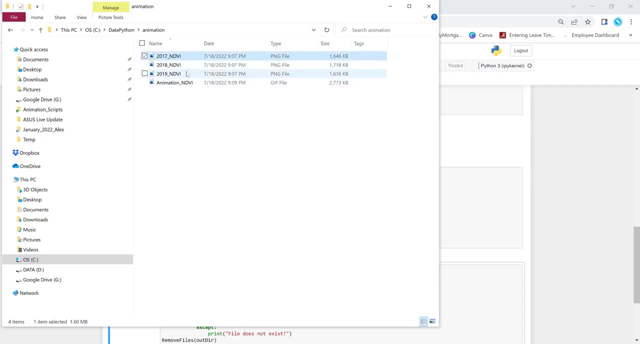 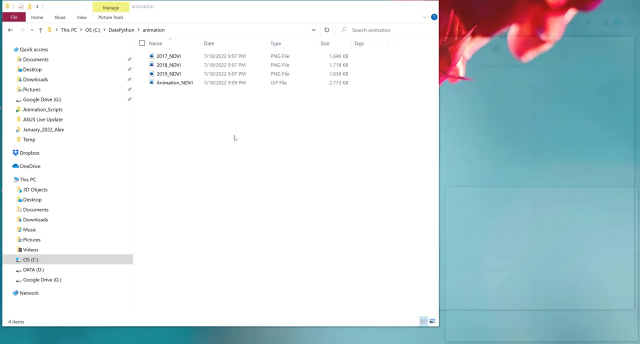 And we have all the legend here, the color bar, So we have already created the GIF animation, Okay, And because we have a lot of static data here, let's just clean that. So the next bit of code is: it will clean all of these files so that we don't just get confused with the animation file. 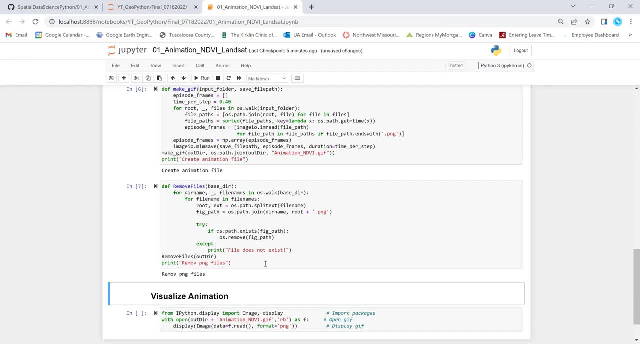 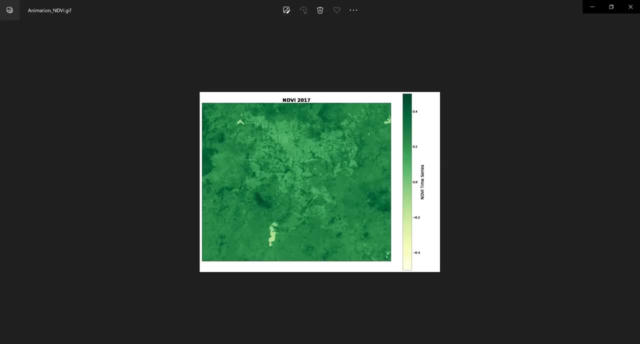 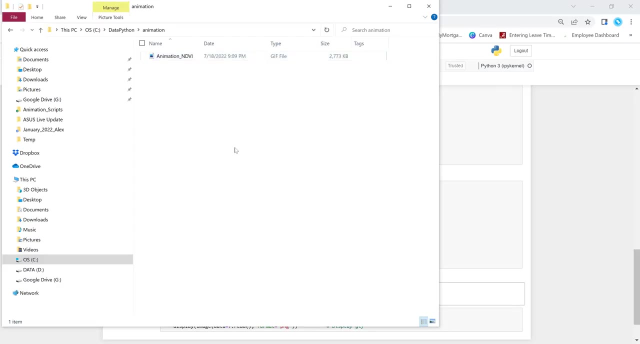 Okay, So I'll execute the remove function so that we have a cleaner folder here. So we don't have anything, We just have only the GIF animation folder here. That's pretty cool, So we can use this in our presentation and, you know, different reporting and things like that. 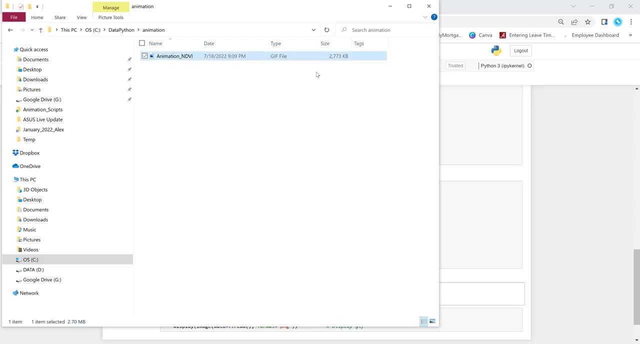 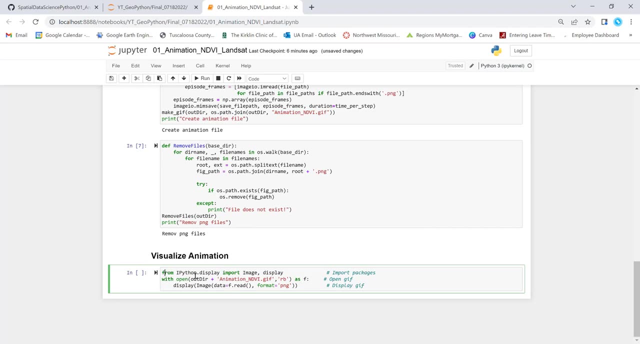 And one of the cool things is that you can also pull this GIF image in a Jupyter notebook and you can visualize that. So, to visualize that we can execute this bit of code, You'll pull that animation, an NDVI animation file, and just place it here. 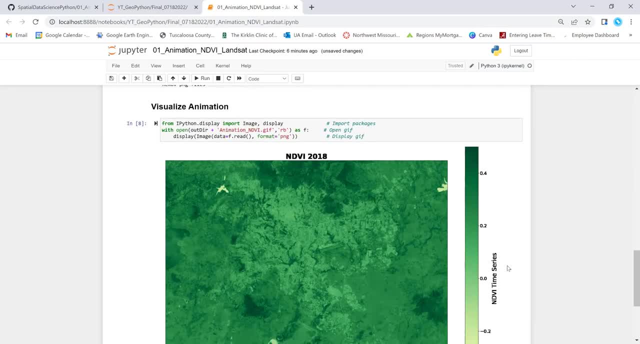 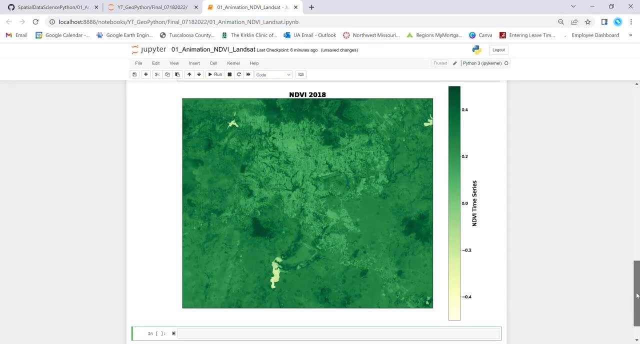 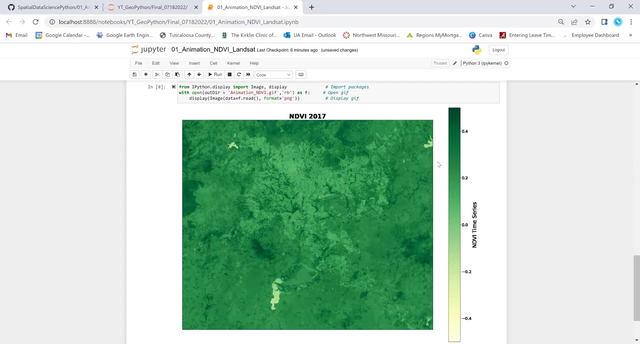 Just let's execute that in a second. You will display that here. So, as you can see here, let's just zoom out a little bit so that you can see the full extent of the animation. So now we have finally generated a pretty cool animation which has all the title and legend. 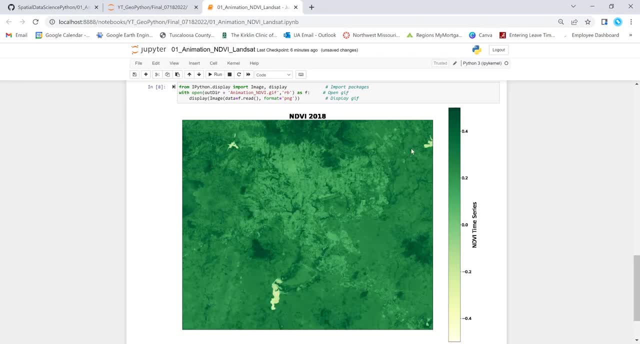 Um, um the color bar, and which is pretty cool, right? You can automatically generate, um you know, animation file using, um uh Python, um you know, script, If you have some sort of image, for example, in this case, NDVI, um you know, from satellite and whatnot. 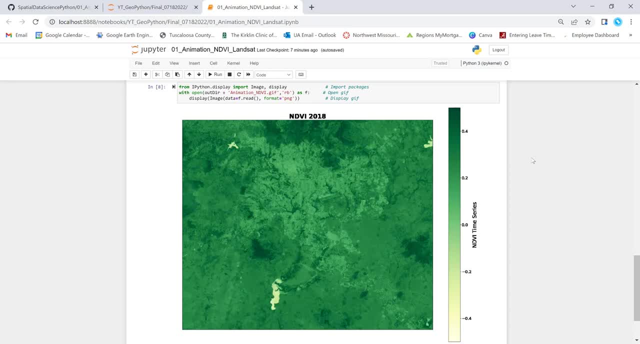 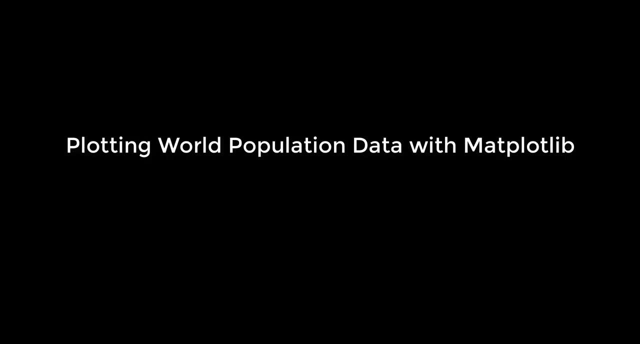 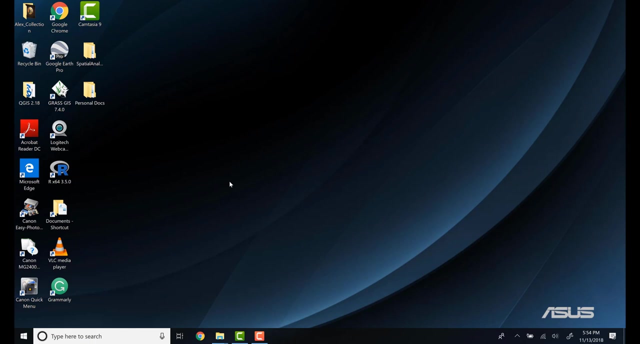 So this is a pretty cool um way to visualize your your data um using- uh, you know um- Python and Jupyter notebook. So in this lecture we'll be um mapping a worlded population using Python, right. 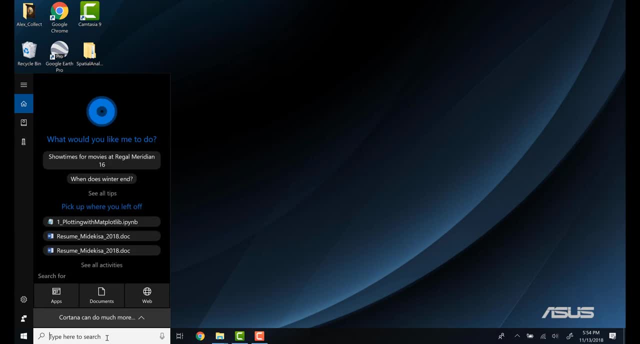 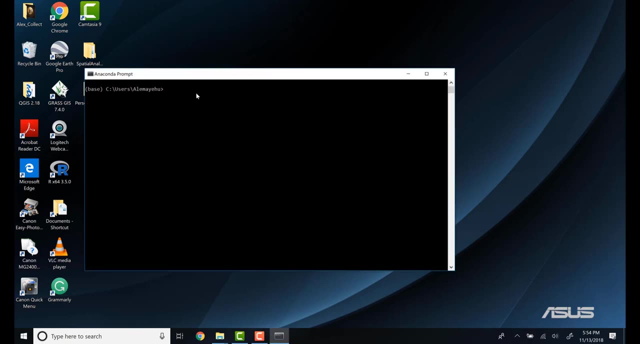 So let's get started. First, let's um open a Jupyter notebook by programmatically using the Anaconda Anaconda prompt. Uh, so, to initiate or to open a new Jupyter window, I'll write just the name of the Jupyter notebook, right? 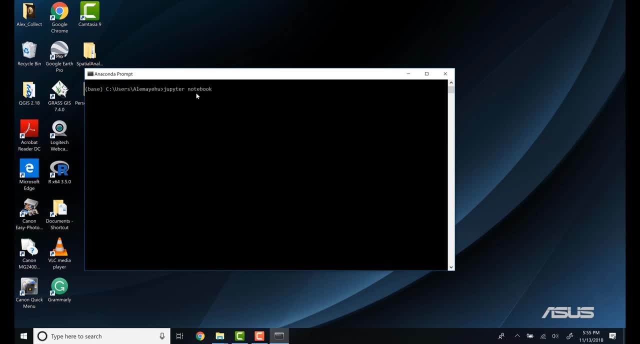 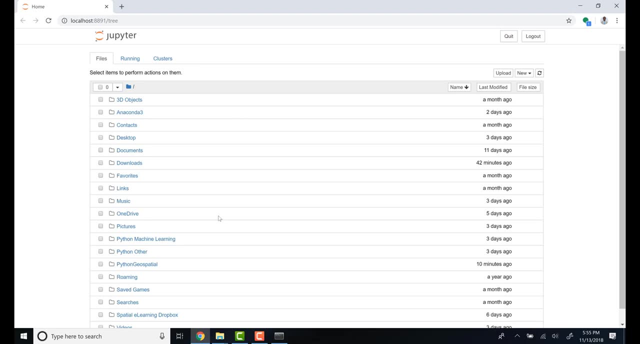 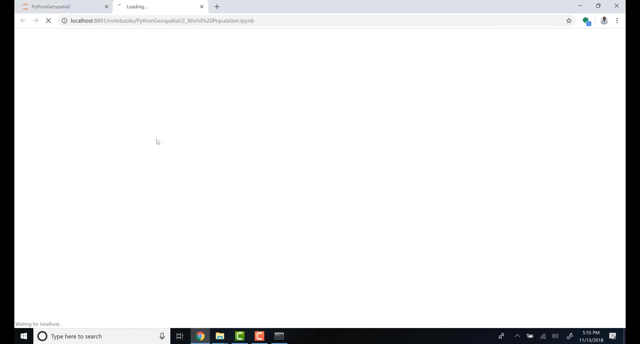 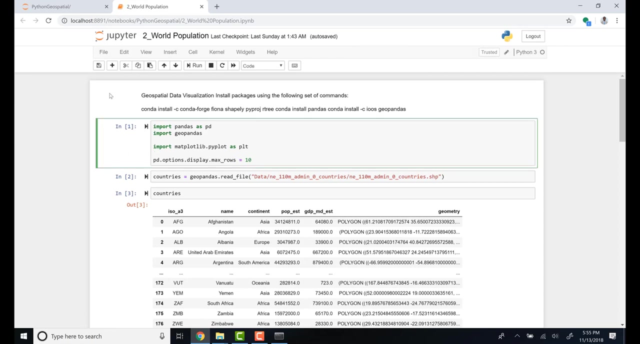 All right, so Jupyter Notebook. if I hit enter, it should automatically pop up a Jupyter Notebook window. right, Okay, excellent. And then here is my you know exercise and code star. and all right, here we go. So the first thing, first is now: you are, you know, familiar with the Jupyter Notebook window. 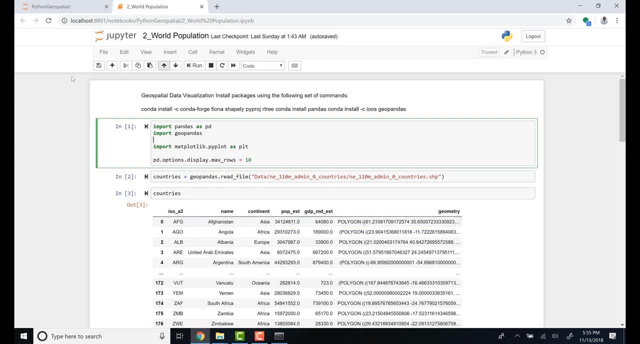 code, you know the cells and all. you know the buttons and some details. So the first thing is: let's import pandas, geopandas- in myplotlib. if you have not done so right Now, in my case it's already installed, but just let me show you how you can install it. 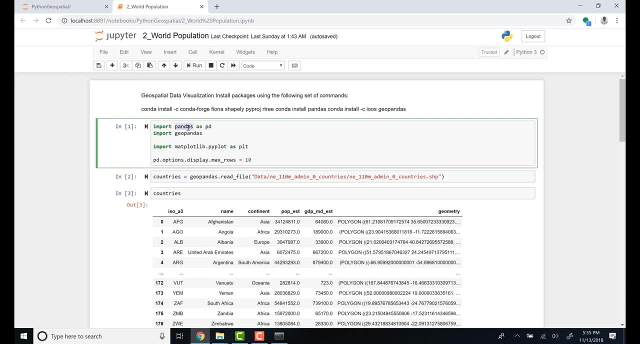 So the you know, the first package is pandas, right, I'll just copy these pandas or just, you know, write it here. So go to the Anaconda prompt. Open a new Anaconda. Open a new Anaconda. Open a new Anaconda. 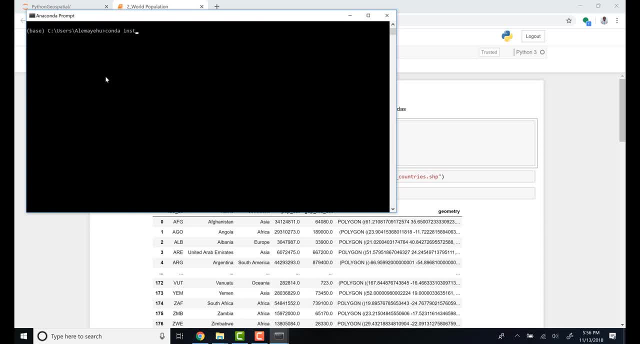 Anaconda prompt. So honda, install pandas. all right, I'll just hit enter. If it's already installed, it would just you know tell me so, and if it's not installed, it will install that package, the pandas package, right. 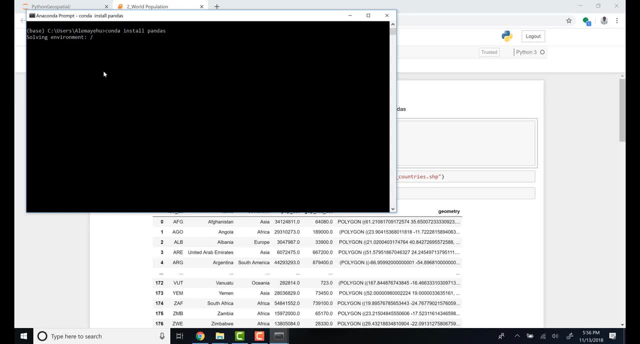 So you have to be a little bit patient. It's processing here and this thing is running, So our required package is already installed, right? So in your case, if it's your first time, then it will just, you know, install it. and if 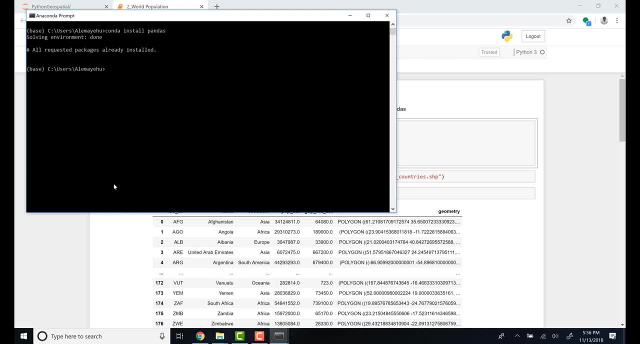 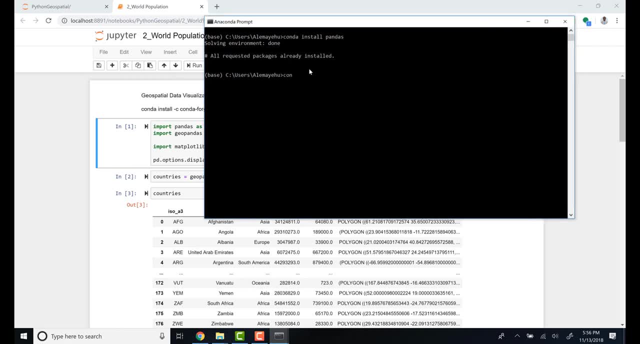 it's processing. it will ask you yes or no. You just type y or yes and then it will just install it for you, right? So what is the other package? geopandas. Let's check that. Conda install geopandas, right. 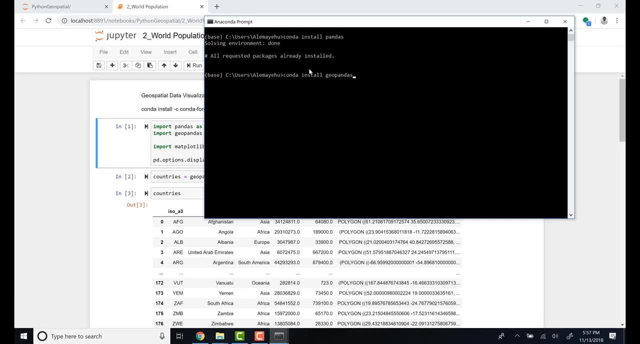 Okay, Okay, So now I'm installing geopandas. Let's check if I already have installed it. It's running checking geopandas package and if it's not installed, it will install it. If it's already installed, it would just let me so. 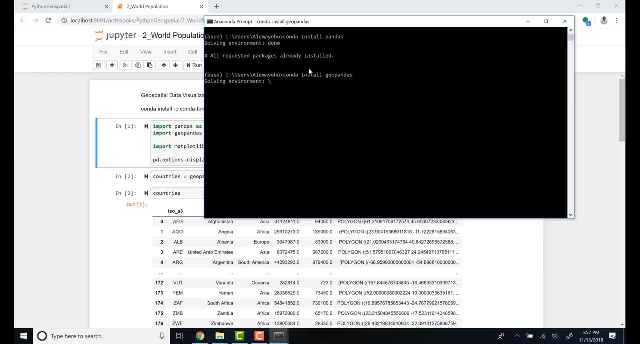 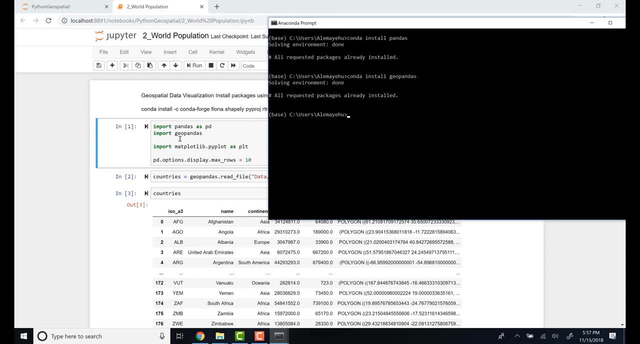 Let me so A little bit patient, all right. So again, so the package is already installed, It's telling me there. So that's how you install. you know here the different you know package that you are, you know, importing. 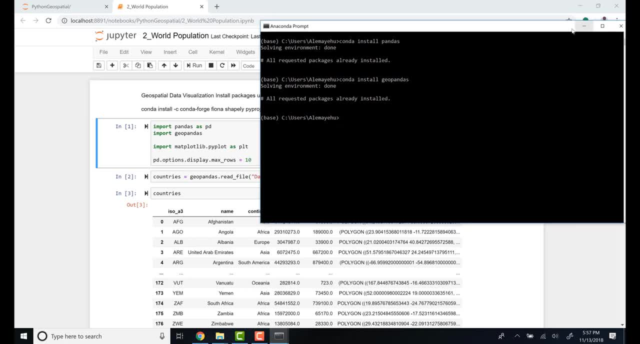 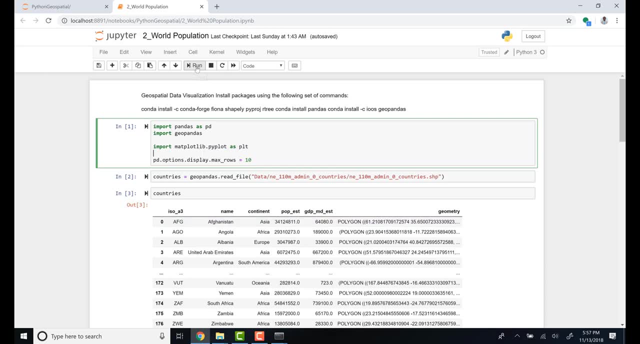 Before you import them, just try to install them here on the Anaconda prompt. So now I can minimize or even close, and now I can just run the cell. Okay, So if it's just going to the next one, it means there is no error, right? 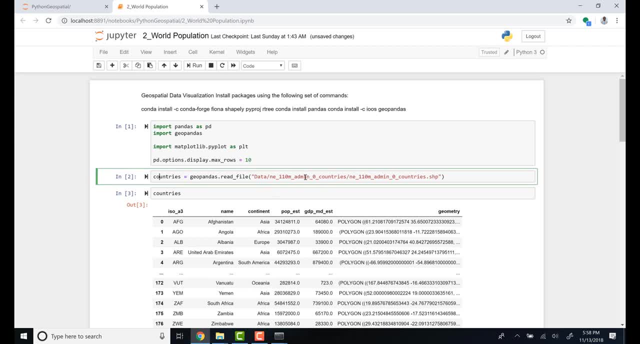 And the next step is just to import you know the country's database. So here I saved it in this you know file. It's a you know from natural earth, It's a shape file for different countries. So if you're, if you're, if you want to put it in the in the right directory again. 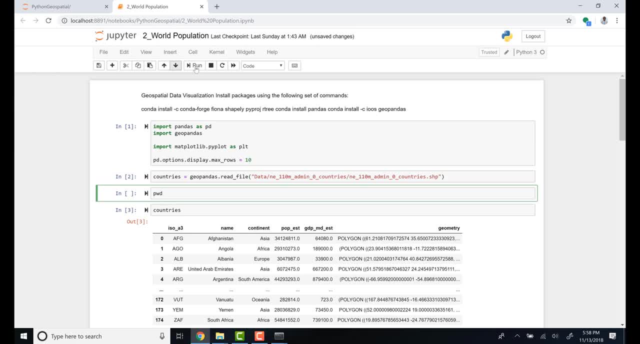 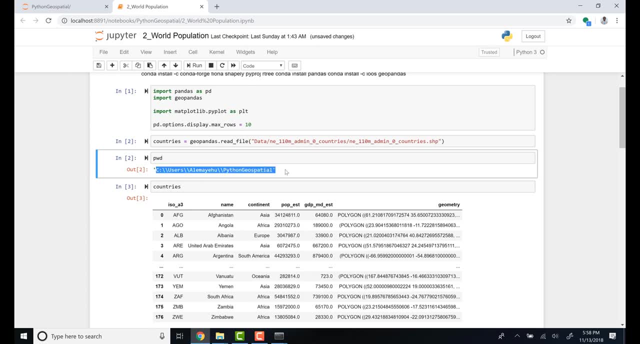 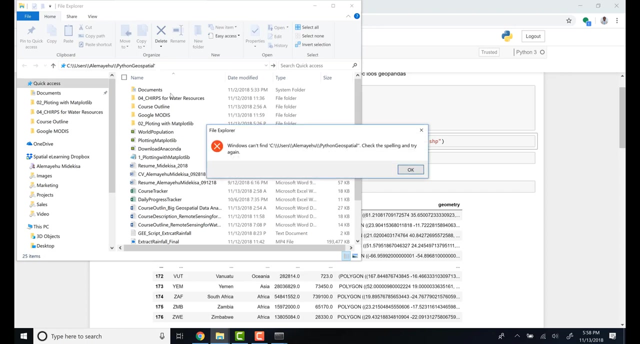 you can pwd. This will tell you your working directory for this exercise though. So this is your working directory And in that directory, just you know, go to that directory and then create a data folder, Right So data, And like just open here, paste that directory. um, oh, that's just a column. 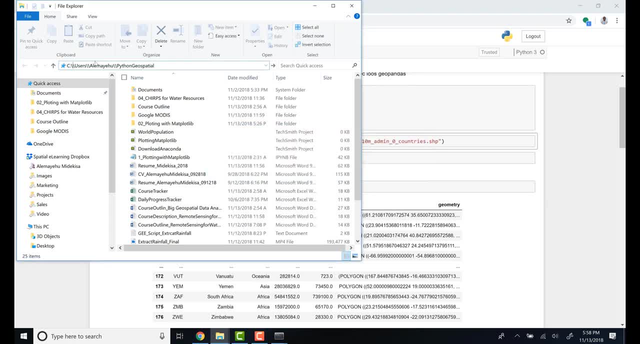 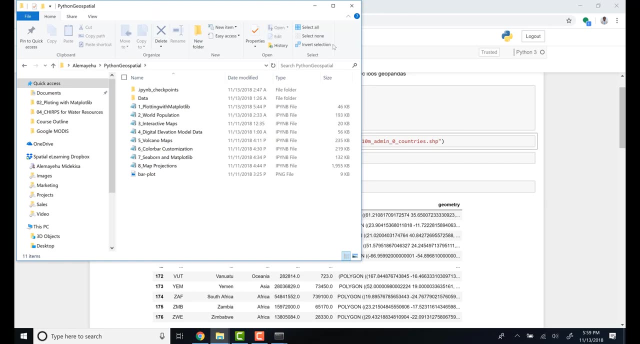 All right. why is it giving me some error? Okay, It's because of the slash. All right, So this is my w you know working directory. I just got it from here, uh, by writing pwd. in your case it may be different. 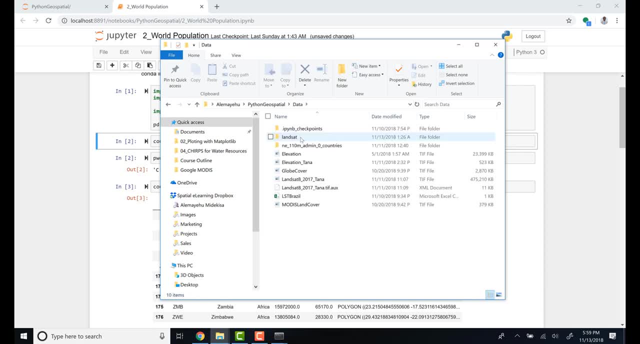 So just go to that directory and create a folder data and then put all of your exercise- you know data here in this folder, All right. So once you put those and so just put all all the files. So this is my file. 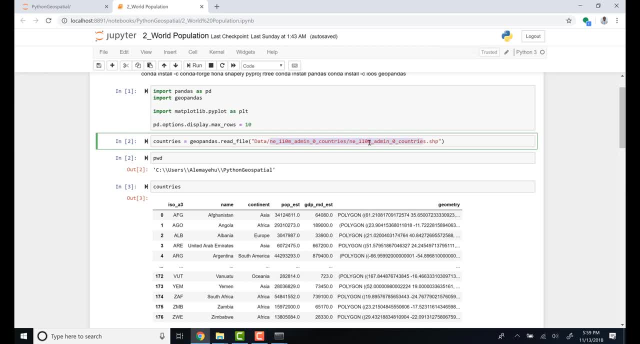 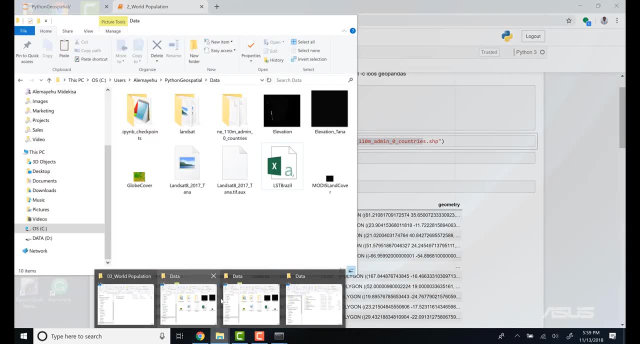 Um, you know the, the shape file, and he uh under 10 meter, admin, um country's database. Okay, Uh, and let's just go to that folder. So this is what, exactly what I'm looking for in this exercise. 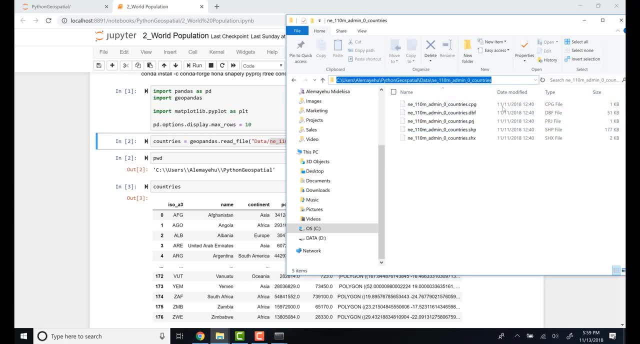 So this is my shape file. Okay, So I'm importing that So you don't write the entire thing, but just to start from data and then you know, you already know you're working, you know directly, So just copy that and then you know, put it here. 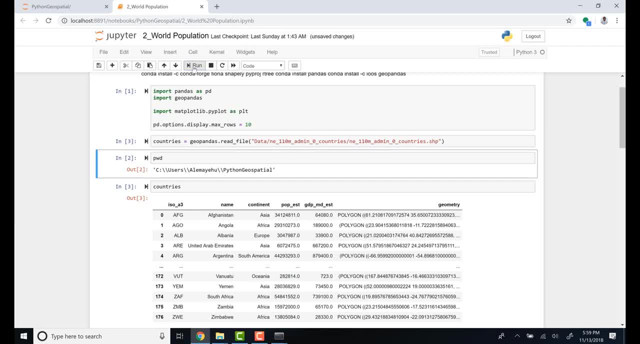 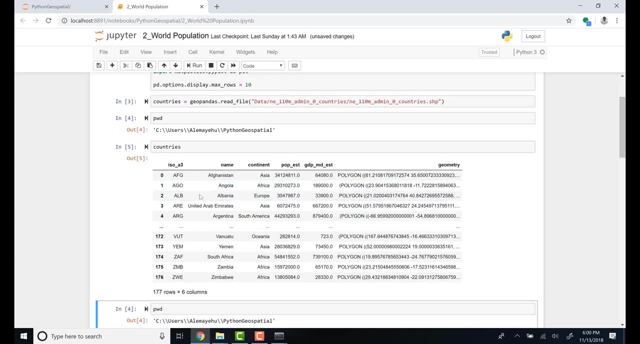 All right, And let's run that. Okay, Countries, If I print that. So what is what is found in this shapefile? countryside? I mean the ISO. this is just a three letter code for each country in the name of a country like Afghanistan, Angola. 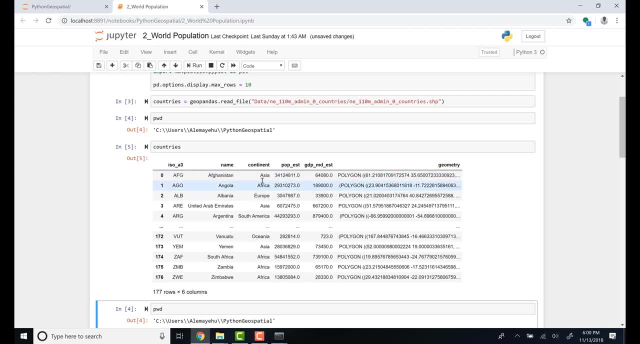 and the continent that um that country is found. And pop estimate is a population estimate which we'll be using uh later in this lecture to map population, um of the word or word population for each country. So now we know that. 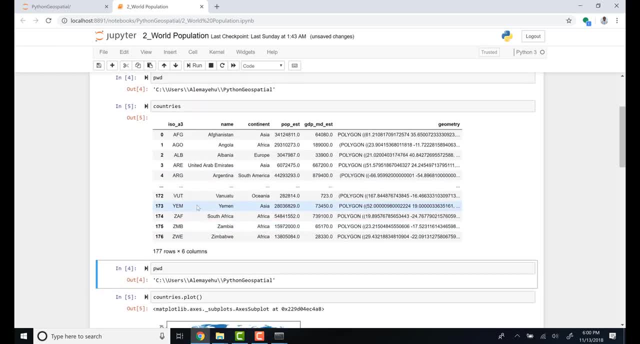 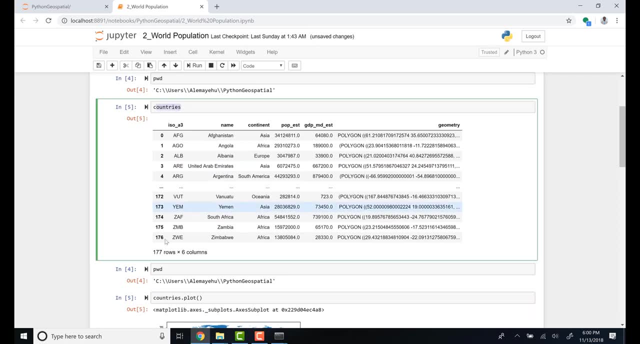 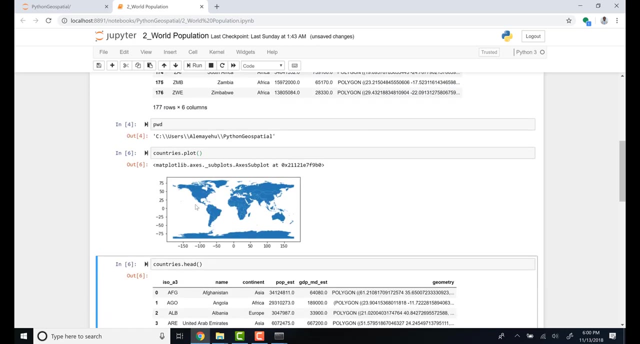 What You know shapefile. uh contains and um. the next step is to plot country. So um the name of. you know the shapefile that we imported and just dot plot. that will give us a pretty cool um, you know just basic um map of. you know the the word. 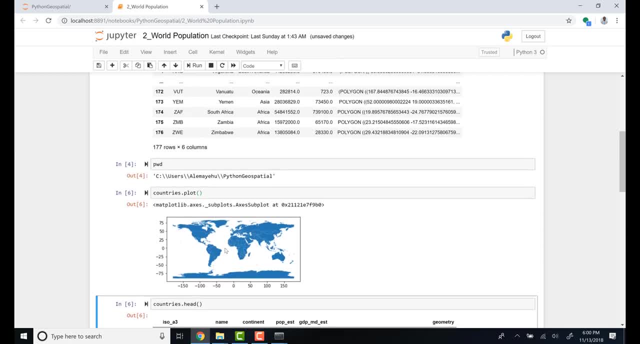 countries. Uh, but, but the but? the thing is that I mean, if you look at this, it's just a single color like blue, and it doesn't provide us any information. It's just, uh, you know, basic plot. 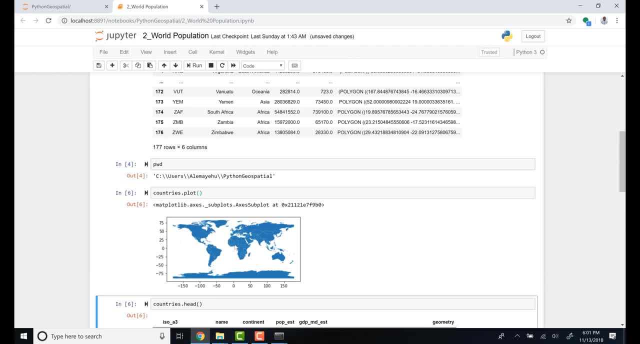 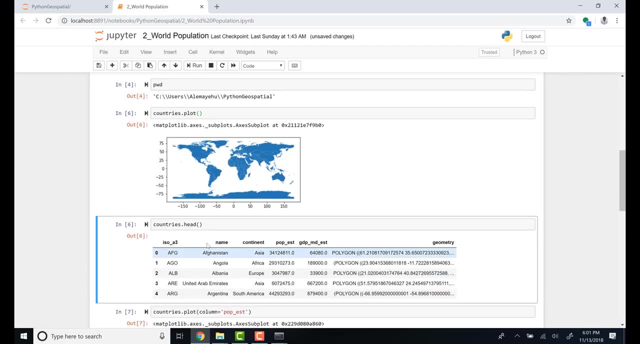 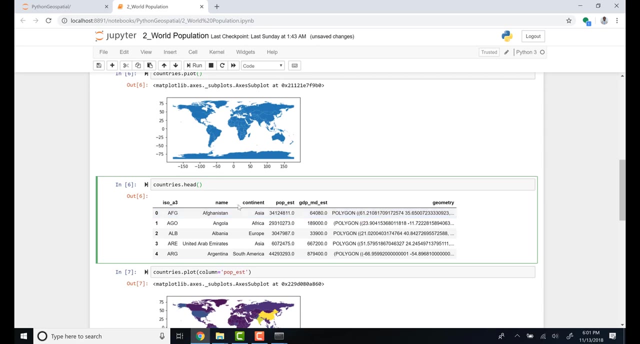 So what we need is just to find a parameter to map, to do the mapping, And in this case we'll be using the worded population estimate. All right, So again you can write. you know, countries head um, which will again tell you, you know. 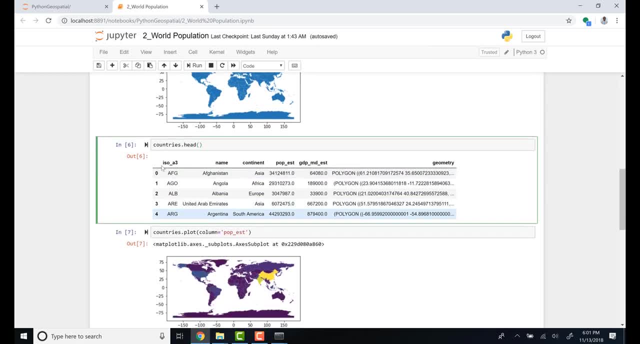 the different columns that you want. So, instead of like a, a default plot, you can define, Um, you know, a parameter that you're interested to plot. in this case, I'll just select pop east. That means pop east, So it will plot based on this, this field or a column. 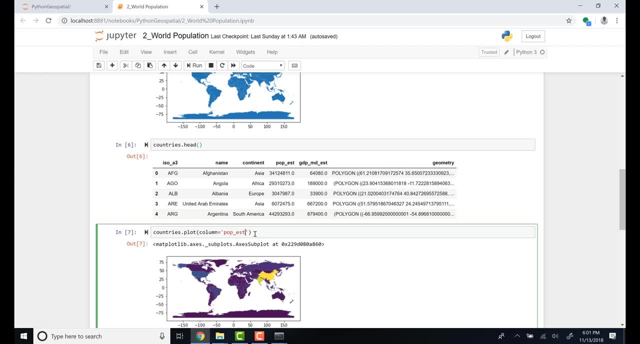 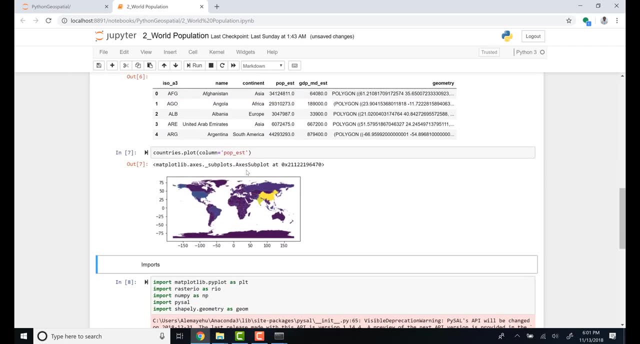 So countries plot and column is equal to this. So it will just give me a plot here If I run that, all right. So it's just giving me um, population of you know the word, that was, you know, random. 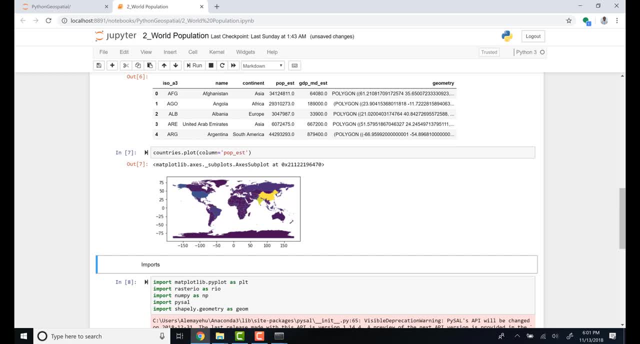 you know colors, like a blue Blue color, But still then it's just. I mean, it's good, in a way, that we're now mapping a population estimate. We know that there's something going on here, the yellow and, um, you know, over here as 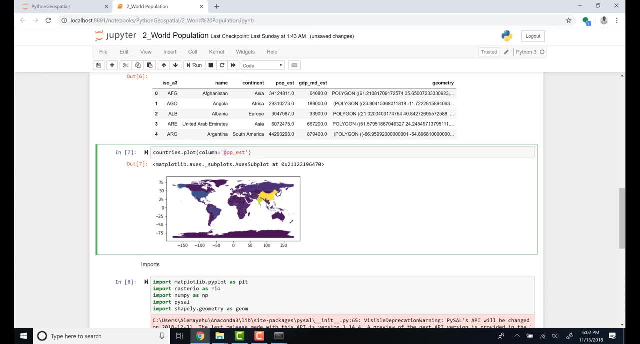 well, but we, we don't know. you know the exact amount or just a proportion of our population estimate, you know, compared to here to here. So we still need more detailed information, Right? So that's what we're going to do in the next step. 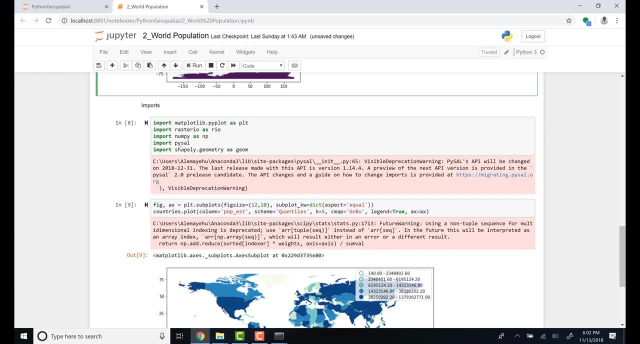 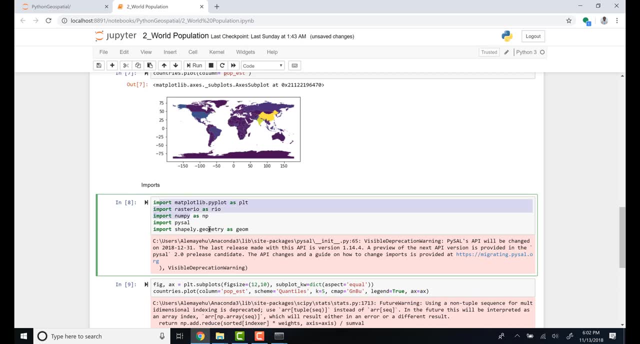 Okay, So, uh, we also. I mean to do that. we need to. you know um import, um uh, uh, install and import. you know these um package. if you have not done so, please do that uh. 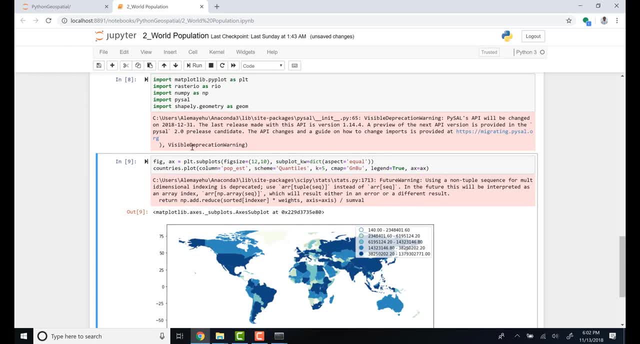 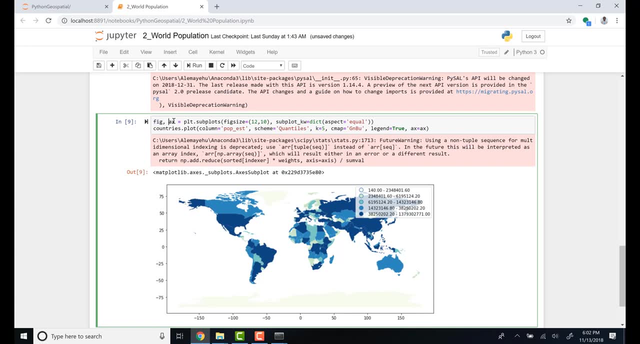 and just run this, um you know, package, Um, I think it should be fine, And then just fig, uh X, um, X is equal to plot subplots. Okay, And now we define some parameters instead of just the default, you know, color choice. 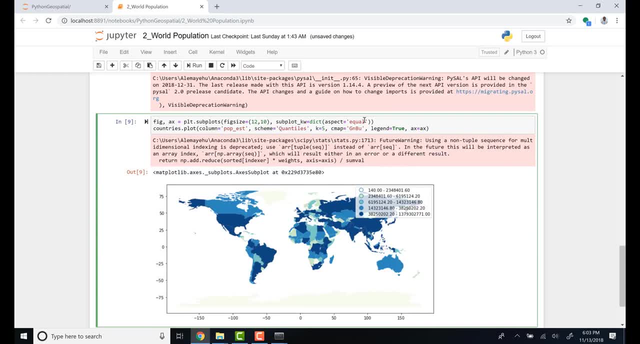 Uh, we, um, you know, we, we prefer like, um, equal interval, like quant, uh, quantiles, quantiles, um, to you know, divide the legend Right, And then we provide the same population estimate data and then we define the color. 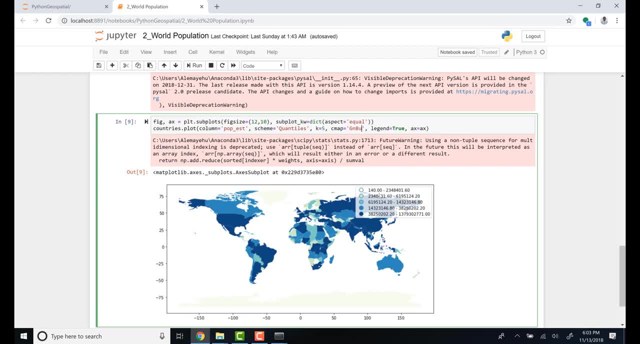 You can change here if you want to, And then, if you do that, it will give you, you know, different colors. The colors came based on the population estimate and provide you the population uh, values. That way it's, it's pretty um straightforward to interpret, right. 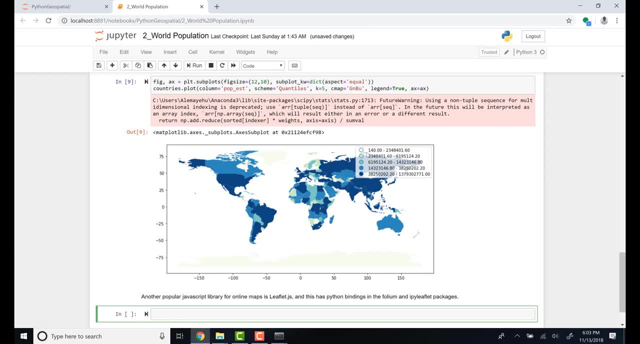 So now we can, you know, we have, for example, here, like the yellow colors are, you know, the lowest population, you know countries, for example, in Namibia and Botswana, uh, fall in this, uh, you know, in this first range. 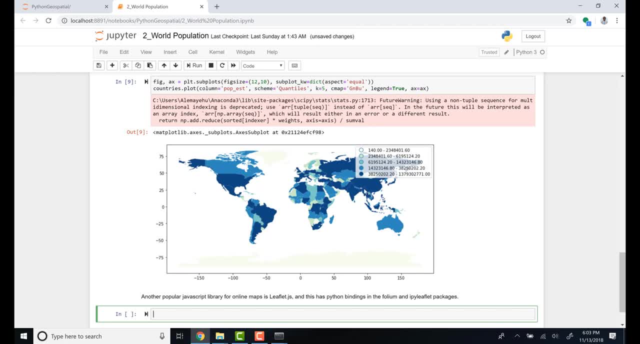 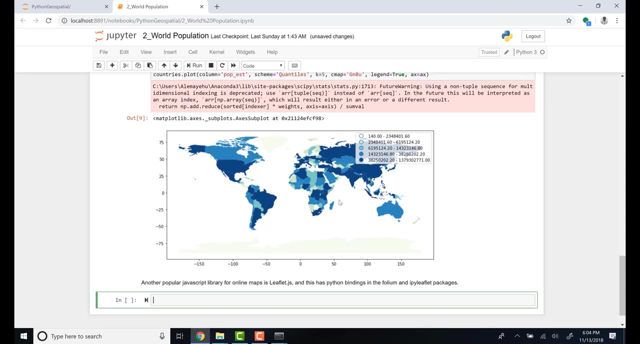 And then the deep blue are like highest populated Areas, like India, China, you know, the United States, Um, so that way, we can, you know, get or extract information visually, uh, by, you know, providing some more details to our mapping. 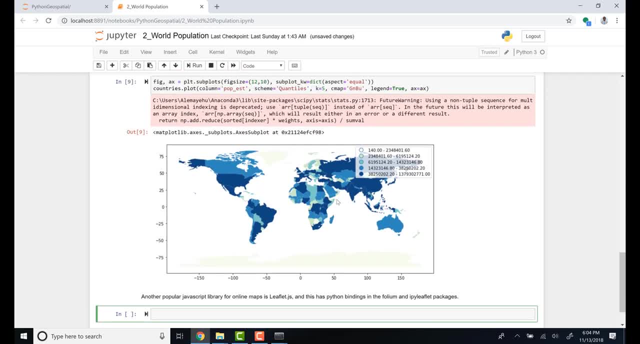 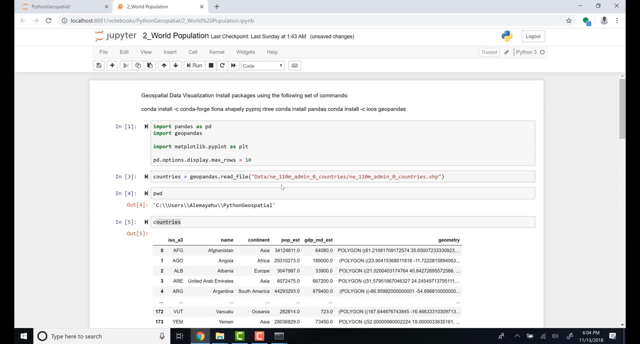 Um that's um how you can, uh you know map, um you know um features uh or shape file uh using uh you know few. package including pandas, GeoPanda SmartBloodLeap. 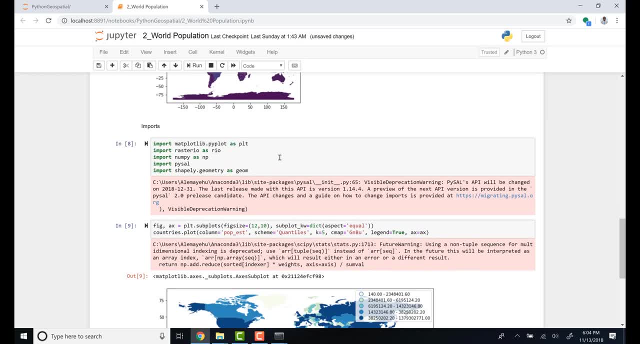 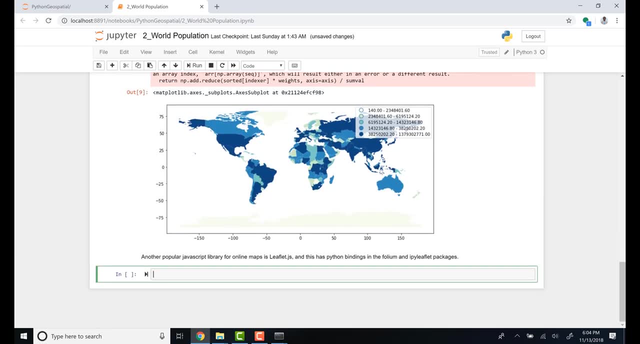 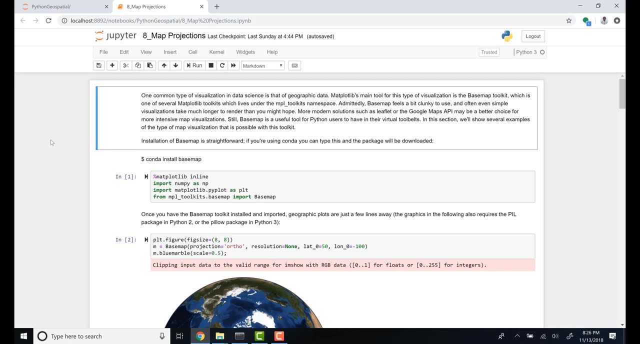 and also uh, some additional uh package such as, um, you know, the Shapley uh and Geometry, Um. so that's um, that's uh. that's it for this lecture. In this lecture, we'll look at how you can uh compare different map projections in Python. 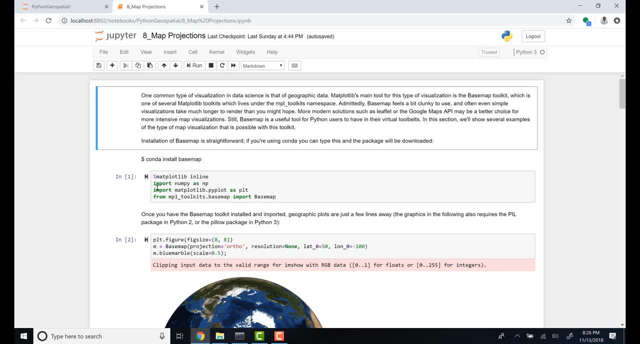 right, Um, so the first thing first is, uh make sure that you uh install uh some package uh, such as NumPy- Uh, I'm at plot leap- and also base map. This is a very important for this, um, you know, for this exercise. 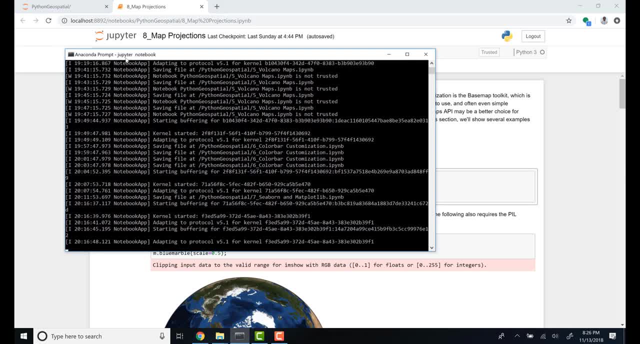 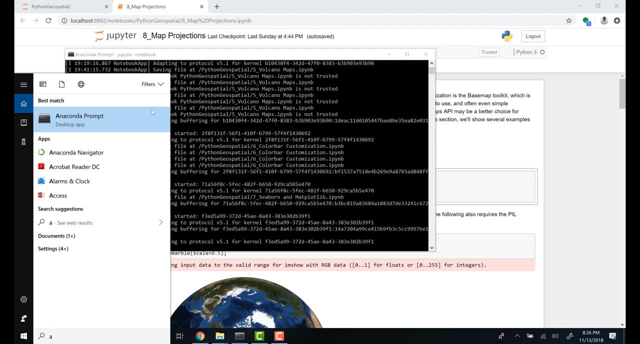 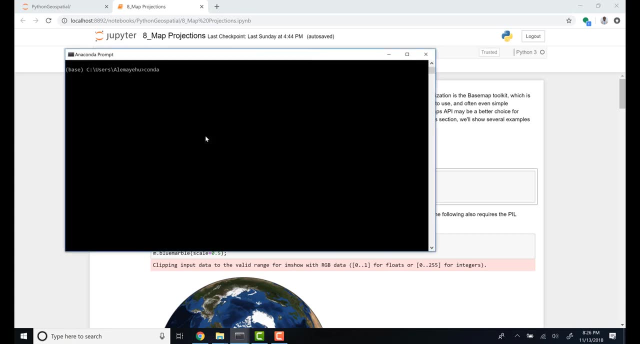 So you just want to make sure that you go to the um Anaconda prompt or just you know able to open here on your console Anaconda prompt and then um write um Anaconda. uh, conda install, um. you know the name of your code. 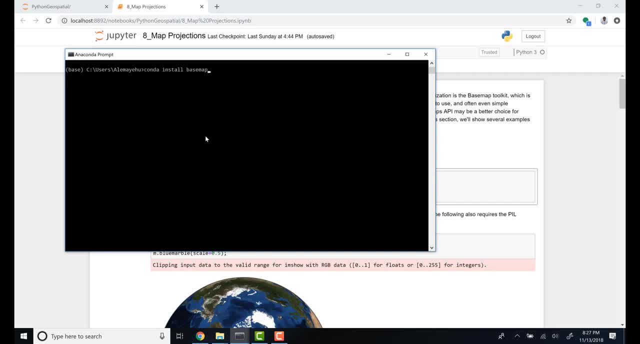 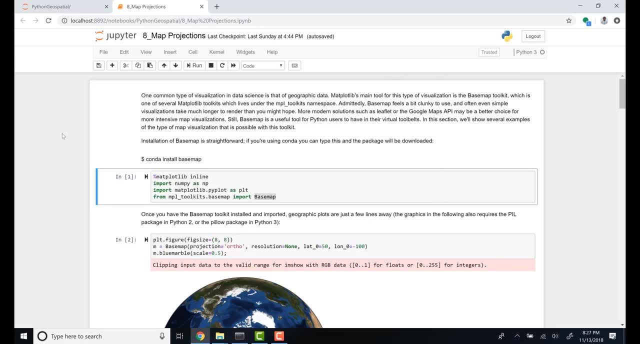 You know the name of your package, for example, base map, right, So you just if you hit enter, that's how you install um. you know your package once you are done with that um and then run the script. 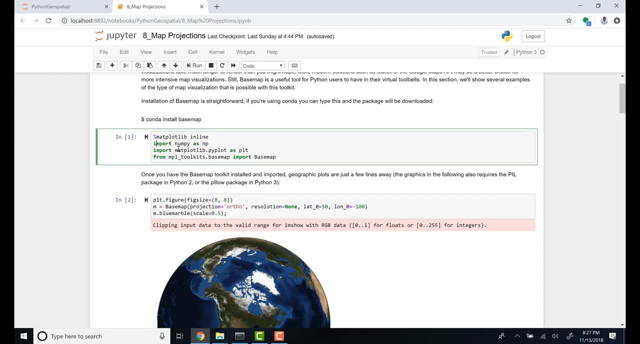 So what we're doing here? just exploring different, um, you know, base map tool to, uh, you know, look at um as a background. you know the, the, the oceans and the continents in different colors, um and in, in different contrasts and also different projection. 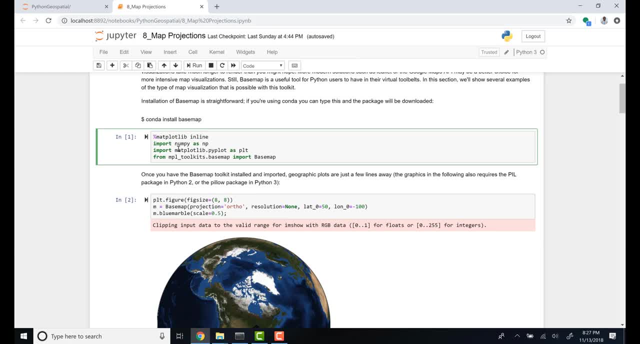 Uh, to create some nice looking professional maps in Python, right, We're using the the map plot leap and base map, right. So the base map will give you a background. um of you know the the map like here: 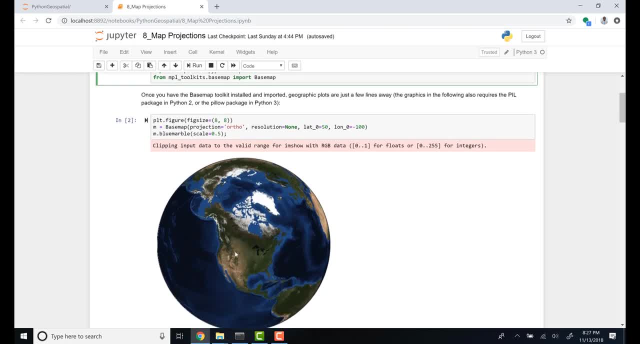 as you can see, for example, you have, you know satellite, you know the satellite background of, you know the earth, uh, the earth's surface and also the oceans, and we'll look at different base map styles. 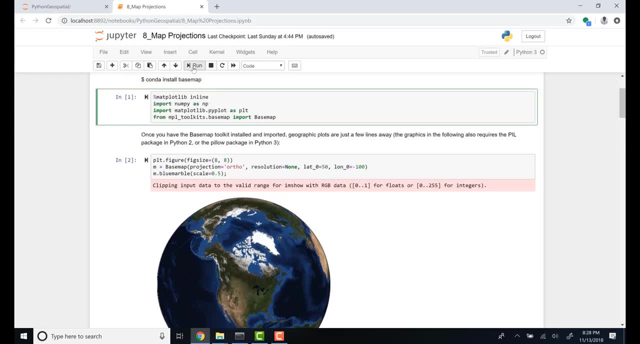 Okay, And also different projections. So let's first run this Let's script. So this is just importing the different package and getting ready, And our first um you know map is that you know we plot dot figure. 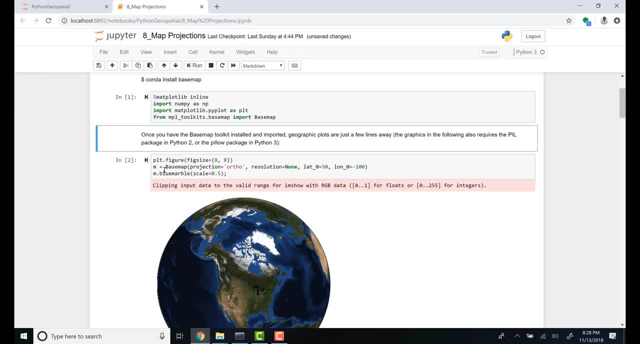 So figure size. we can chain this, you know the, the size of the figure, and then we're importing a base map. um was a projection, Um so auto. so that's kind of the auto view, you know kind of projection. 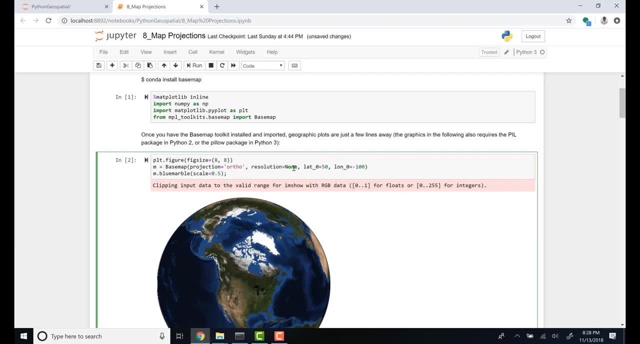 Um, and we can define a resolution, but just, you know, we don't need a resolution here. And then the lot long is kind of the, The, the, the, the focus that we want to. you know, we want to, uh, zoom into our maps. 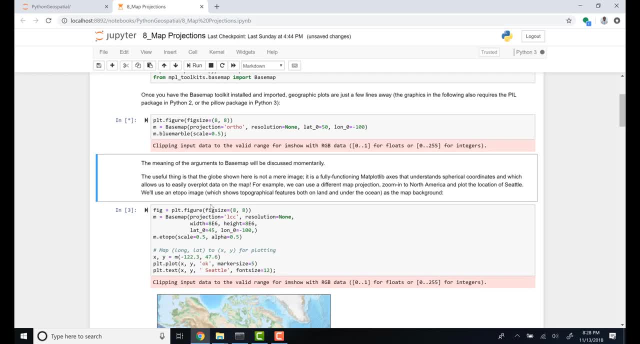 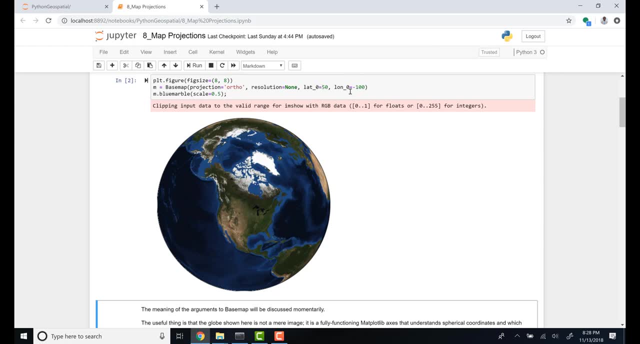 So just if you, you know, click there, um, you know this map, um, you're gonna get you know this, this map. And then if you want to change the lot long information- it kind of changed automatically. 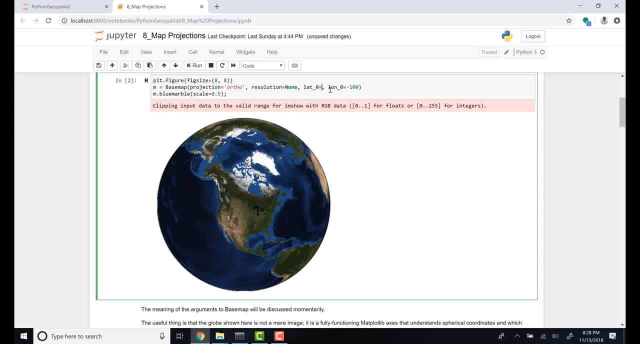 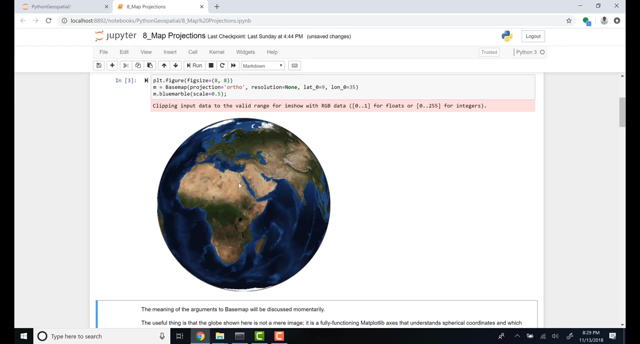 Like, like, for example: um, if I look at here, uh, latitude nine maybe, Okay, Okay, So do, do, do, do, do do. the g to 35 should go somewhere in Africa, All right, 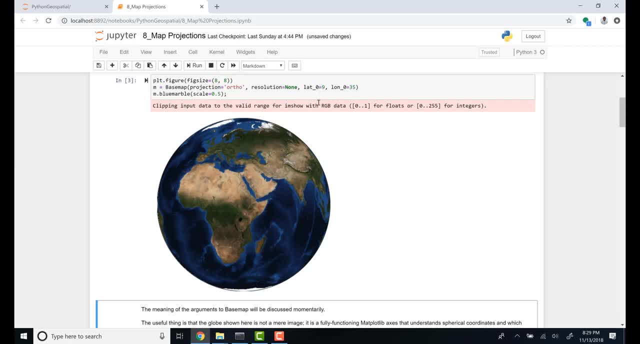 So you can, you can dynamically change the focus of you know this map, right? Uh, if you change it a little bit, um minus you know 10, it will just go, you know, below some, some part below the equator. 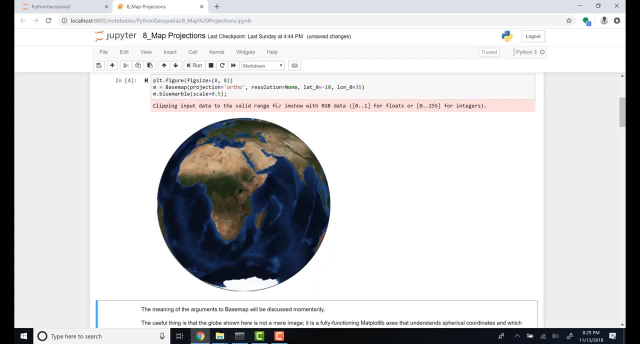 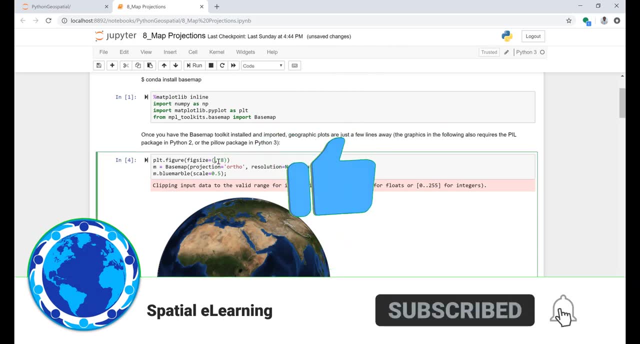 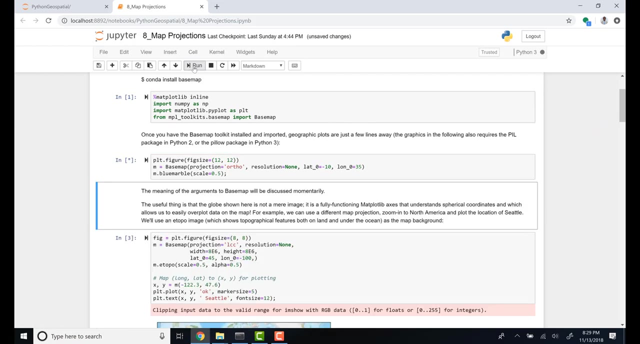 Right, Um, and zoom in into Africa. So, So you can, you know, you can play with this uh lot long information, um, and then the size, um. you know, for example, if I change this 12, um and run that, see, so it's just. 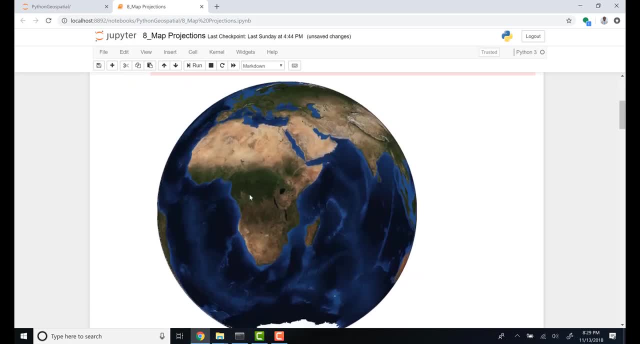 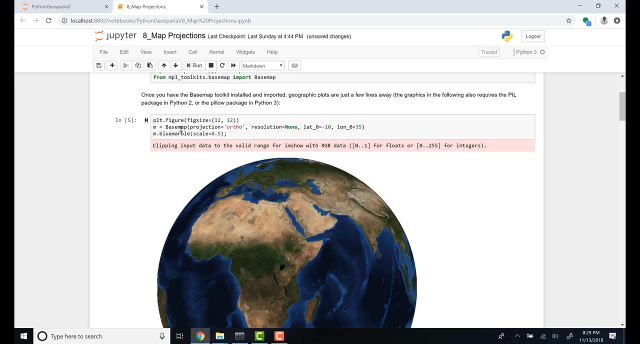 enlarging it. you know, you can increase the size of that map and then you can focus a different map. It's pretty cool. It's. it's amazing That this base map you know package Mm-hmm. 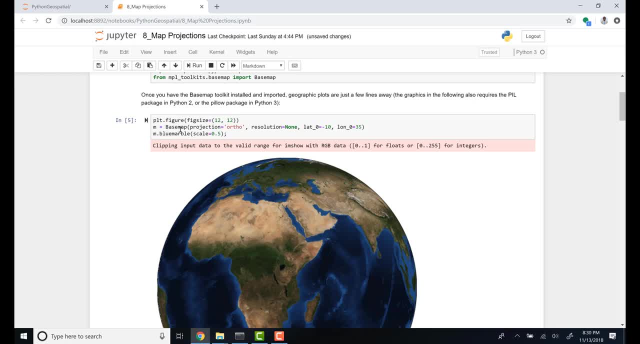 Which will let you create some, um, um, you know, very nice looking. you know professional maps. Right Was a, it was an amazing. uh, you know background. Let's go to um another. uh, you know mapping style. 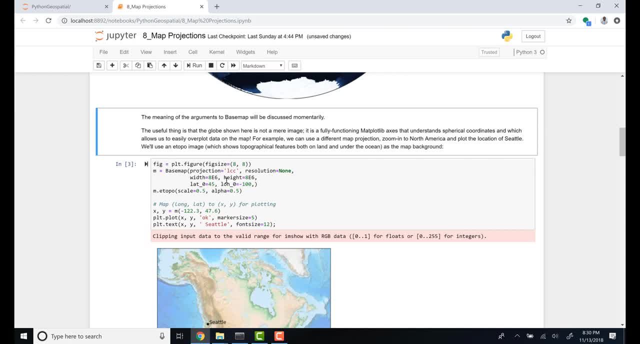 Okay, So here we're just creating: um, it's, you know, LCC, that's the, the, the projection style that we're choosing here. Uh, again, we'll plot. you know the size of the, you know the map. 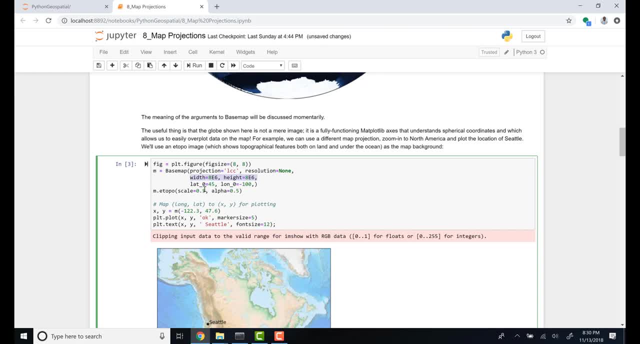 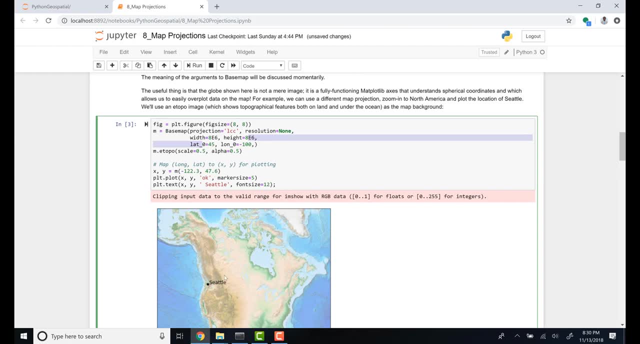 And then we we define the weeds Like you know, the weeds in the height and just also the lot line information. um, here in this example we'll just focus in Seattle. So we're giving a lot line information in Seattle area. 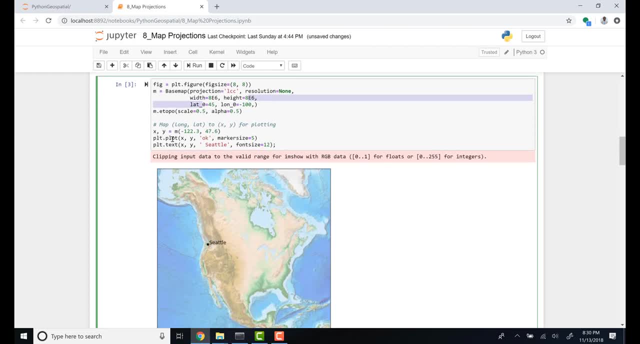 Um and w the. you know, the beauty is just, we can also create some um, you know marker, like, you know this marker here, and then we can write a text if you want to, uh, you know Seattle and then just run. you know the. the plot we can create like focus on. 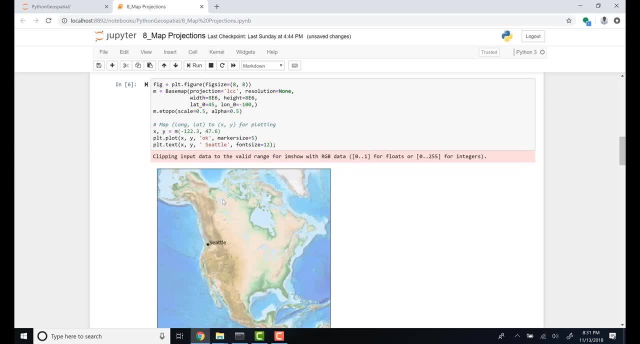 a certain, you know, region of the world, Right, Um and again um, you know, I can change this into um, say, for example, nine, and here longitude information, you know, 32, uh, maybe um, East Africa. I think that's where it is. 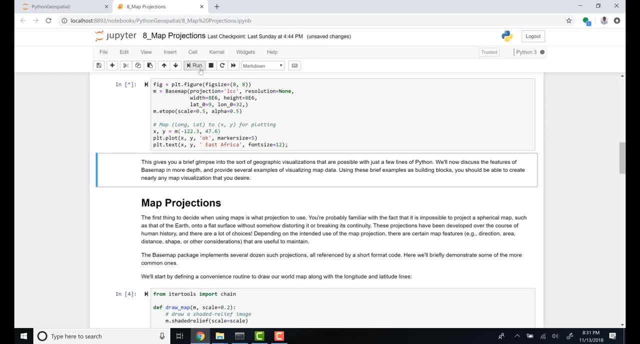 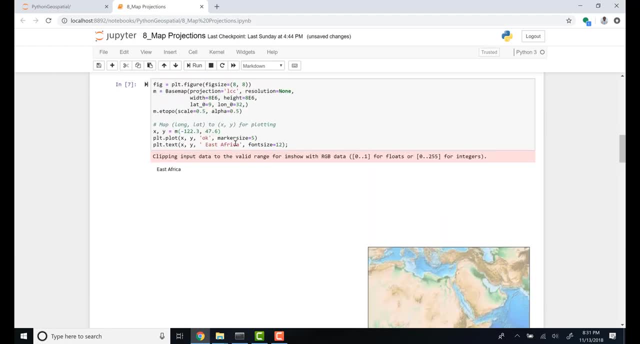 Let's just try and then run. Okay, Okay, Okay, Fantastic. So that's where. okay, We have to define the, the where just, uh, the markers are. it should match the location of the base map. So, um, this is the longitude 32, and and then here is the latitude. 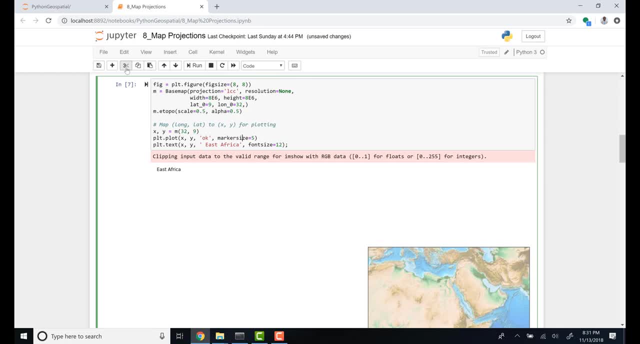 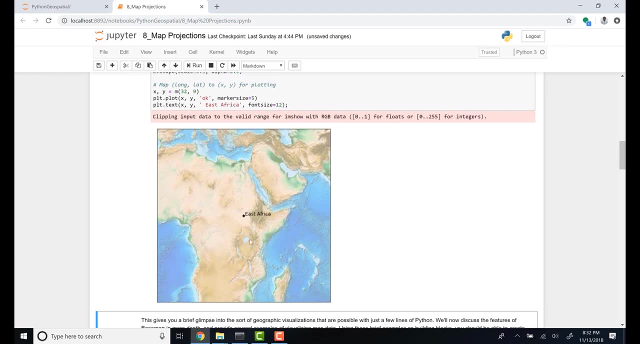 All right, Let's just create, uh, let's run that, Let's run that and see what's coming- Fantastic. So this is. you know, so you can change, you know you can play with, you know this, uh. 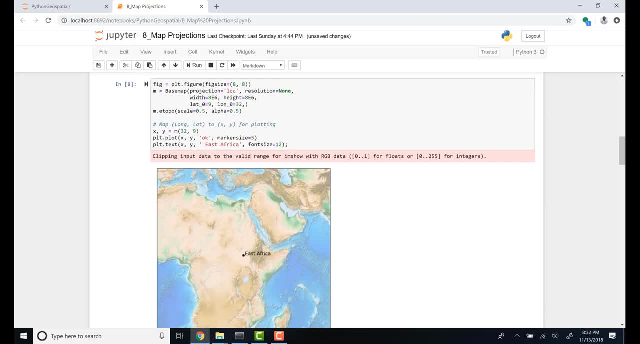 plotting parameters in a in a base map package. That's, that's amazing. Um, so we can change the location, the longitude information, and then zoom into that area and then create some uh markers and also create some text where that area is. 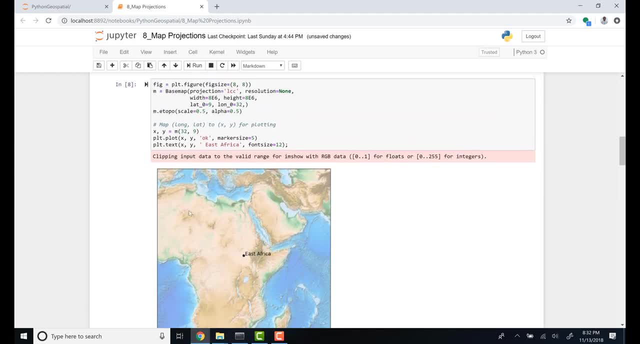 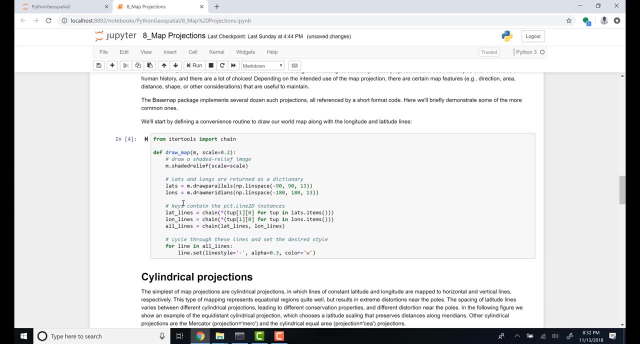 And it's just it's, it's just brilliant, Right, Okay, So um, and then here let's look at um, you know, map projection, So so here, so far we don't have a latitude and longitude, right. 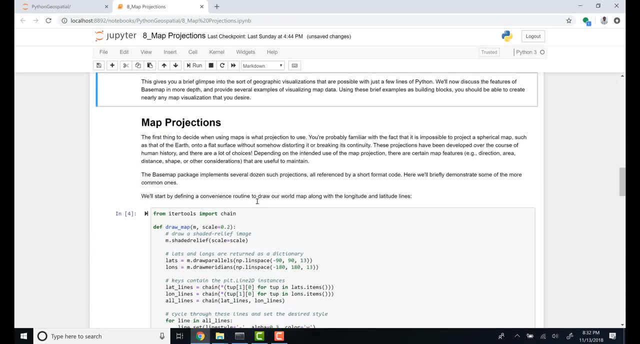 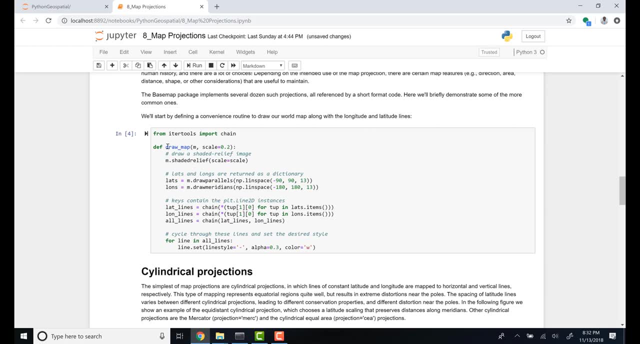 Just you know, this is just a plain map. but now what we're doing here is just write a function to create um the lot long lines, right? So I'll have here um a draw map function, So div draw map. this is my function and um it has just this input parameter, which: 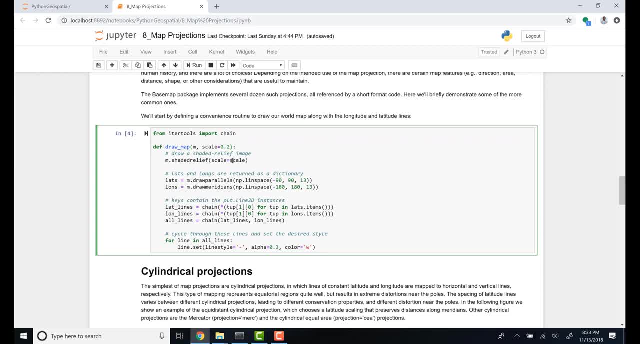 is our map. I'm just going to display it, Just to give it a little bit of space. Right, You know we're going to specify the length, So you can just actually use the pointer to only write your your way to the currently. 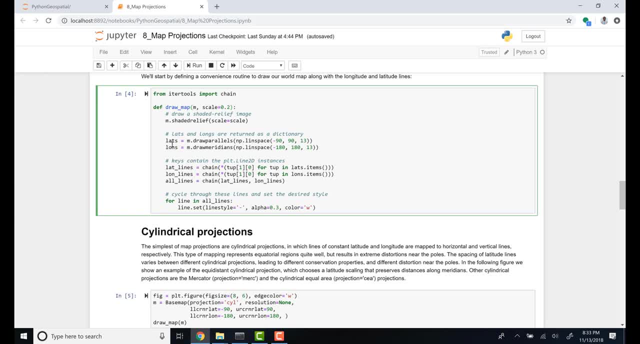 and then draw a shaded relief image Right, And then it would just create, um, uh, a lot long, you know the lot long you know, minus 90,, 90.. Um, every like this is the difference. 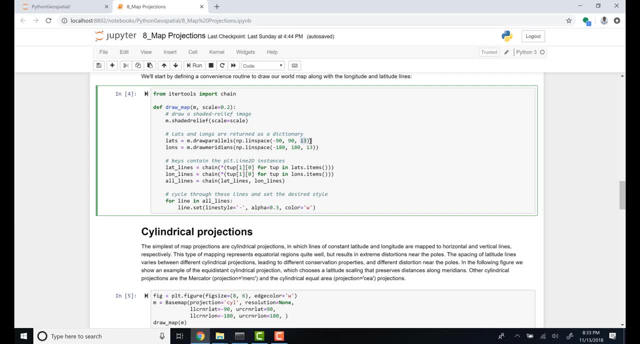 So you know, create a line every 13, um, you know 13,, um, you know units Right, And the longitudes are again the same, just it's, you know, minus at 180,. this is like: 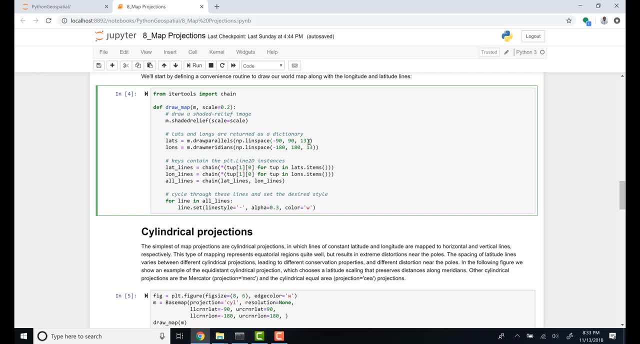 the farthest, uh, um instance, you know of, of, of the, of the, of the longitude that we're trying to go, though you know, minus 180, this is like the farthest you know west, and this is the farthest east. 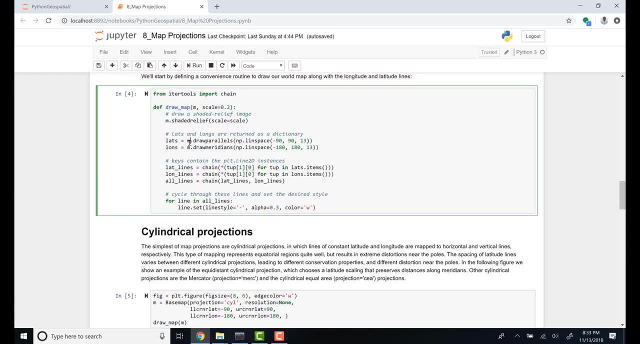 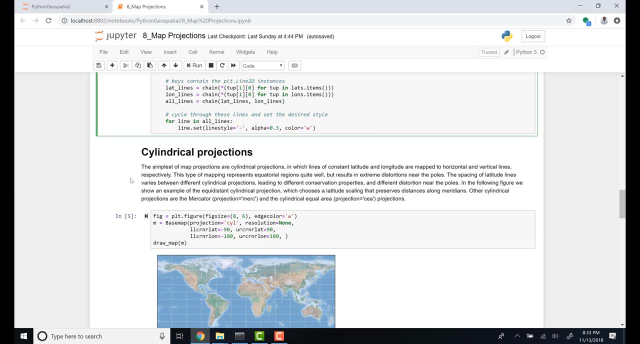 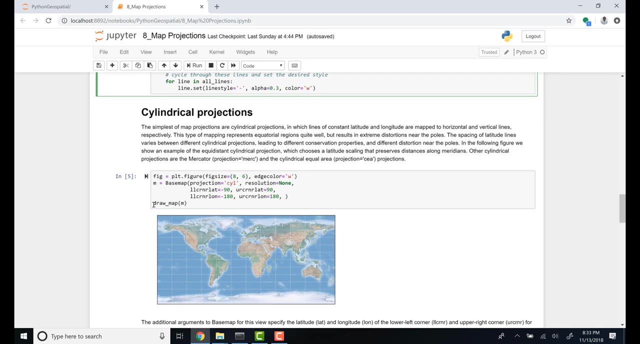 right. And then, once we have this function that creates, you know, a latitude and longitude, let's do you know, create different map projections and then see what comes up right. So the first one is a cylindrical projection and this just creates a typical. 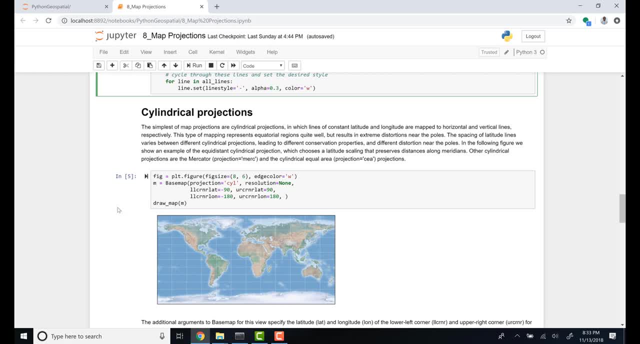 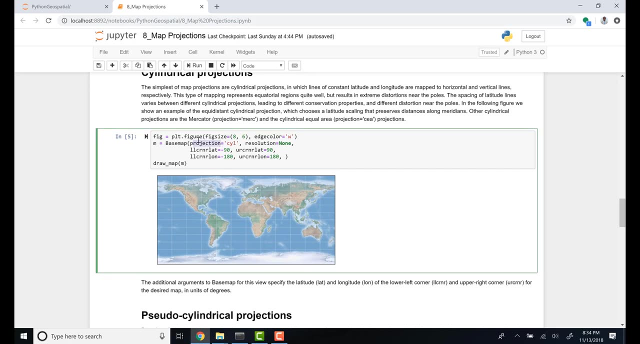 like, you know, the lat-long, the lat-longs are, you know, have a constant, you know gap, like on a straight line, on a horizontal and vertical lines. this is just what you look at. So here, what we're creating is just, you know, defining the projection parameter. 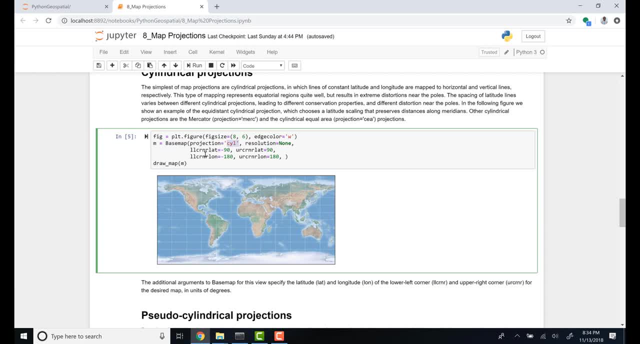 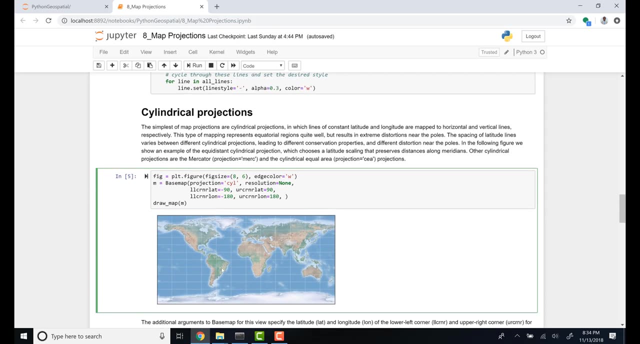 like a cylindrical projection and we're defining the. you know the lat-long, or just you know the latitude range and the longitude range and just draw them up. so draw map is you know function that we created where we can create these lines right? so if we run the 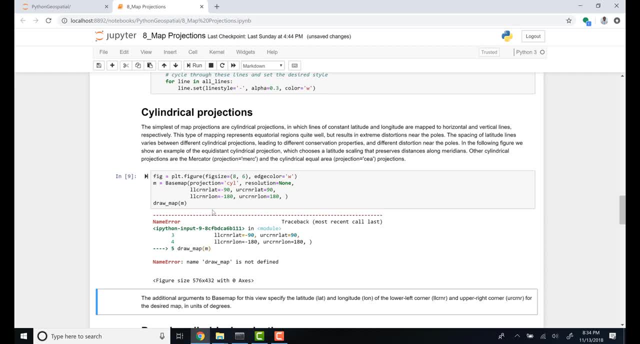 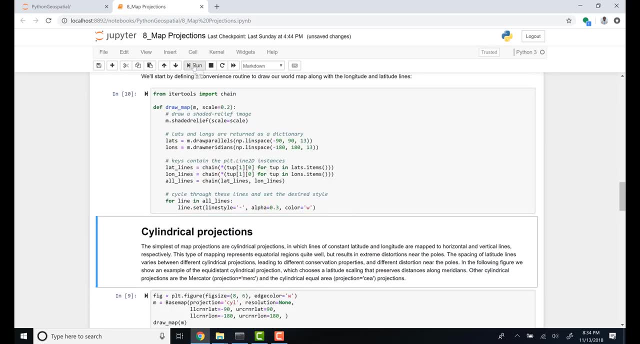 script. for some reason it's just to draw map. okay, we haven't ran this script. that's why, all right, okay, it's because we have not run this, this initial script. that's why it's just giving us here. now it's, it's going good, like I can run it. 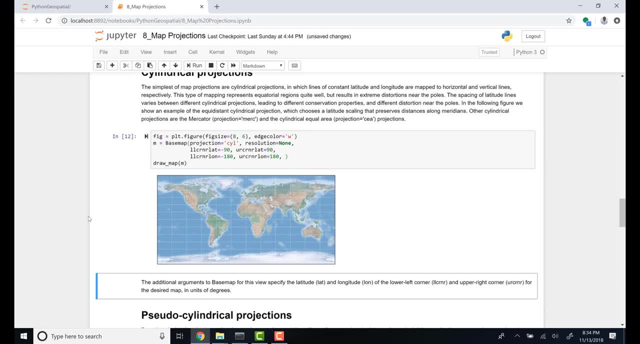 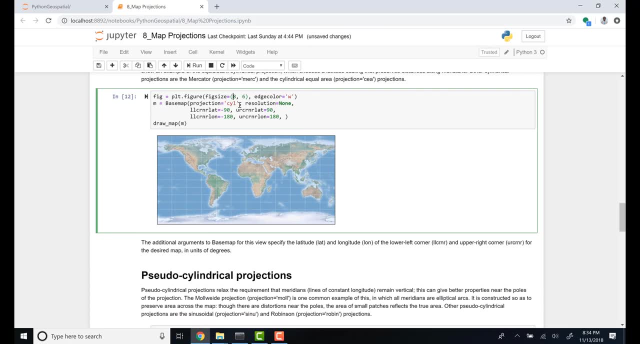 again it should be fine, right, okay, all right, perfect, fantastic. so this is just weak. I think we can change the size of it, probably 8, 6, just proportional, probably 12, 8 plus 4, 10. maybe let's just run it, you know, in large, you know. 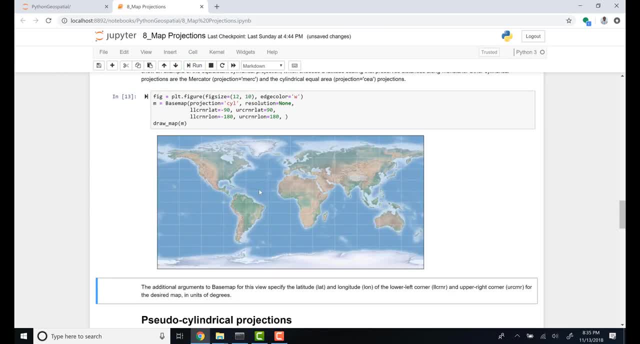 increase the size a little bit so that we can see. yeah, that's pretty cool. so you know, this is amazing. we just have, you know, satellite background and also we have this lot. you know longitudes was a constant, you know gap and also the latitude, like here, and 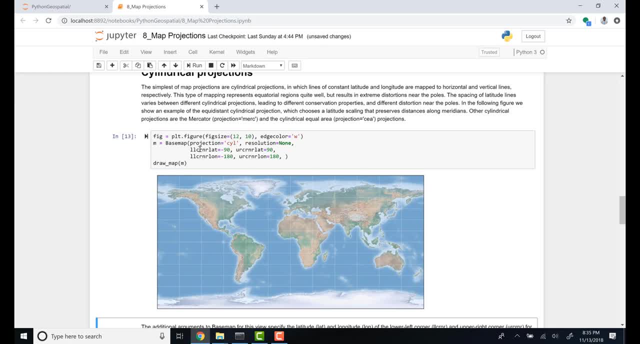 we have that you know draw, map function and also we selected a you know cylinder, cylindrical function and we can, we can define the size like by, for example, I can say the latitude, just to be like, you know, 10 latitude that you know the farthest now I think that's the, the, the South, and this is just Norse and also. 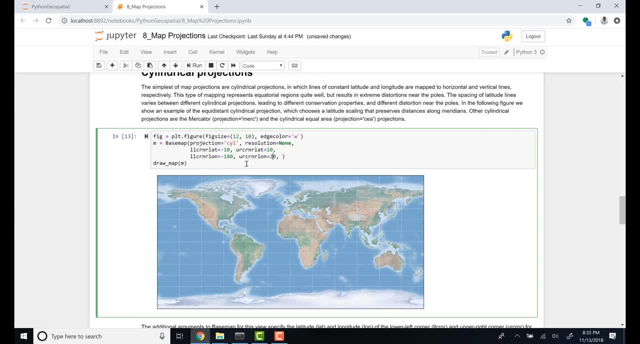 the, the longitude, probably 20 and minus 20. how about that? all right, and we'll have a different, a little bit different, you know, zoom label. okay, you see, I was just falling somewhere- that we don't need that late. let's just change this, probably in a minus 5, and we're going to call the length of our million here for. 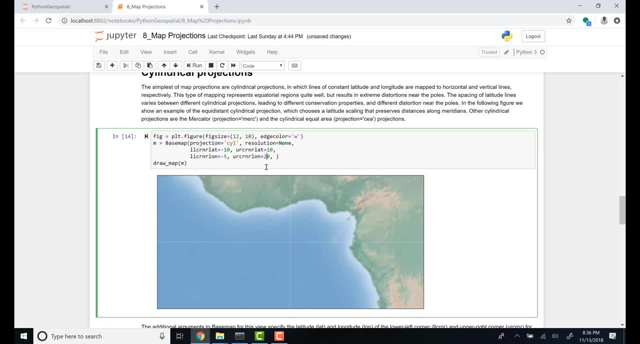 that lake and we're just changing the length of our million here for that lake. five and um, that's the longitude. so, uh, how about 35? you know? and okay, let's just run that. all right, it didn't like it, let's just do about um. 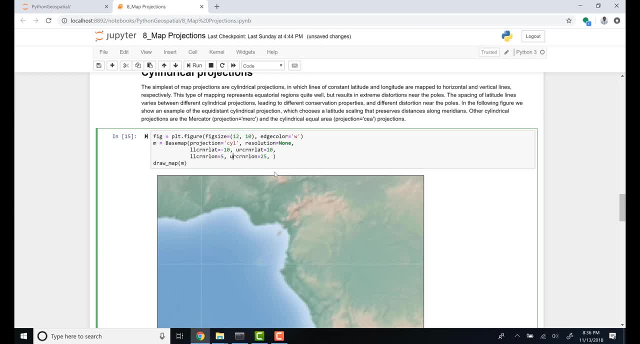 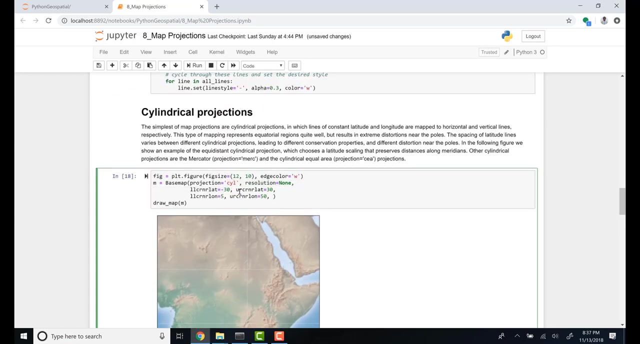 um five and 35.. let's do that just small, some part of like central africa, okay, and let's have something like this. let's have something like this and 30 over here, right, okay, hopefully this our last try just to zoom into, you know, africa. okay, let's just increase a little bit um. 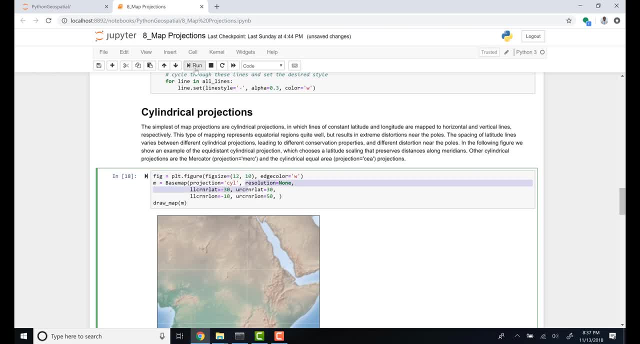 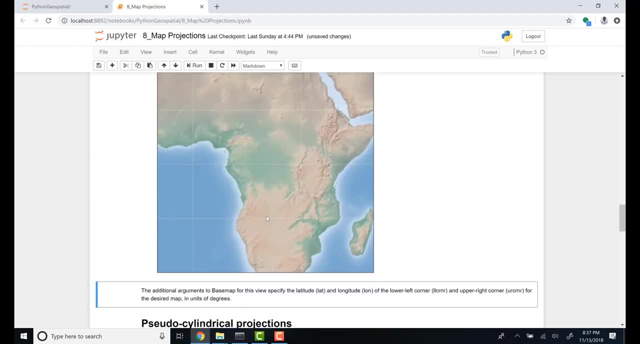 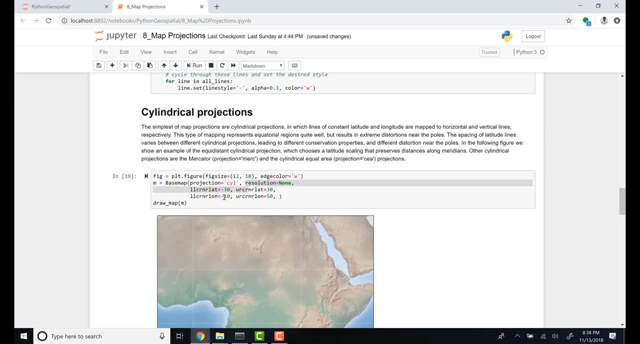 minus 10.. all right, we're just, you know, experimenting to. you know the the lot long. you know um gap, so this is like mostly africa, if not. all right, so we can, we can define the different. you know lot long. you know border lines and just um zoom into any place.